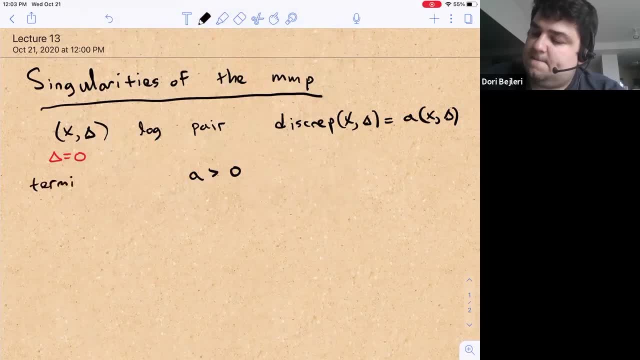 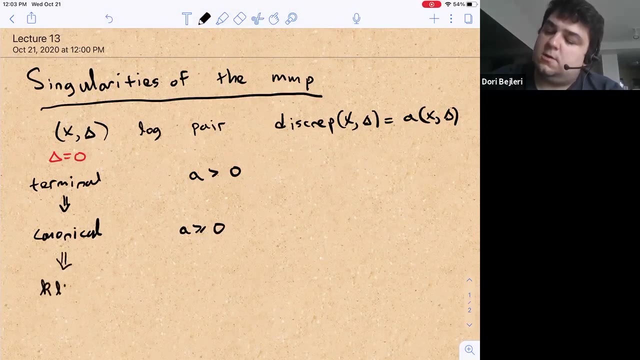 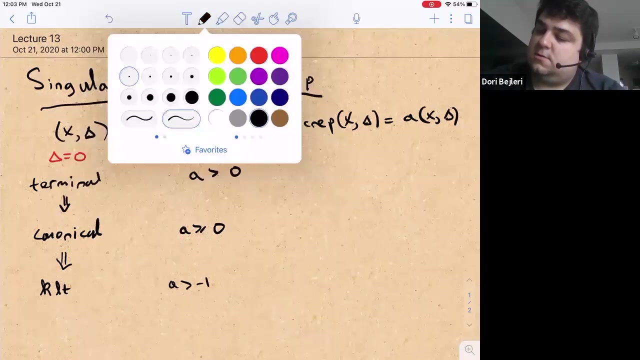 So when a was bigger than zero, we said this is terminal. And then if a is greater than or equal to zero, we have canonical. And then if a is greater than minus one and in general the round down of delta is zero, then we have KLT. 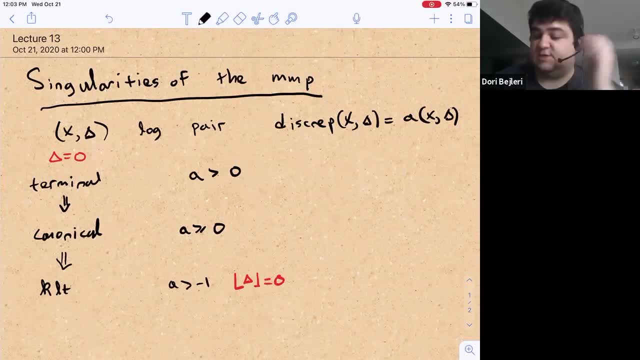 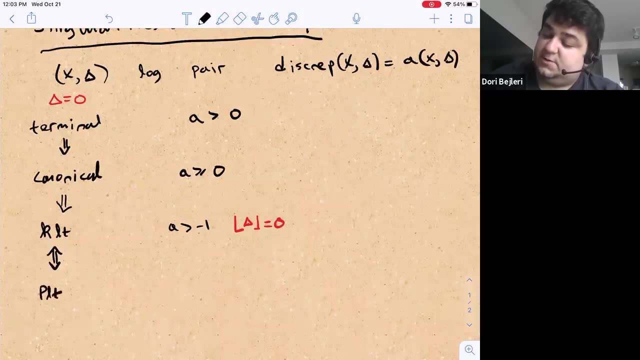 But on this side we're just going to consider quickly the case where the boundary is actually zero. And then we have on this side: KLT is the same as PLT because there is no boundary, So the condition is obviously satisfied, which is the same as DLT. which was this more complicated? 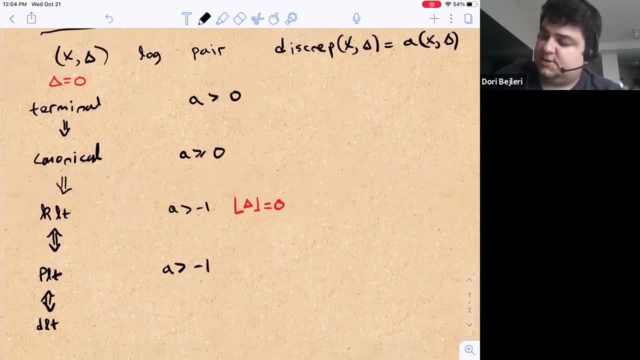 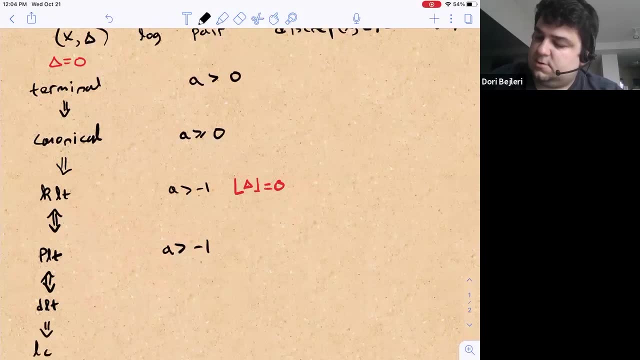 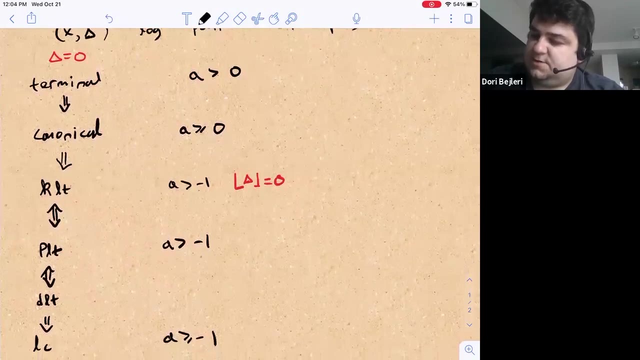 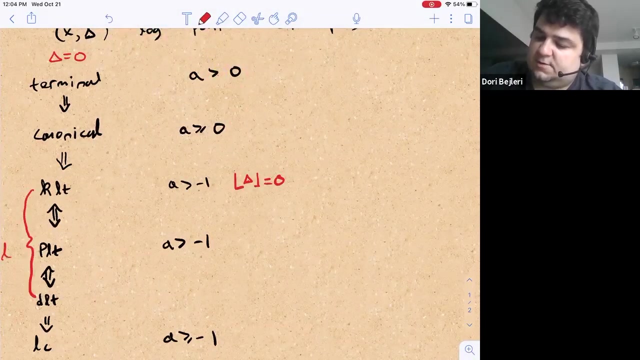 In other words, the condition is satisfied, which means that the boundary is no longer existent. And then we can see that we have the same question here, But again there's no boundary, It's equivalent. And then all this implies log, canonical. Okay, So these implications are true when there's no boundary, And so for that reason we'll just all three of these are sometimes is called log terminal when there's no boundary. So if you ever see lead x be log terminal, you know that comes into play. 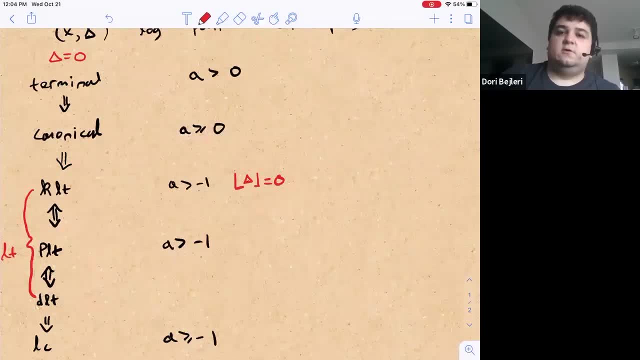 You're probably going to see that in your code. then it just means there's no boundary and this discrepancy condition is satisfied. But when there is a boundary it's slightly more complicated. There's just one implication that I said. that's not true. 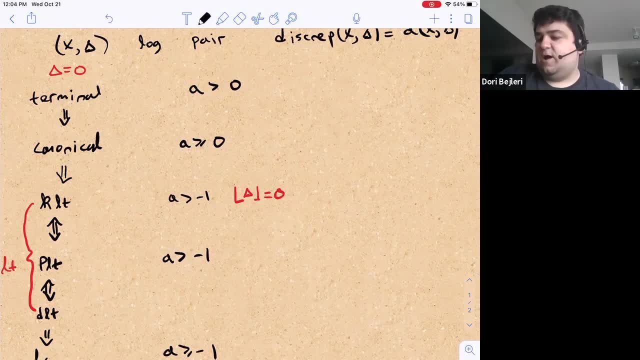 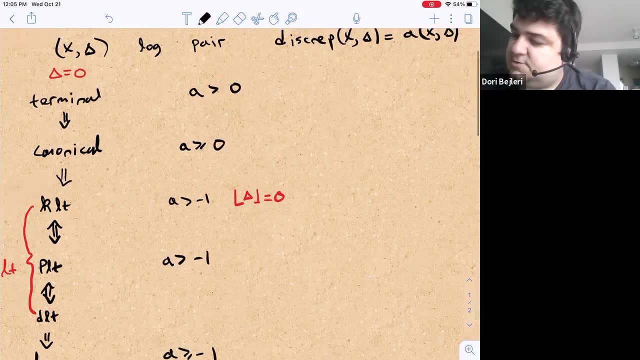 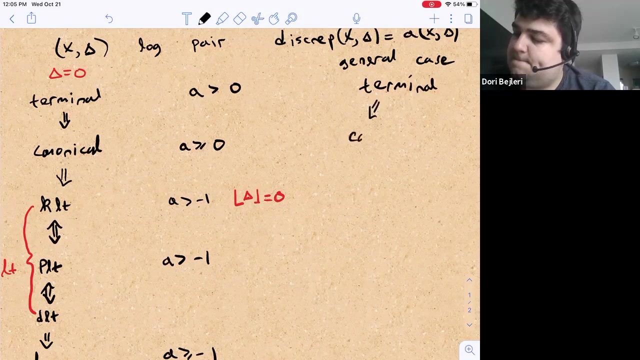 And it's exactly this: canonical implies KLT, one because of this round down condition. So in the case where the boundary is not empty, So general case, right on this side We have terminal implies canonical And terminal implies KLT. But canonical does not necessarily imply KLT. 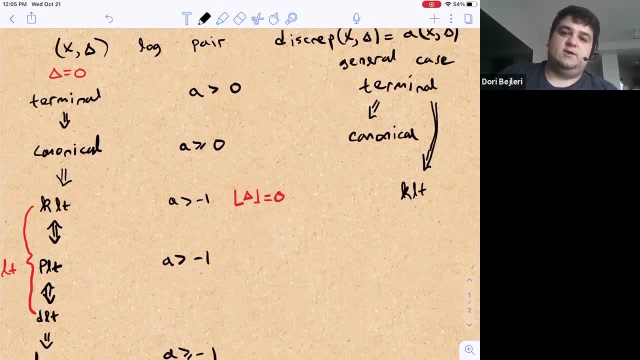 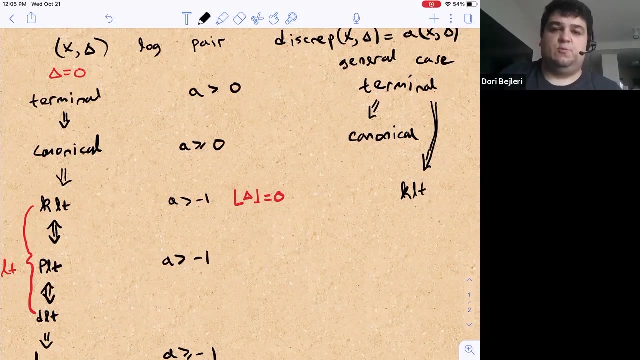 Just because you can't have a pair with canonical Singularities where the divisor is coefficient one. And this exactly happens when you have a smooth variety and a smooth divisor. So we have a smooth variety and a smooth divisor. then this round down condition isn't satisfied because you have coefficient one. 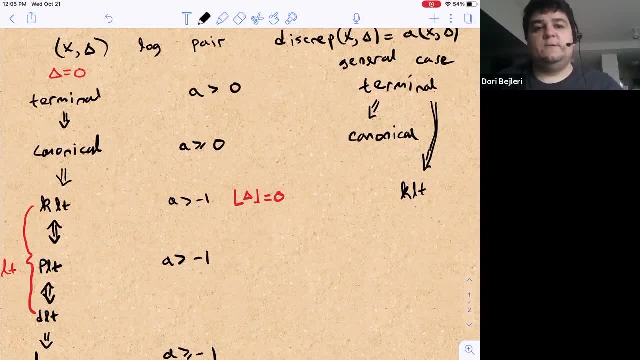 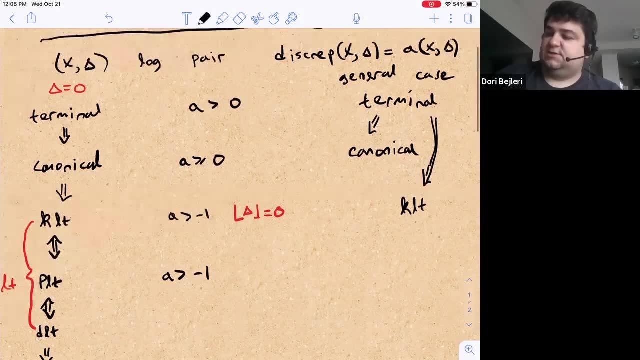 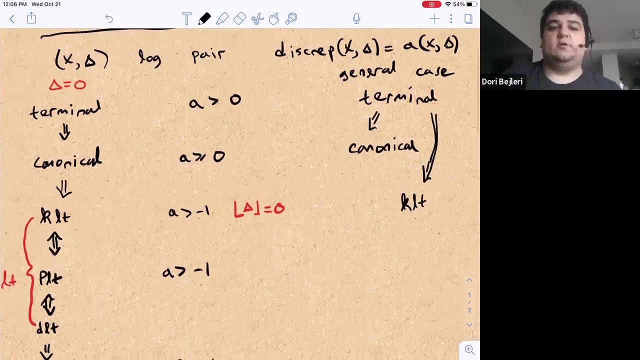 But all the discrepancies are actually greater than or equal to zero. So another way to think of it is that for the KLT condition you really want to look at not just the discrepancy but the total discrepancy, When you look at all divisors and not just exceptional divisors. 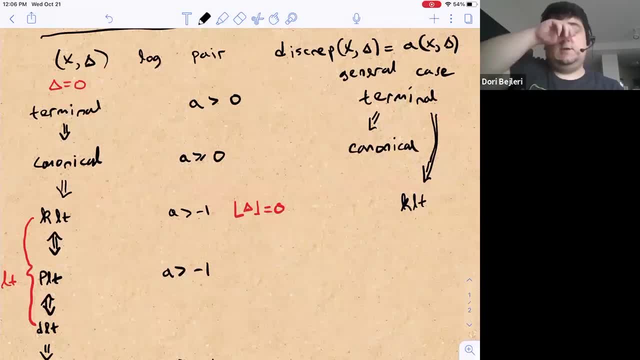 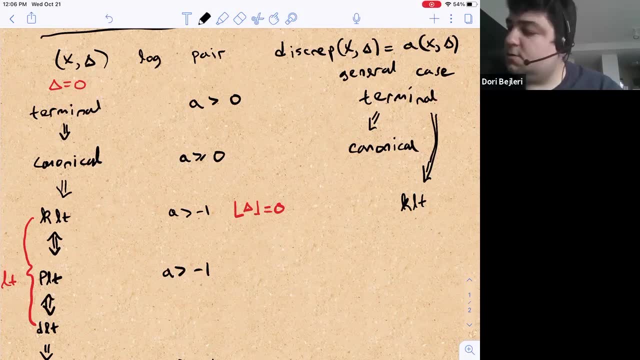 So you can rephrase this KLT condition as saying: the total discrepancy is greater than than minus one, And that exactly tells you the coefficients have to be smaller than one. But then canonical does imply PLT, And so does KLT, And then this implies: 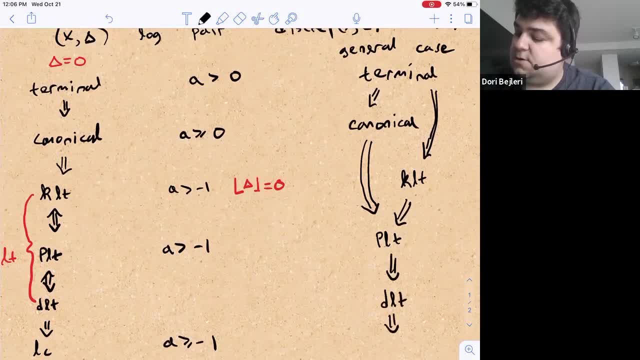 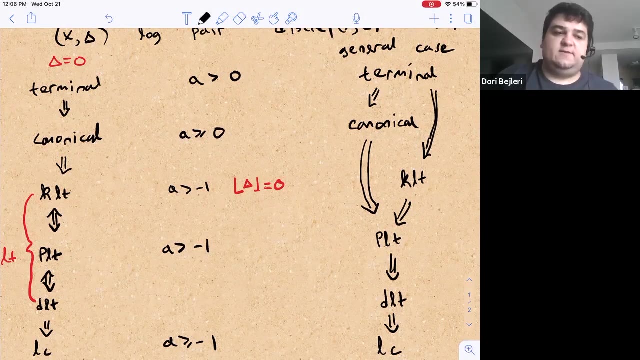 DLT, Which implies law, canonical and all of these are. all these arrows are actually just one way arrows in the whenever you have a non-empty boundary And I should say like this: this example where canonical is in KLT, the only like soon as you like, if X is smooth and you have singularities along your divisor. 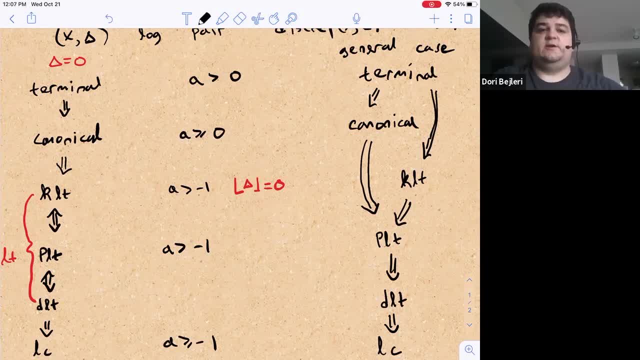 Then canonical will force the coefficients to be smaller Soon as you get singularities on your divisor Cause. then you have to actually do some blow ups and the multiplicity matters. So it's really it's only the case where, Where The divisor itself is smooth. 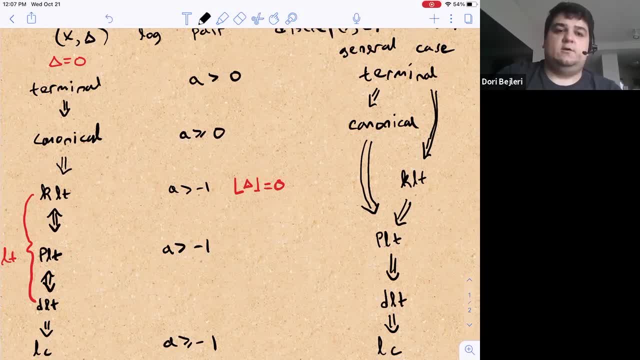 That you have this slight issue. Okay So, And let me recall the definition of DLT that we gave And I'll write it here. So he said: DLT, It was a condition that there exists a Z and X closed, Such that 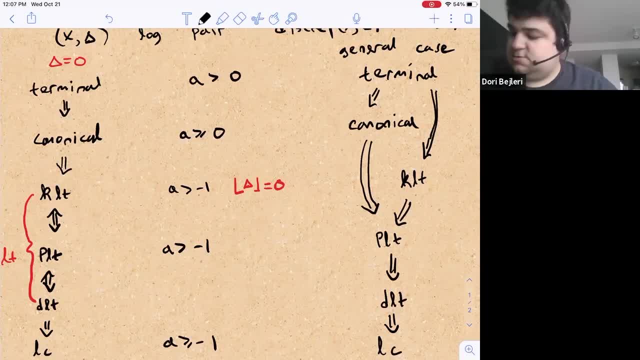 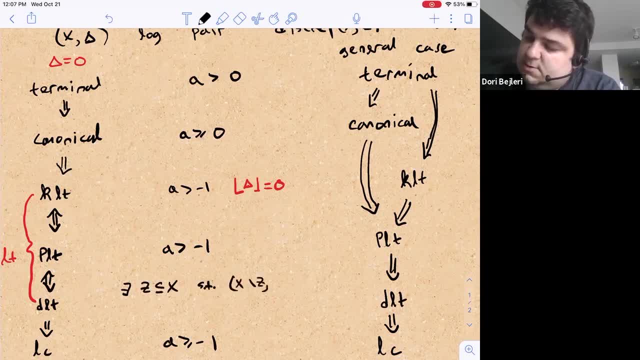 DLT, DLT, DLT, DLT. On preload, The pair X minus Z, Delta minus Z Is normal crossings. So simple, normal, normal crossings. It's really important. It has to be simple, Normal crossings And. 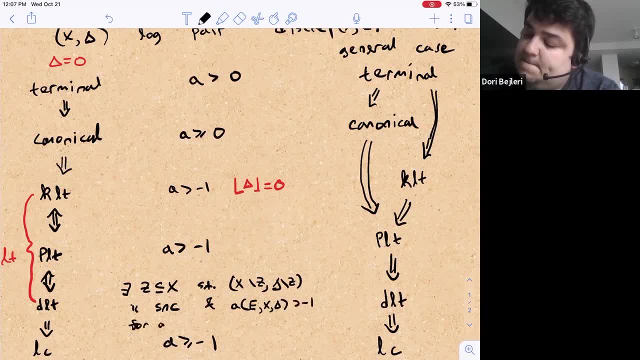 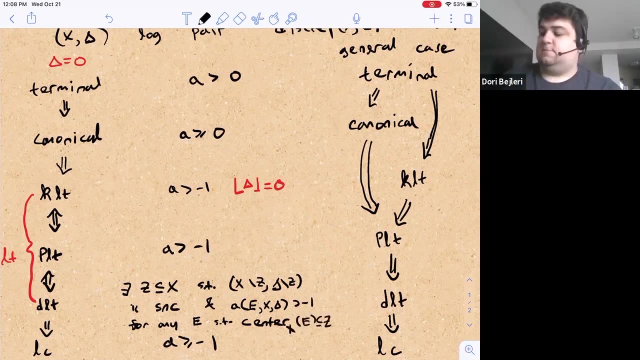 The discrepancies Are greater than minus one for any E lying over Z, Z. yeah, so so the definition is saying you have some locus where you have these discrepancies, uh, that are like the klt case or the plt case, uh, but then outside of that locus, maybe you have 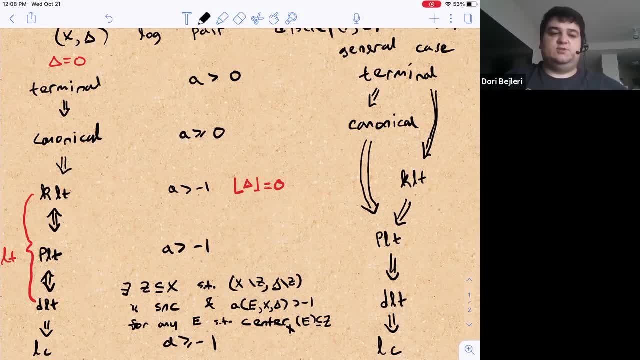 worse discrepancies. maybe you have strictly log canonical, but those strictly log canonical ones are just coming from normal crossings, so they're they're easier to handle, um, from simple normal crossings. so let me give a few continuity properties about how these, uh, how these singularity conditions behave under perturbations. 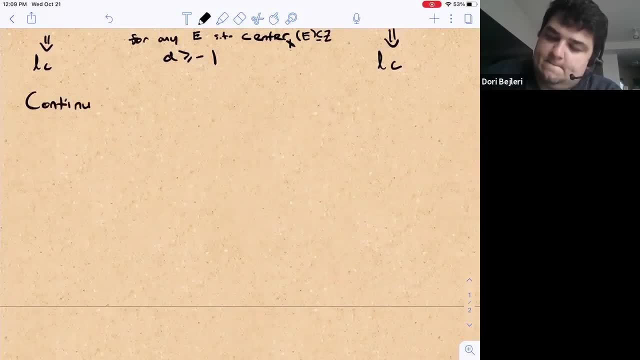 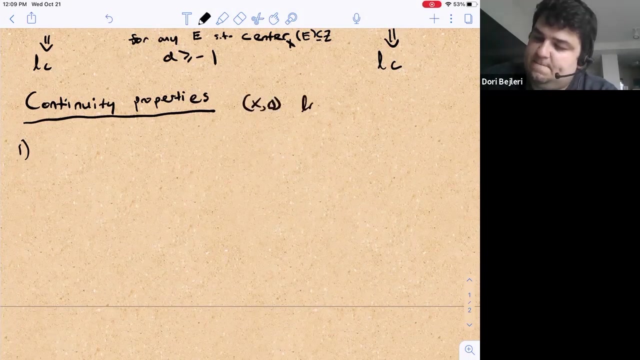 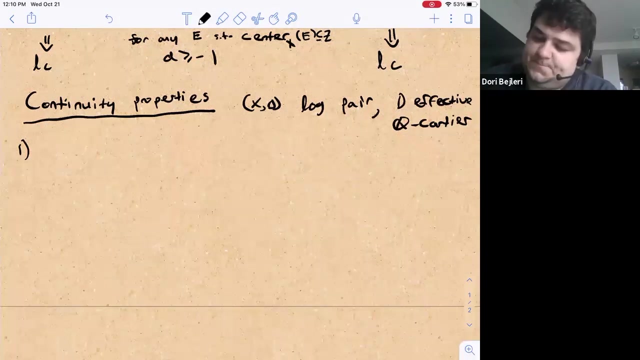 and uh, these are basically just from the, from the definition. so let's say, x comma delta is a log pair and d is effective in q cartier. so the the general question is just, if you perturb your delta by adding some epsilon d, uh, how do these singularity conditions behave? um so, first condition: if x delta plus d, 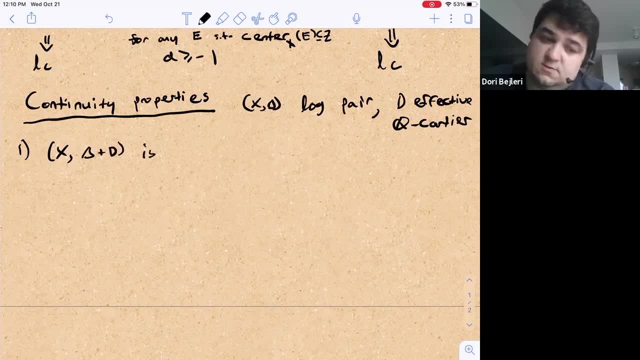 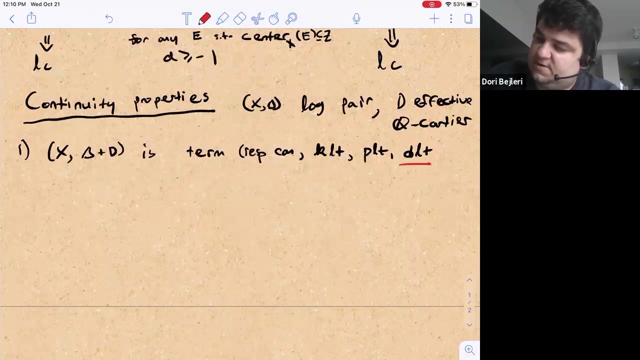 is any of the of the conditions, let's say uh, terminal, respectively canonical klt, plt, dlt. but in every time, in this uh, in what's following, every time we talk about dlt, we'll add the extra condition that uh delta is effective. that was part of the definition of dlt, actually. 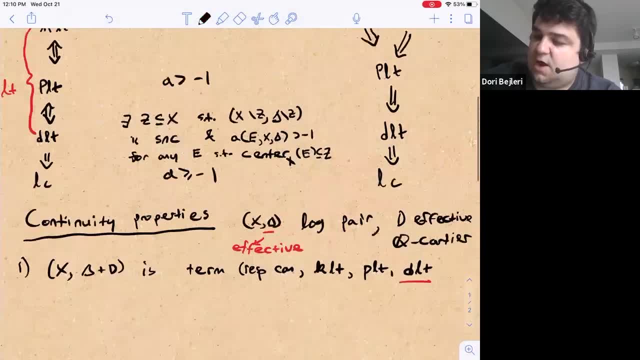 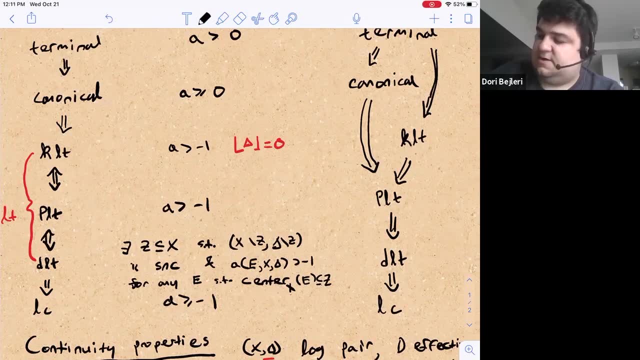 i should have said uh. so for all these other ones you can, you can talk about them, but i'm just going to talk about these singularities. uh, with your boundary having negative coefficients, even though that almost never actually comes up, uh, but the theory still makes sense for dlt. you really. 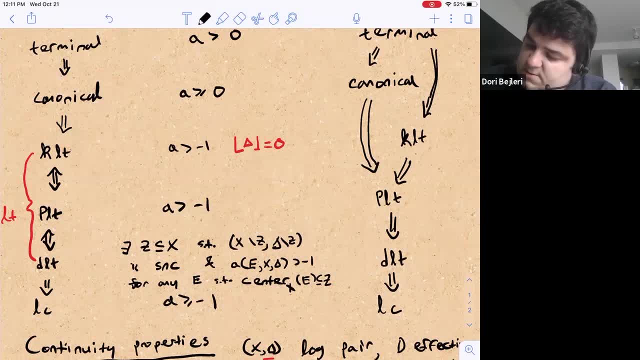 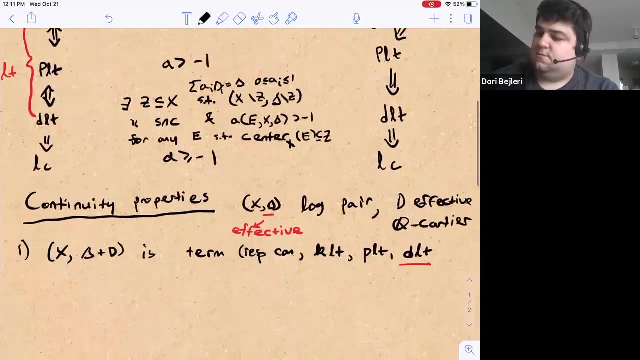 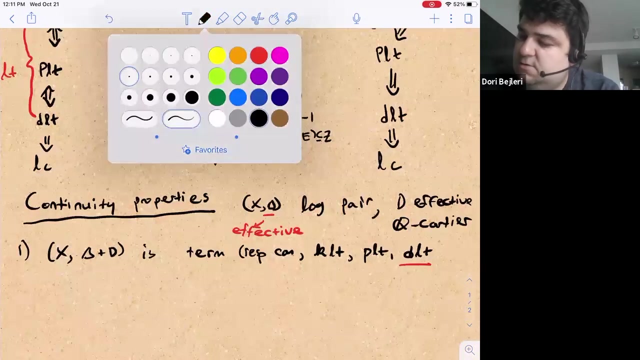 want uh that the coefficients of delta are between uh zero and one, only for the dlt case. so so, so, so, so, so, yeah. so in what follows, assume uh effective whenever we're talking about dlt. otherwise you don't have to assume effective. but in all applications delta is effective, so it's not too big of a deal. 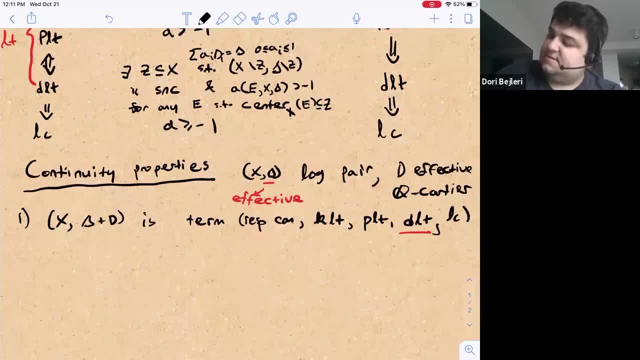 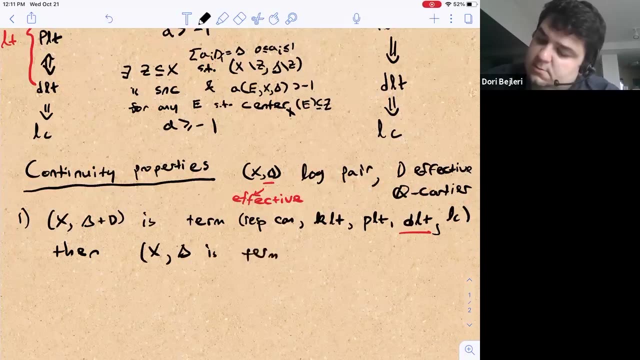 so if you have that x comma delta plus d is any of the singularity conditions where d is some effective divisor that you've added, then x comma delta also, so it has, uh, has these singularities, um, so this says that uh. so this says that, uh, that if you have, if you subtract something, 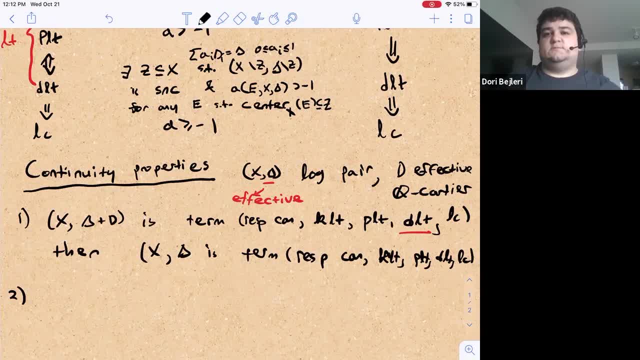 that if you have, if you subtract something, then the singularities can't get worse, then the singularities can't get worse. that's essential to saying um, ours we have now. temperatura is one of the global conditions for uh dlt and um dlt can tanta dlt has a fugacity of破יל. 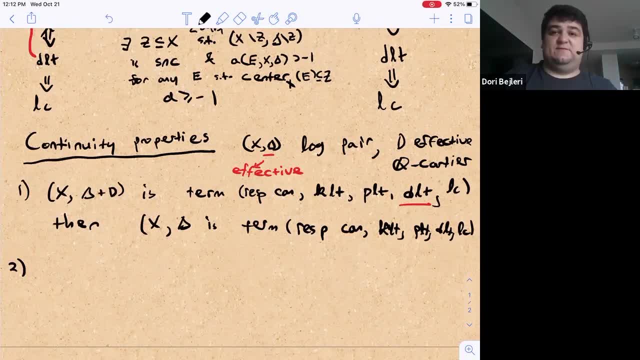 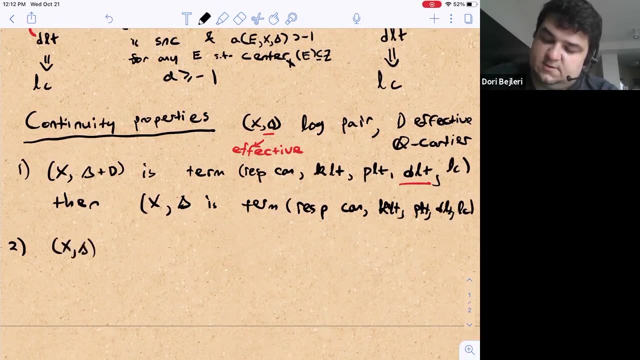 Lemma from two classes ago that I didn't prove. I left as an exercise that when you add an effective divisor the discrepancies get smaller. So when you remove an effective divisor the discrepancies get better. Two: if x, delta is terminal or respectively KLT. 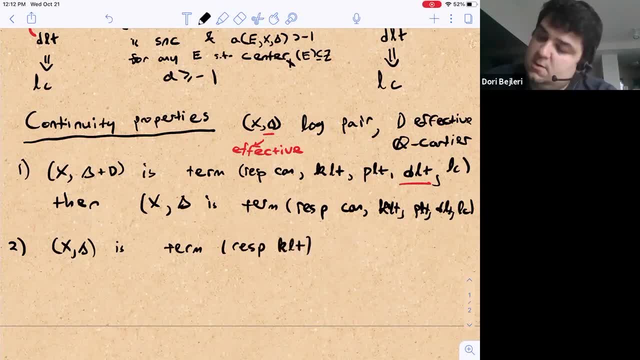 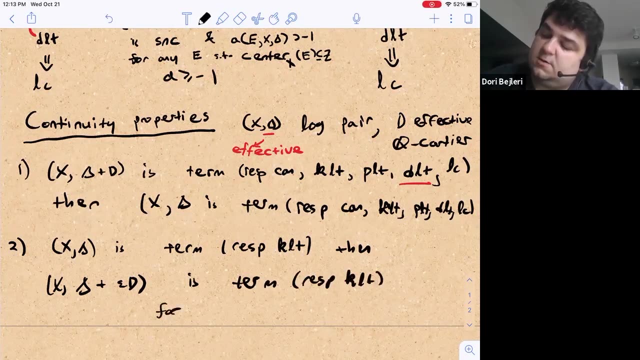 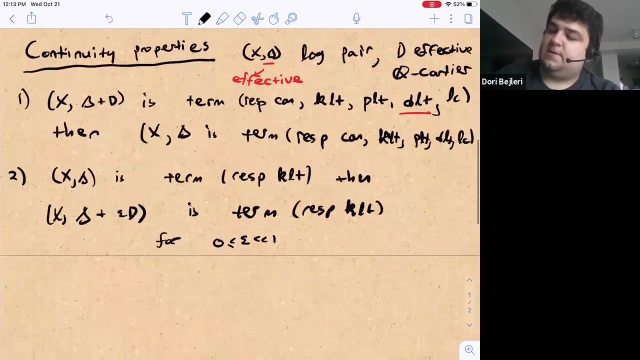 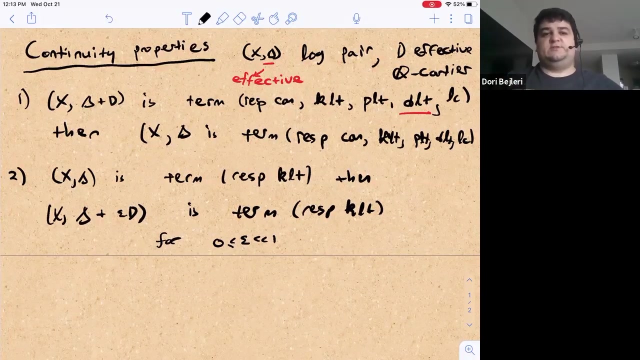 then x, delta plus epsilon d is also terminal, or KLT for epsilon small enough, And so this is one of the nice things about KLT is that it's really an open condition. That's why it's so important. You can perturb your divisor by some small epsilon and you still lie within KLT. 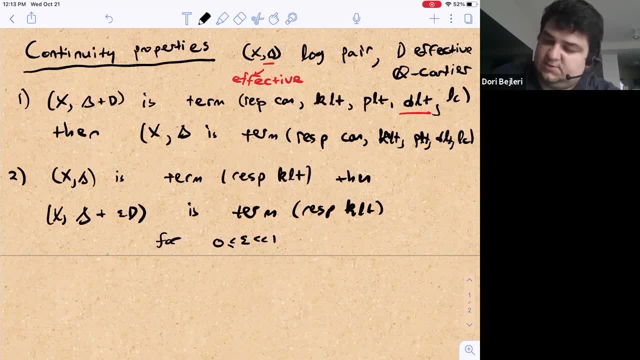 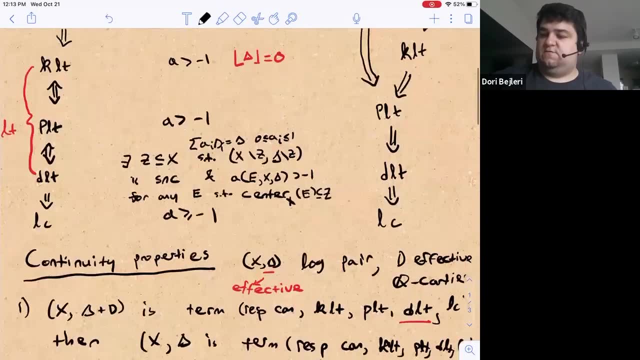 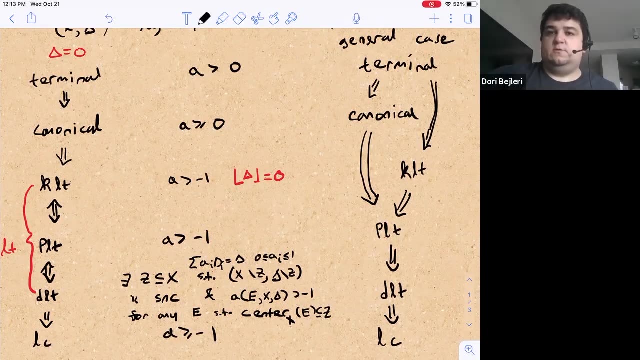 For PLT and DLT it's a little more complicated because you need to control the places where the coefficients are one. So this is what's nice about the condition of rounding down being zero. for KLT, It doesn't matter what you add, as long as the coefficient is small enough, you won't break the discrepancies. 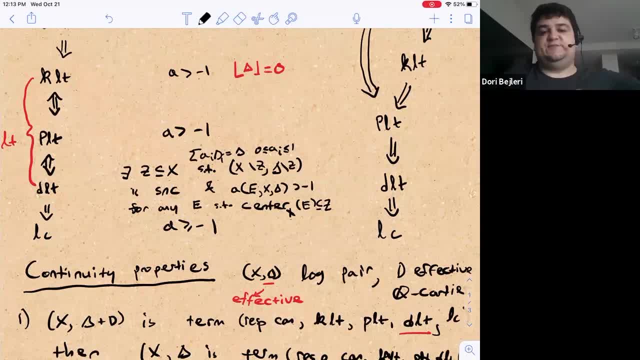 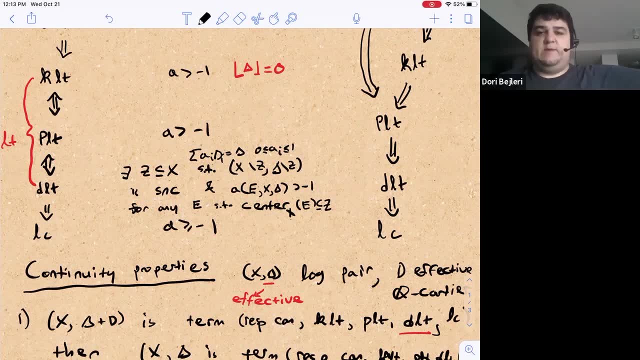 But for PLT and DLT you need to be a little careful, because you might have some coefficients and you can't add anything to that divisor without making negative discrepancies, Essentially because of that example where we showed that if you have a divisor whose coefficient is strictly smaller than minus one in the discrepancy 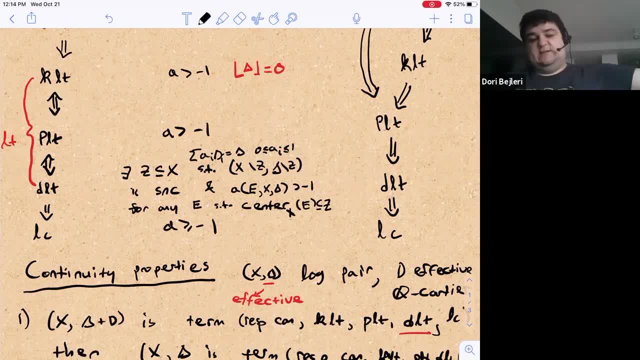 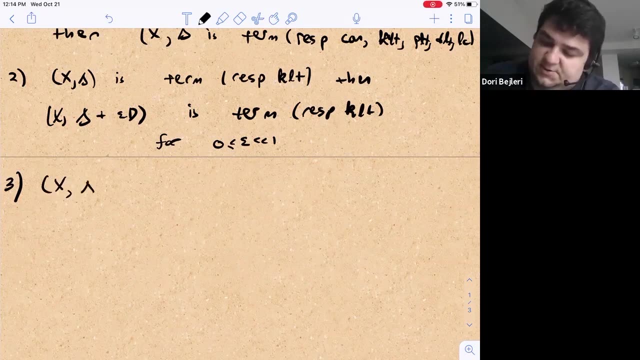 then you actually have discrepancies that are minus infinity. So as soon as you have this divisor that has coefficient, one, which is allowed in the PLT and DLT case, you have to make sure that you're not adding anything to it. And so for PLT and DLT, the analog is: this is true as long as you are careful about what divisor you add. 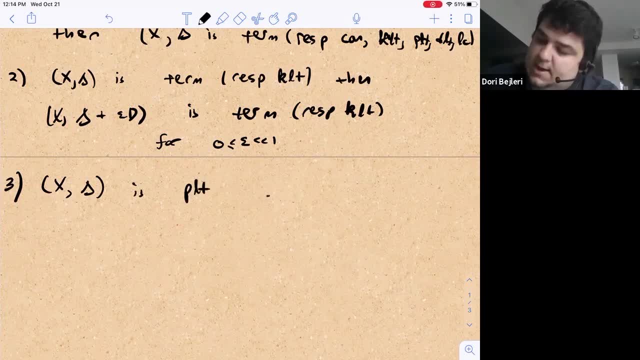 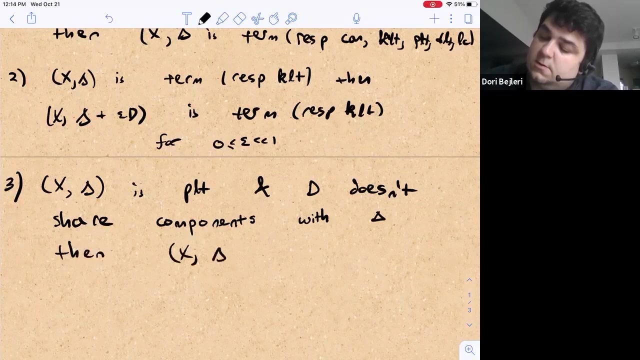 So if X comma delta is PLT and D doesn't share any components with delta, then X comma delta plus epsilon D is PLT for small enough epsilon And similarly for DLT. this is true as long as you are careful about what divisor you add. 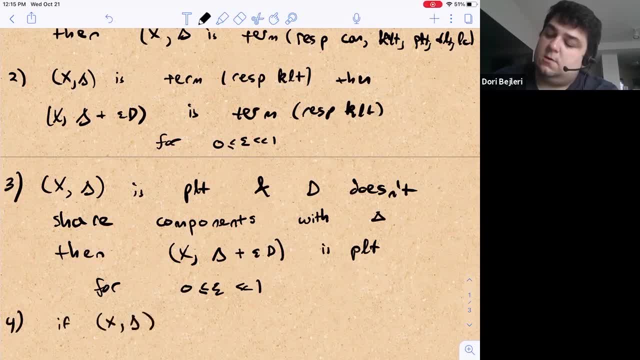 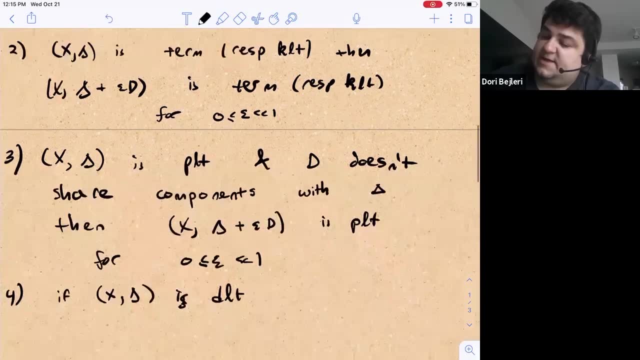 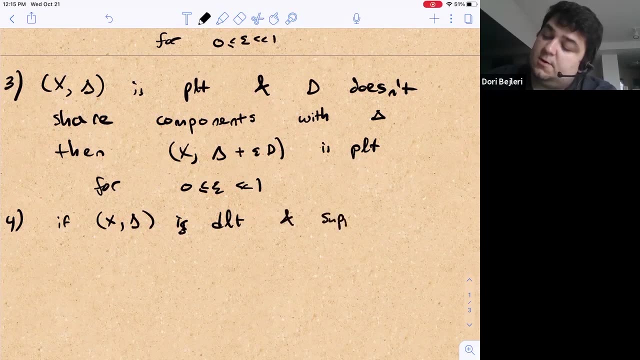 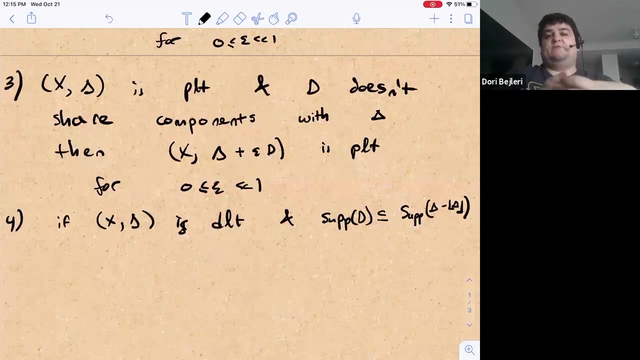 So if X comma delta is PLT and D doesn't share any components with delta, the easiest condition to try to impose is that the support of D is contained in the divisors that have small coefficients. So, basically, so if I look at only the divisors that have coefficient less than one, 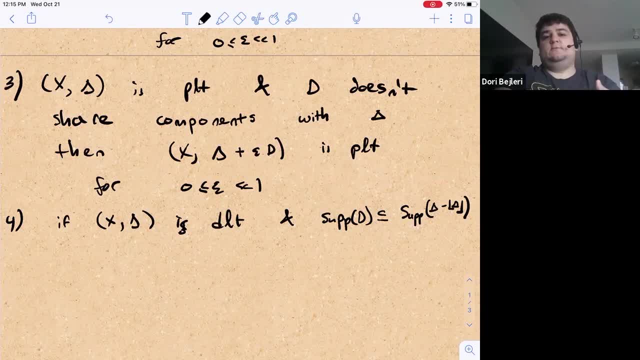 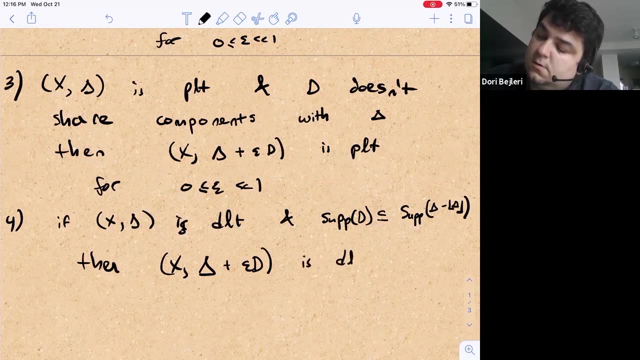 then I'm allowed to perturb those and still be DLT. And then, finally, the last one is saying that the canonical ones, that canonical and log canonical, are like the closures of the terminal ones. So let me write it for log canonical. 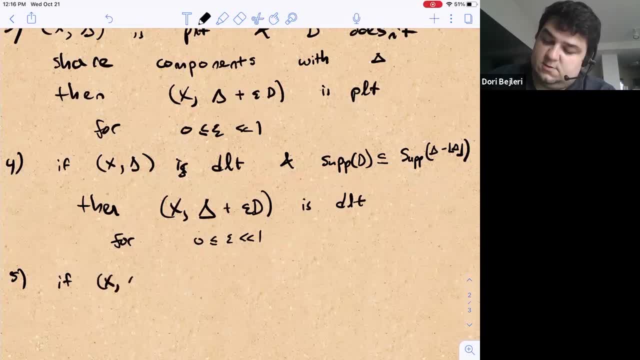 first, sorry for just canonical first. So if X delta is terminal, then X comma delta plus epsilon D is PLT, then X comma delta plus epsilon D is PLT, then X comma delta plus epsilon D is PLT, then X comma delta is canonical. 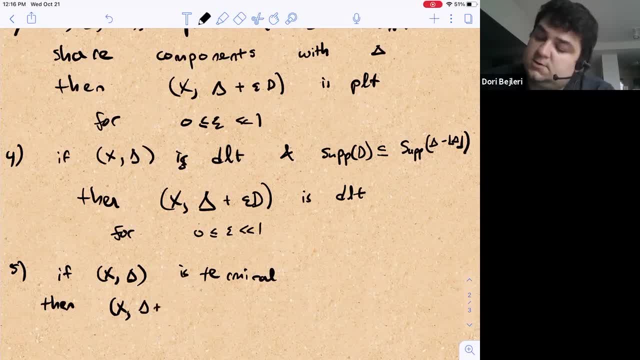 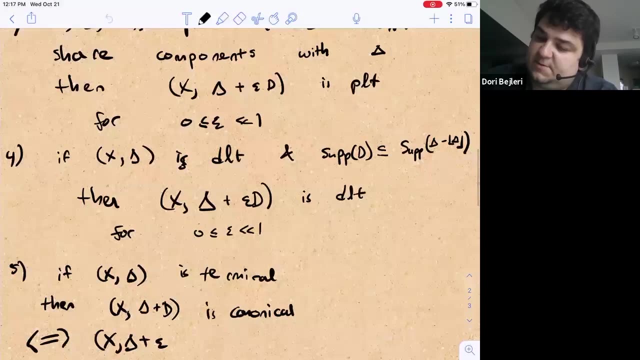 sorry, X comma delta plus D. So then when we add this extra divisor we get something canonical if, and only if, X delta plus epsilon D or plus CD. now, because it doesn't have to be infinitesimally small, plus CD is terminal. 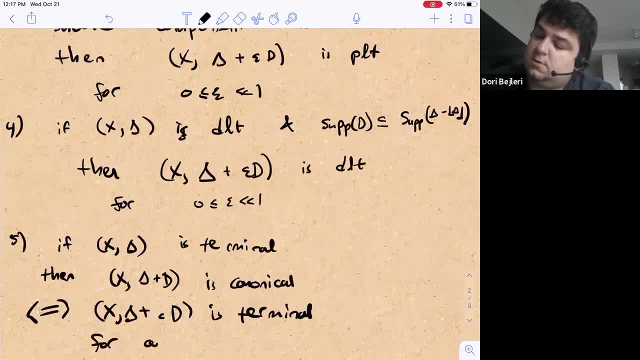 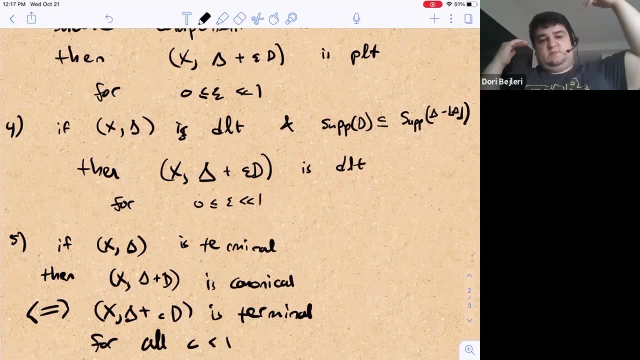 and it's optimal for all C less than one. So it's saying that if you add something and something that's actually canonical than any smaller numbers, soon as I take one minus epsilon times D, I actually have to be terminal. So kind of canonical is the boundary of terminal. 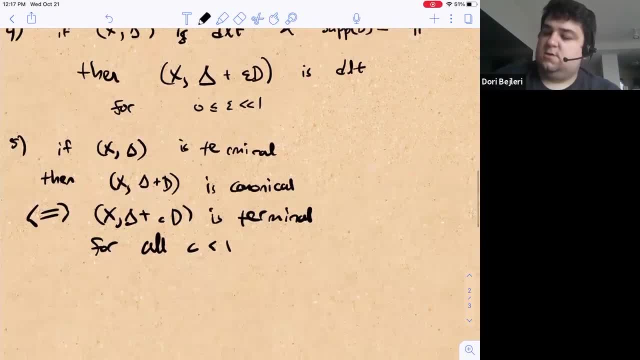 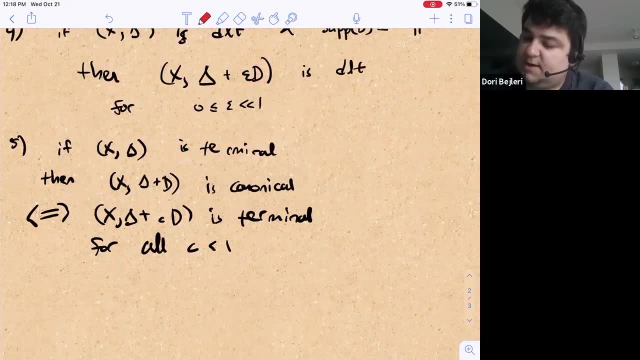 Let me modify this for those two. let us how: Yeah, So if Z, dot delta D, or for the log case. So in the log case, if we assume that the pair is KLT, PLT or DLT, then x comma delta plus D is log canonical. 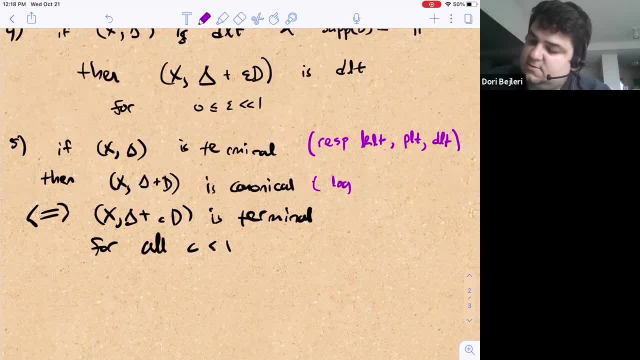 So in any of the three log terminal cases then when we add D we get something log canonical if, and only if, the pair delta plus CD is KLT, PLT or DLT for all C less than 1. So if we have something KLT, then when we add D. 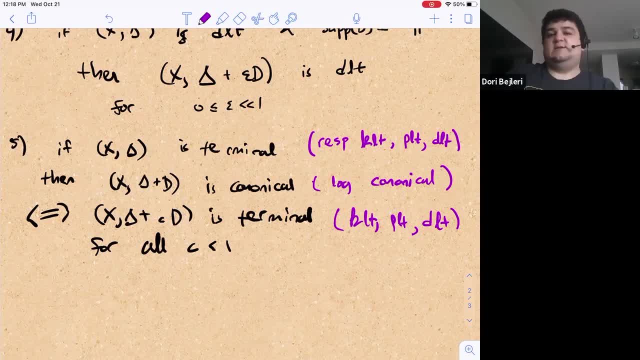 we get something log, canonical if, and only if. whenever we add 1 minus epsilon D, we get something that's still KLT, And similarly for PLT and DLT. OK, a few more propositions and definitions before I can do a bunch of examples. 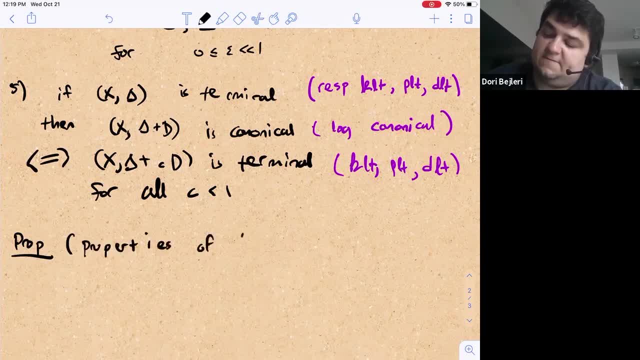 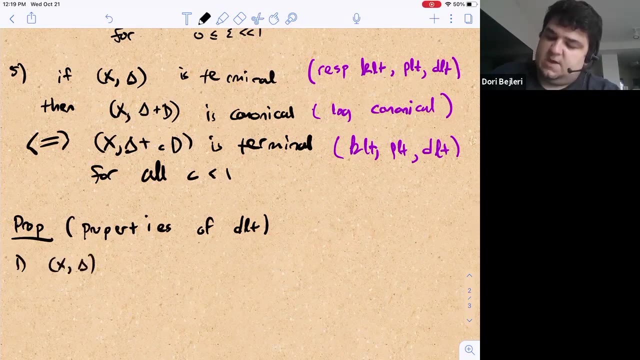 So here are two properties of DLT, And I waited till after continuity results to state them because They really use the continuity results, even though I won't write down the proofs in full detail. So the first one analogous to the other ones. 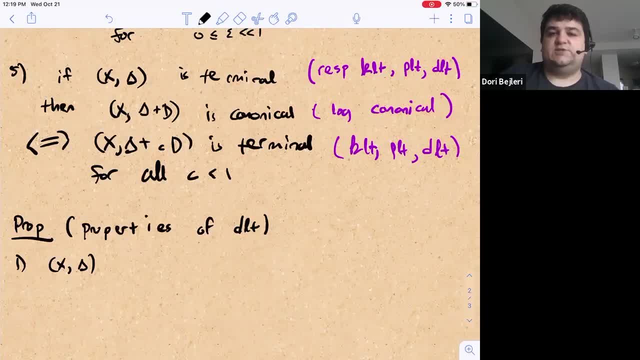 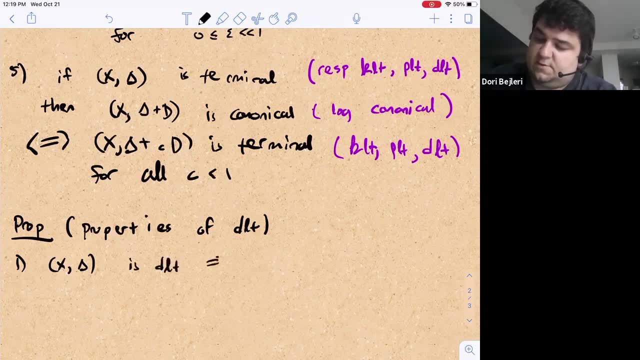 where we showed that you only need to check one resolution to check any of the other properties. the same is true for DLT. So x comma delta is DLT if, and only if, there exists this closed subset z, such that x minus z, delta minus z is SNC, and there exists a resolution such 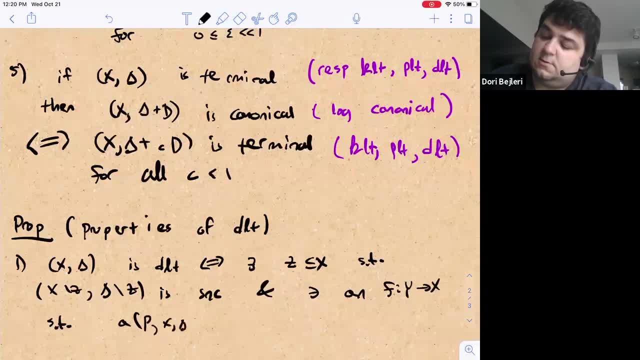 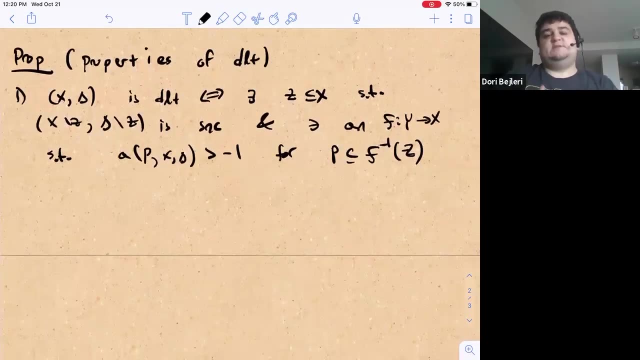 that the discrepancy of any prime divisor is greater than minus 1 for any p lying in F inverse of z. So again, this is saying that your DLT, if you have this, this subset, away from which your simple normal crossings, and then you have a resolution where every discrepancy 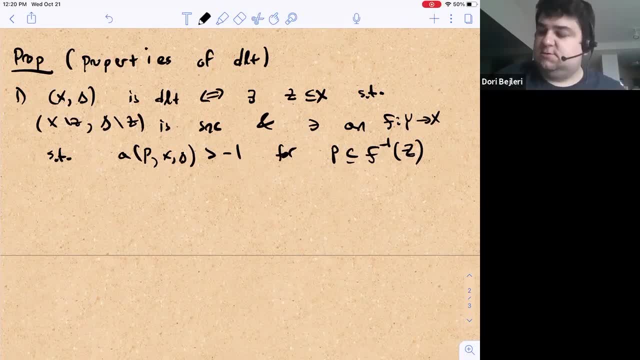 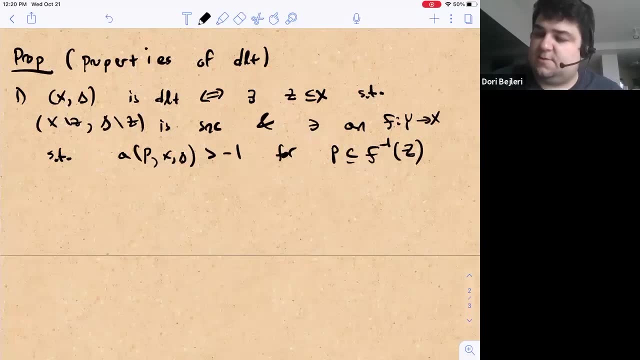 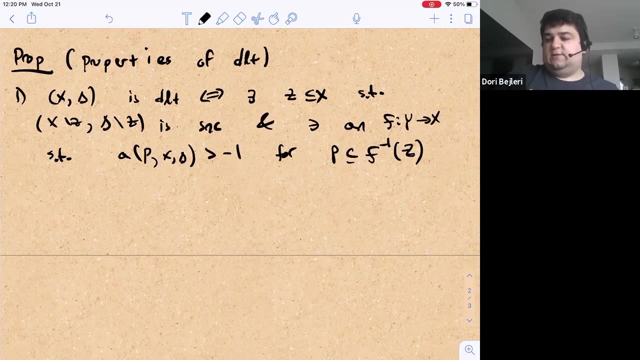 over that z is greater than minus 1.. So you only need to check one resolution rather than the definition, which said just any exceptional over that z had to have discrepancy greater than minus 1.. OK, and the proof of this, essentially, is like we've done before, where you pick a resolution. 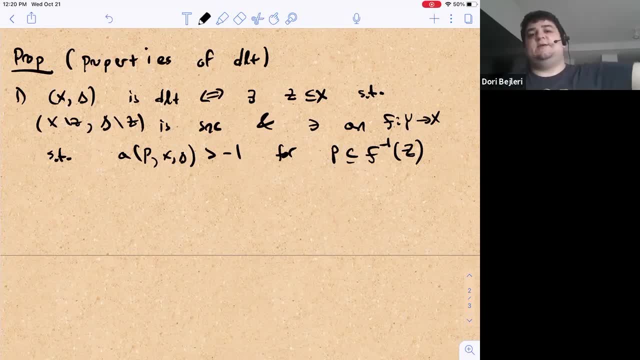 and you put the right divisor upstairs so that the discrepancies downstairs are the same as the discrepancies upstairs. And now you use that. you have this extra wiggle room that all your, except like all the divisors inside of F, inverse of z, have to have coefficient strictly smaller than 1. 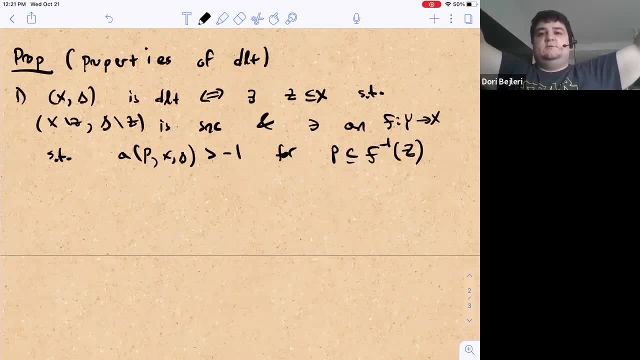 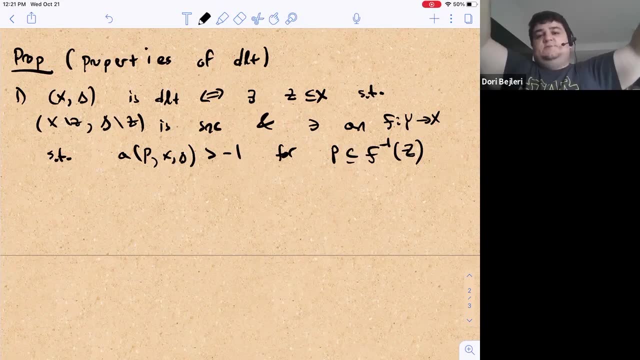 in your divisor upstairs, in your boundary divisor upstairs, because of the definition of DLT, And so you have this extra wiggle room where you can add any, like some small epsilon of these divisors and still get something that's log, canonical by these continuity results. 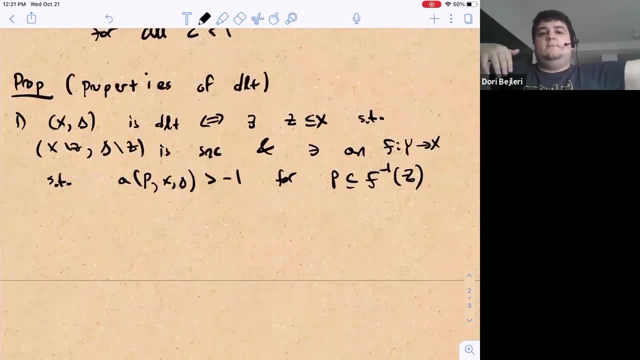 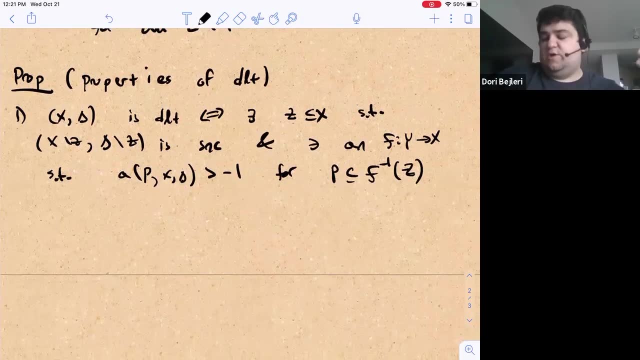 But when you add this epsilon you make the discrepancy strictly smaller. And so when you make the discrepancy strictly smaller and still get something log, canonical, then all the discrepancies you had had to have been strictly bigger than minus 1 over those divisors. So it uses this kind of perturbation. 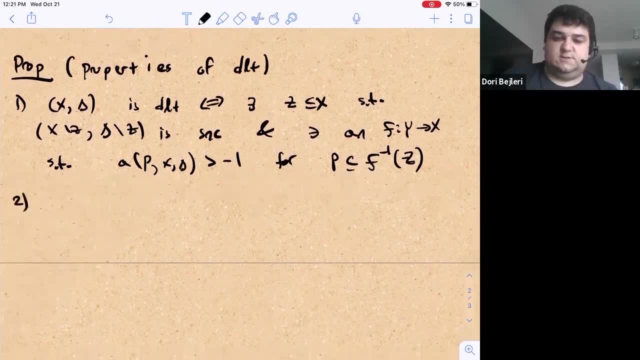 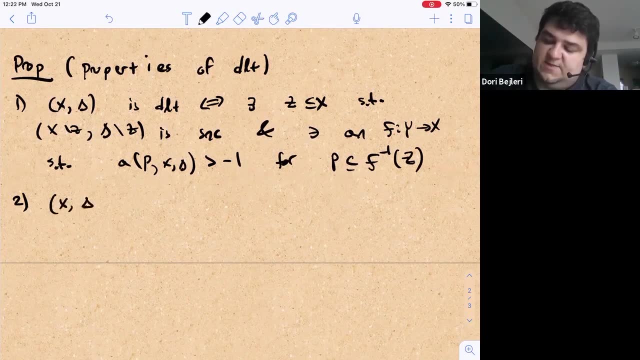 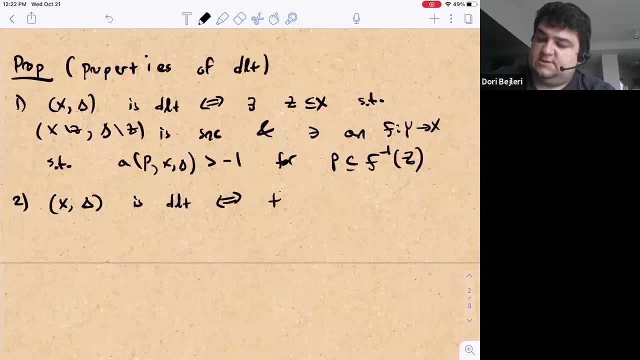 but essentially the same idea as the other versions of this proposition. A more involved one, which is maybe the easiest definition of DLT to digest but maybe a little harder to work with, is that x comma delta is DLT if, and only if, there exists a log resolution. 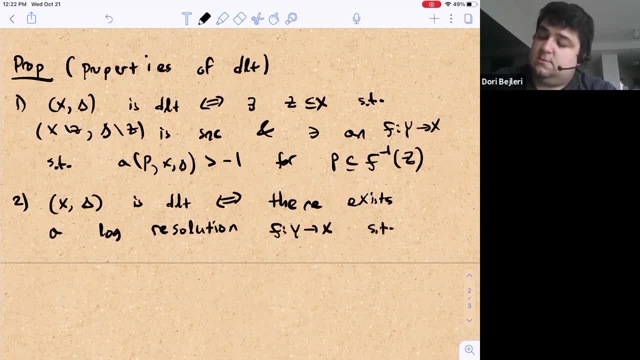 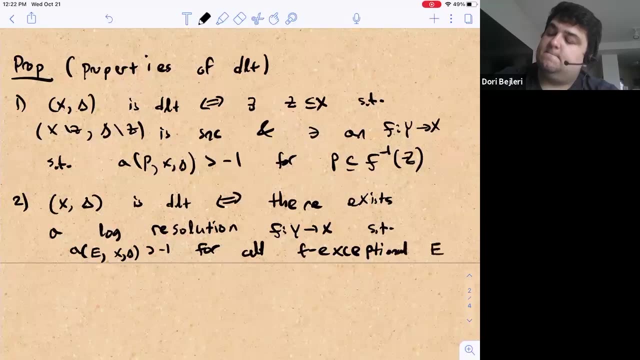 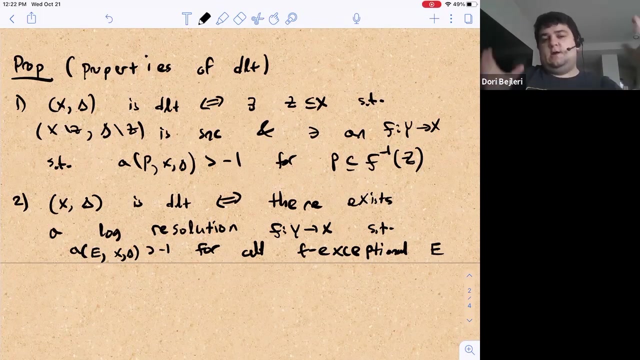 f from y to x, Such that the discrepancies are greater than minus one for all f exceptional divisors. So this one is saying that your DLT if, and only if, there exists a resolution where the discrepancies on all exceptional divisors of that resolution have are greater than minus one. 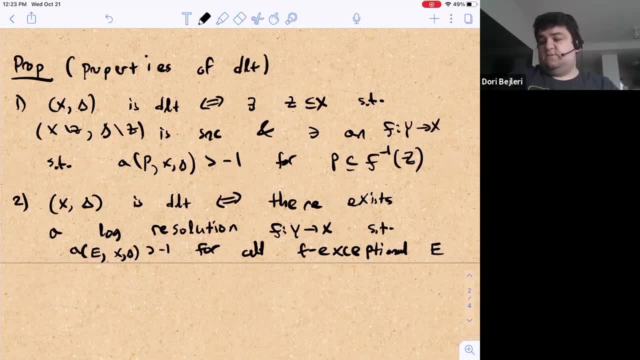 So here you actually have to be careful about the resolution you pick. You can't just pick any resolution, because if you're in the normal crossings locus away from the z and you start blowing up at some point where two of your of your snc divisors intersect, 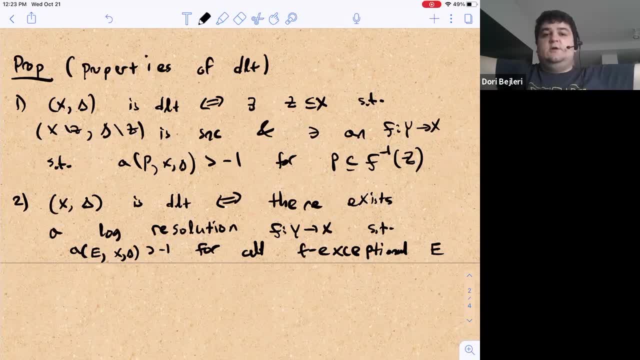 then you'll get a discrepancy that's minus one for that exceptional And so the the content of two is that when you're doing resolution of singularities, you can actually control the resolution that you build. so you only resolve the z, You only have to blow up inside of the z. 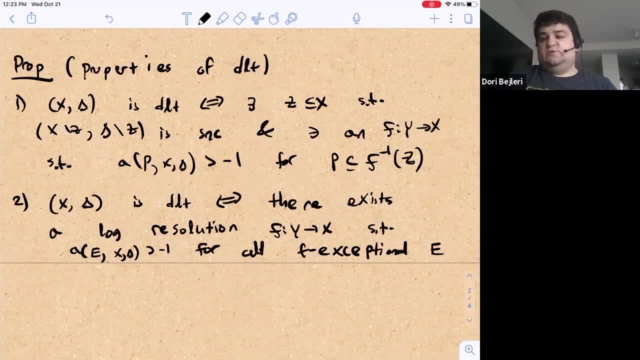 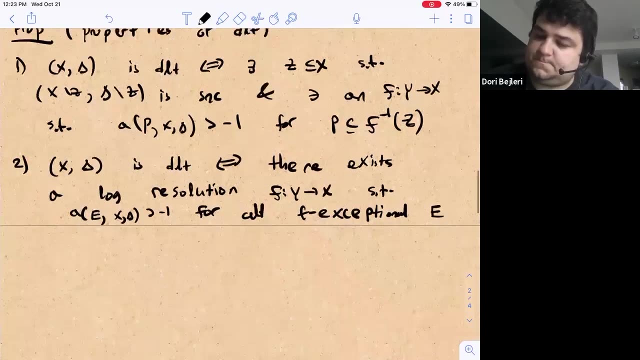 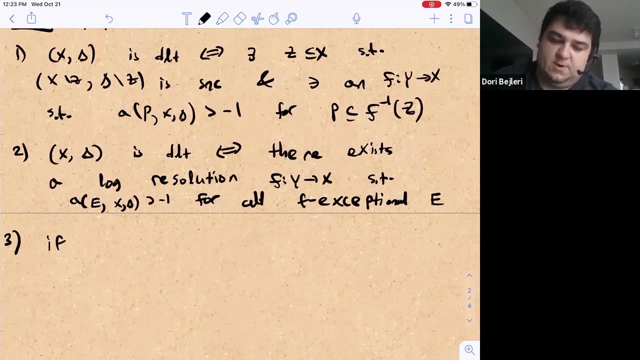 because you're already snc outside of z, And so to prove the equivalence in two, you actually need to control how you resolve singularities, which is why it's a more subtle definition for DLT than the previous one. And then a property: if we know that x comma delta is d. 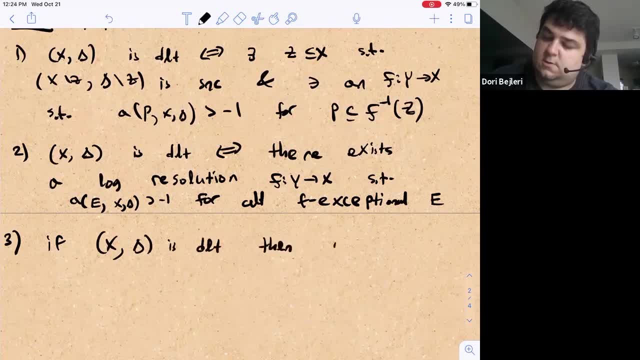 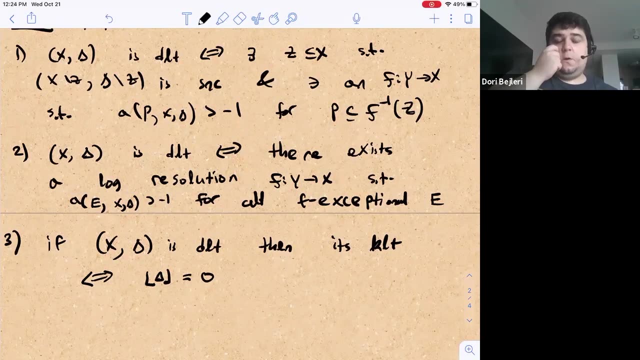 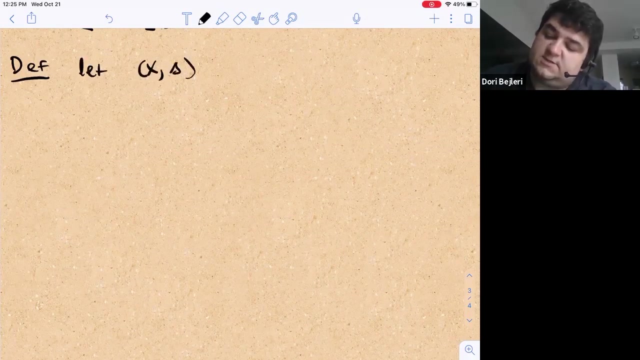 dLT, then it's KLT if, and only if, the round down is zero. So it's saying that the gap between KLT and DLT is this round down condition. So let x comma delta be a log pair, Then a non-KLT place. 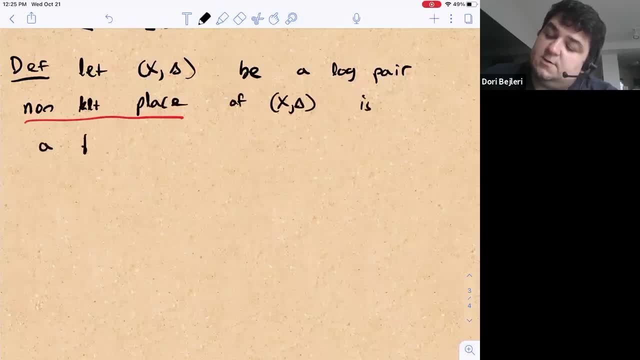 of x comma delta is a divisor p lying over x, So some prime divisor p lying over x with discrepancy less than or equal to minus one. And then a non-KLT center is a closed sub-variety of x comma delta. that's the image of one of these divisors. 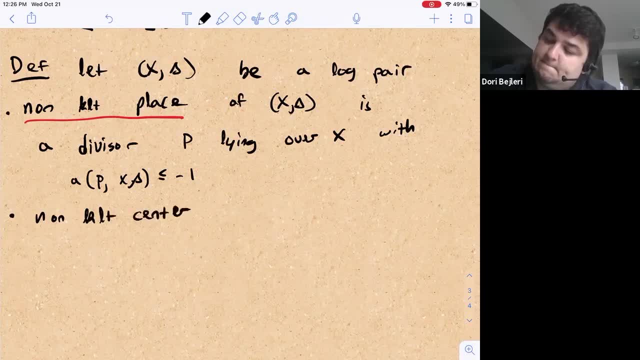 So that's the image of one of these divisors. So the original value is just the DLT. It's simply the non-KLT function and the variable part of the DLT is the state of the non-KLT. So that's primarily going to be the value of the non-KLT. 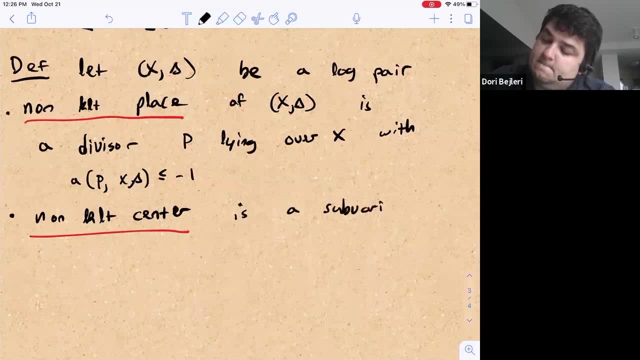 Now you could have known that if you were to do a simple DLT condition with the non-KLT function that you were looking for- the non-KLT function available at the end in the case file- the system will confirm that you got the non-KLT function. 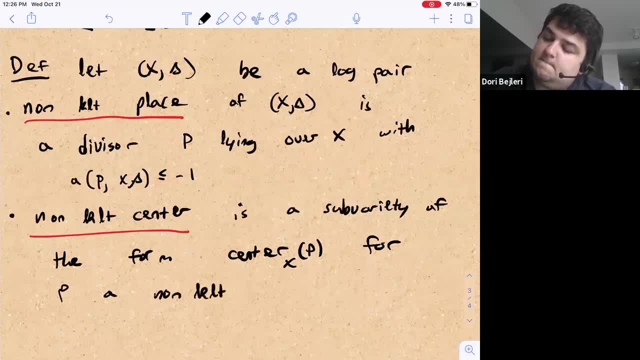 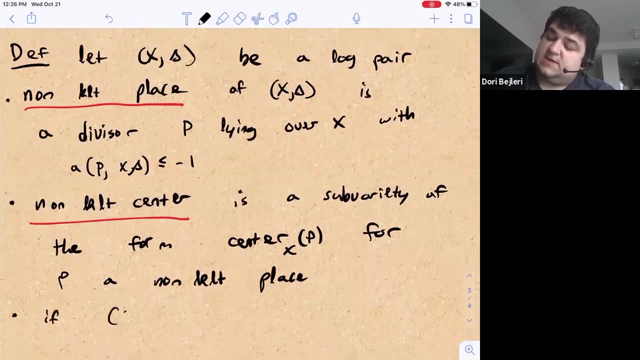 So if you want to take a look at the non-KLT function and see the difference between those two, like the non-KLT and the non-KLT function, that's the non-KLT function, So some kind of a median, If x comma delta happens to be log-canonical. 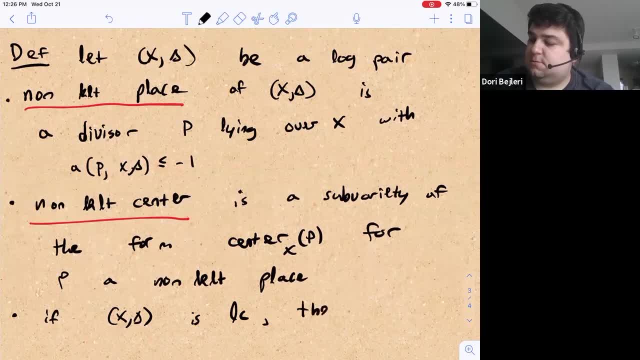 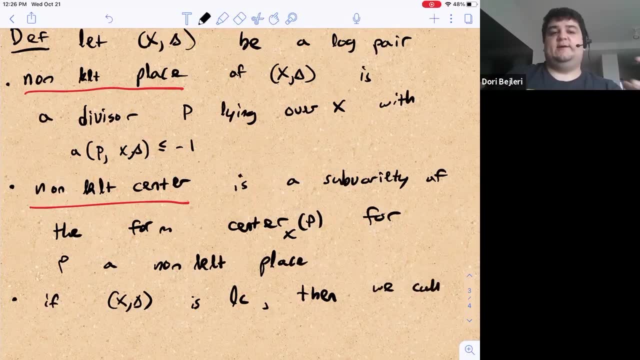 then we call the non-KLT centers log-canonical centers, Because that's the place where the singularities are strictly log-canonical rather than KLT. Is this too low, Like? where's the cutoff? Oh, that's good, OK. 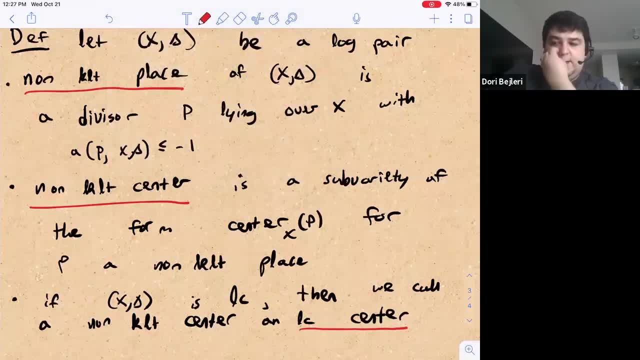 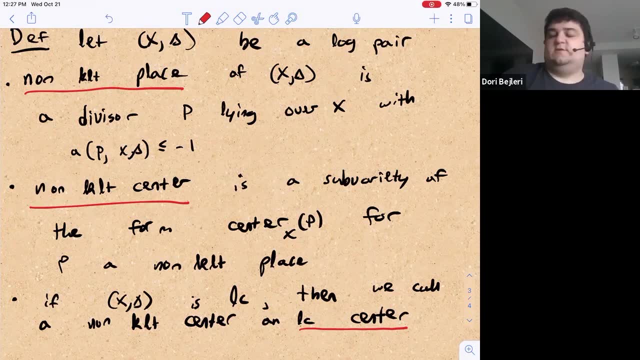 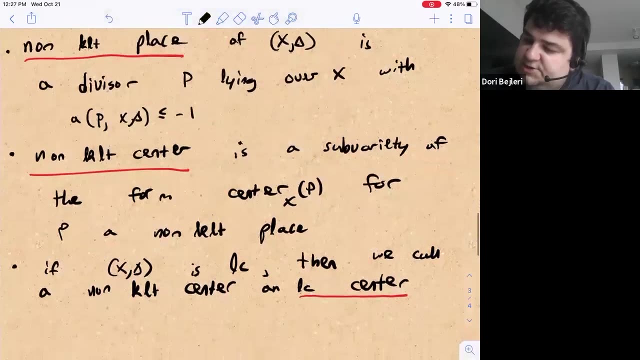 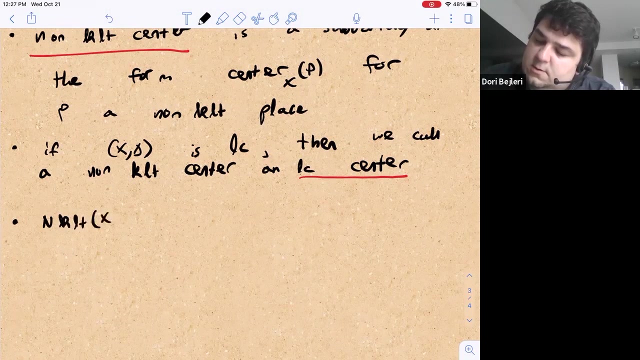 So often in literature you'll see log-canonical center. But that definition only makes sense when you know you're parallel. A pair is actually log-canonical, So it's good to kind of define both And then some notation will denote by nKLT. 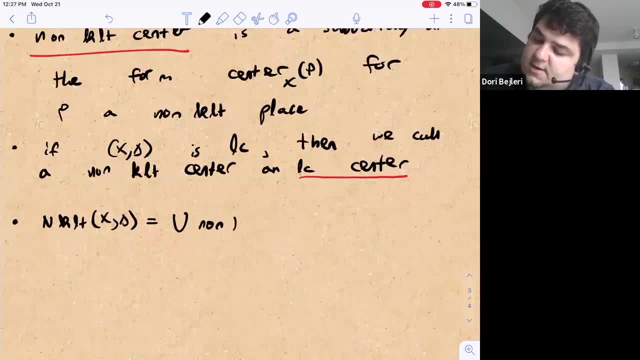 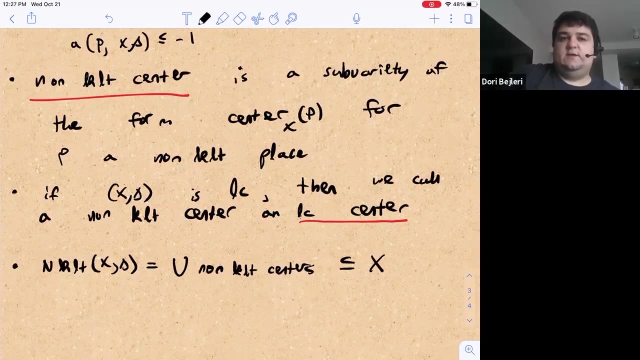 the closed sub-variety, which is the union of all non-KLT centers. So of course, here we're using the fact that you can test KLT on one particular resolution to know that there are only finally many of these centers. 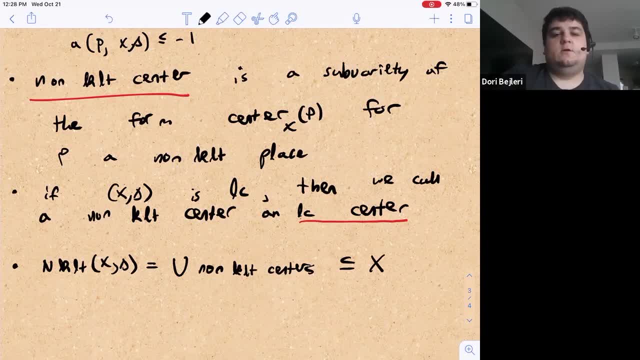 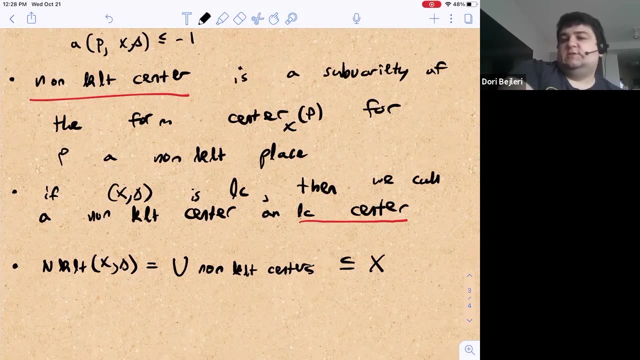 OK. So any questions about that definition And a lot of the game here will be that we can control what's happening away from the center. OK, OK, So we can control what's happening away from the non-KLT locus using vanishing theorems. that. 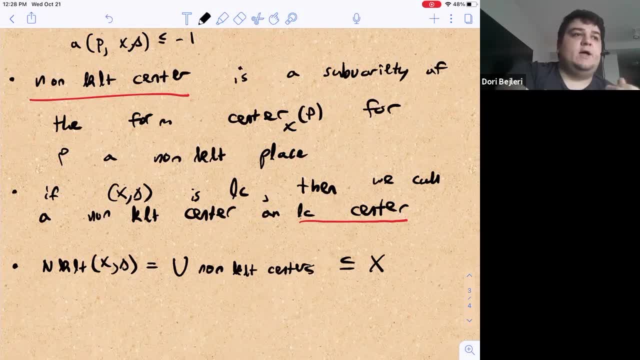 will start proving, hopefully in like 10 minutes, And then you need to understand what's happening at these log-canonical centers. So a lot of the game of working with log-canonical varieties is that you have some linear series you want to understand. 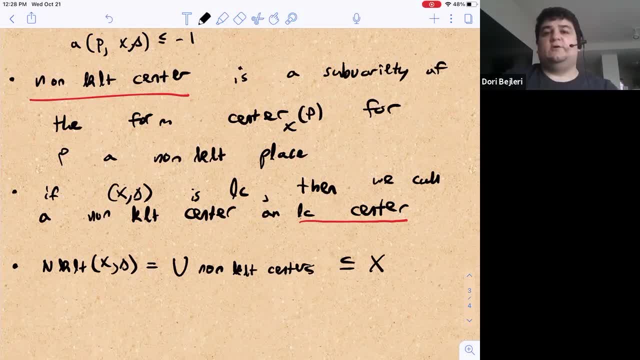 some divisor you want to understand And you need to control what it looks like on the log-canonical centers, which is where things can go wrong, And there you need to use some kind of inductive induction methods to understand those. OK. 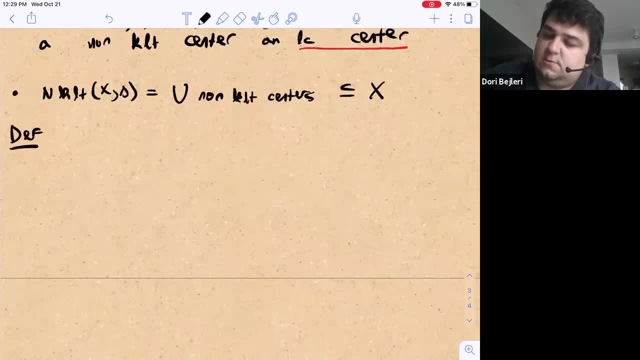 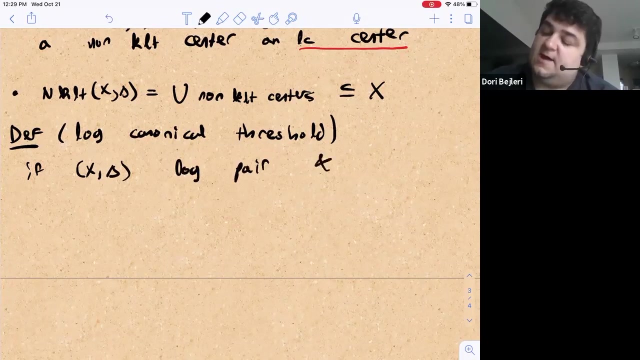 And then finally, the last definition. this is the log-canonical threshold. So we have x delta r. our log pair D is some effective q-card q-divisor, And let's suppose, Because that x delta is log-canonical, 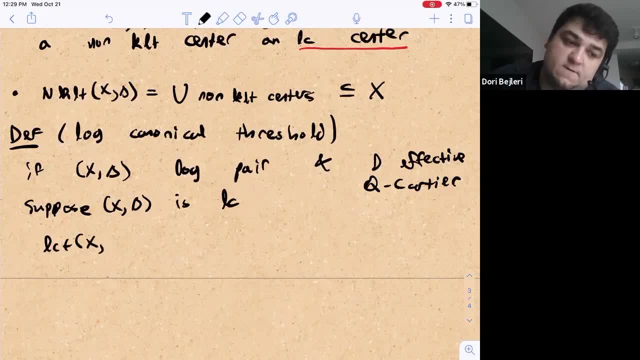 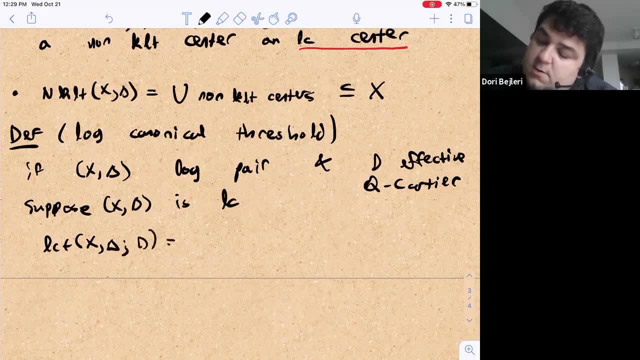 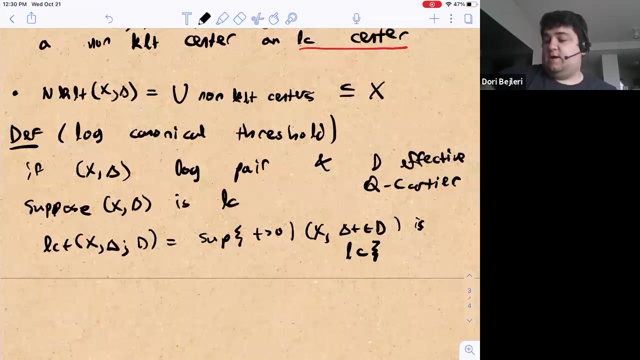 Then the log-canonical threshold of x comma delta with respect to d is the supremum of t greater than 0, such that x delta plus td is log-canonical, And by our previous continuity results we then know that for any t smaller than the threshold, 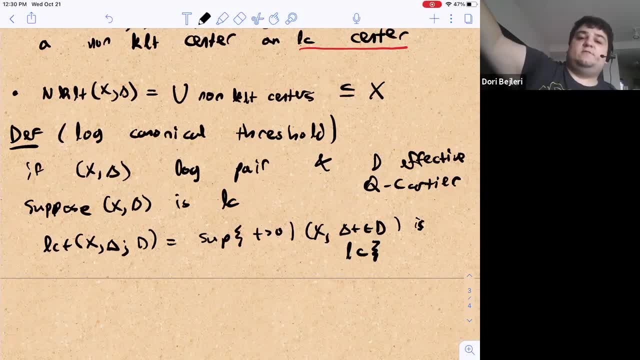 Let's say that x comma delta is KLT, for example, instead of strictly log-canonical. let's say we're in a nicer situation where it's KLT. then we'll know that for any t that has smaller than threshold, this new pair is also KLT. 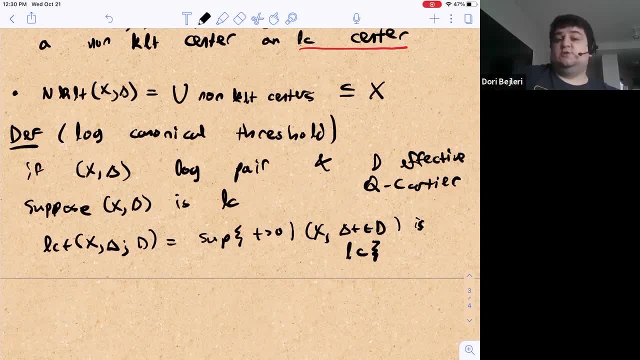 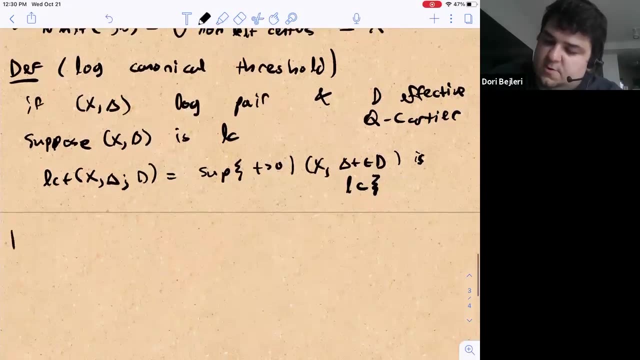 And so this kind of threshold is just where you exactly bottom end to end whatever you want to call or work on. OK, Thanks, Bye, Bye, Bye, Bye, Bye, Bye, hit this log. canonical boundary disclosure of the of the KLT locus. and here, so a couple remarks. 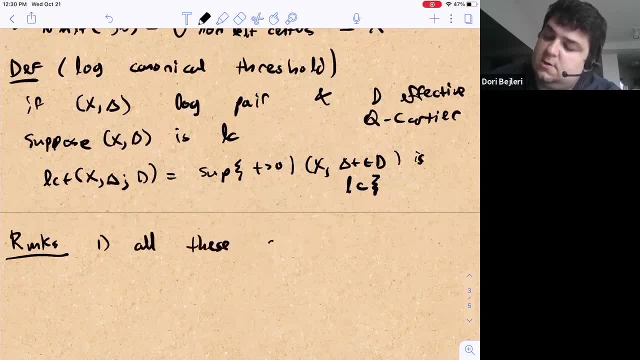 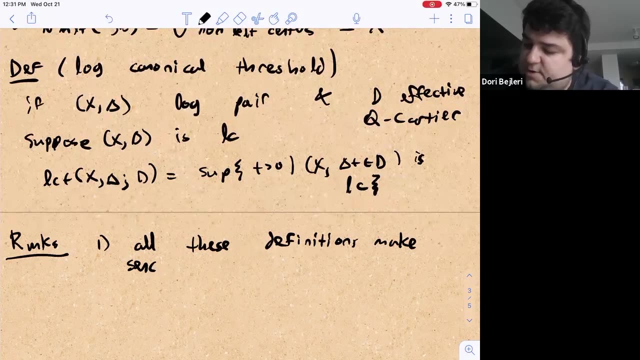 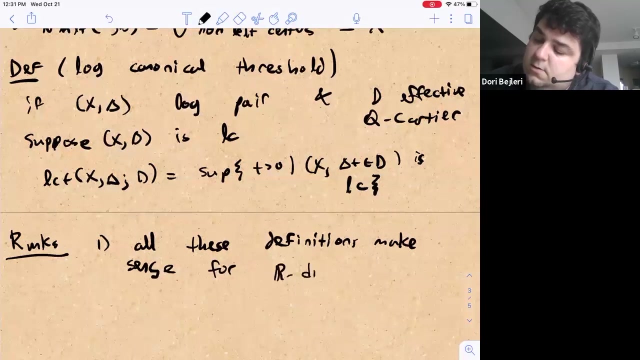 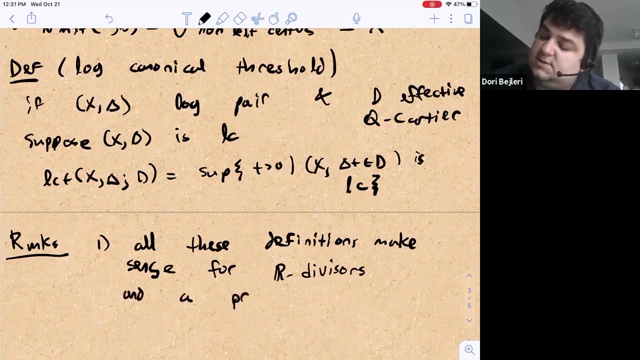 one is just that all these definitions make sense for our divisors as long as you, you assume the appropriate Cartier, our Cartier for for kx plus d and a priority. this t is just a real number, because it's the supremum of some uh, some set uh, but the. the second remark is that if 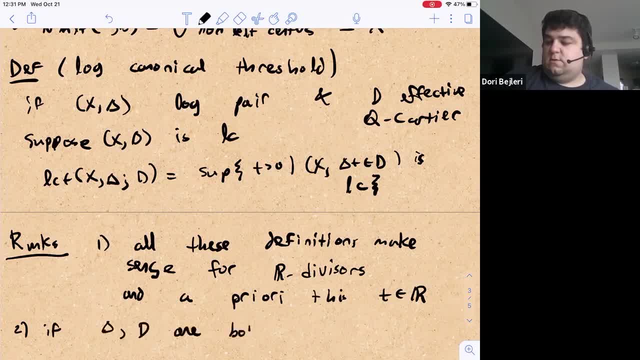 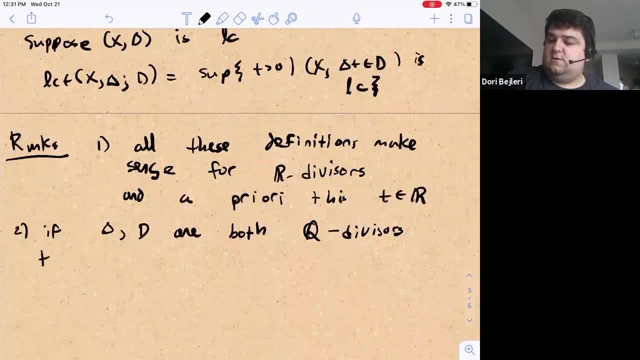 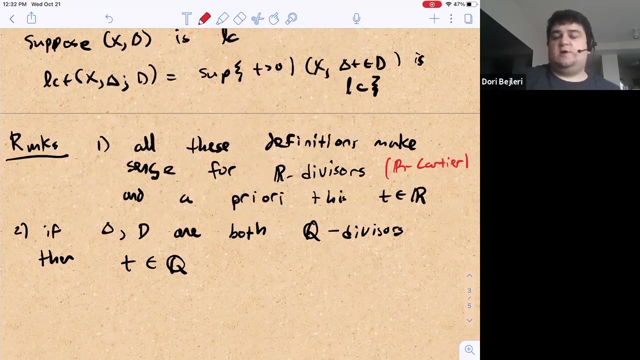 delta and d are both q divisors. uh then then t is actually rational um, and maybe I should say here again: these definitions make sense for our divisors, as long as you assume the appropriate. all the appropriate things are our Cartier. basically, anytime we had to assume something was q Cartier, assume it's our Cartier. 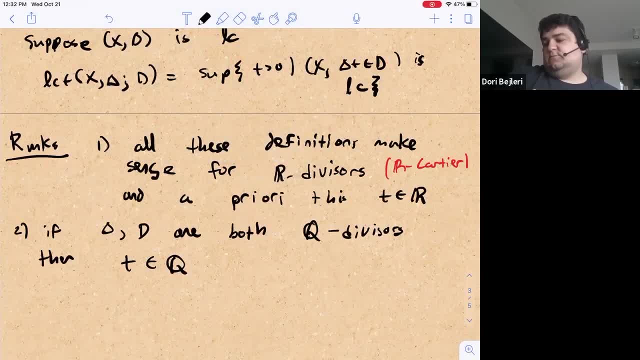 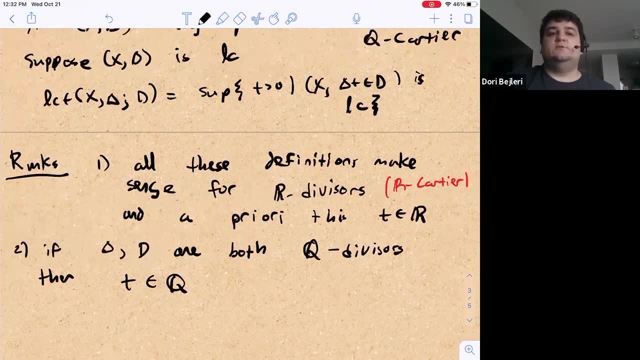 um, and, and this last part, why is this log? canonical threshold: uh, rational, if the divisors are rational, 酷 you, you can just compute it using using a resolution. so so you take a like on what you guys was. so so you write down a resolution, you compute the discrepancies and you find a form. 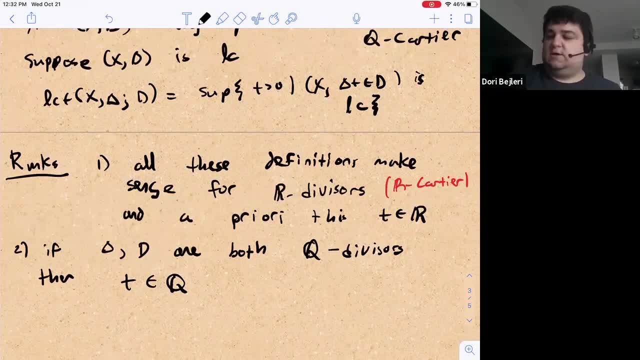 of my dear and grab a quick go around. I want to focus on both to think about that. I know I don't see you for this log canonical threshold, so I'll give that as an exercise. it's just not so easy to call the one thing um. 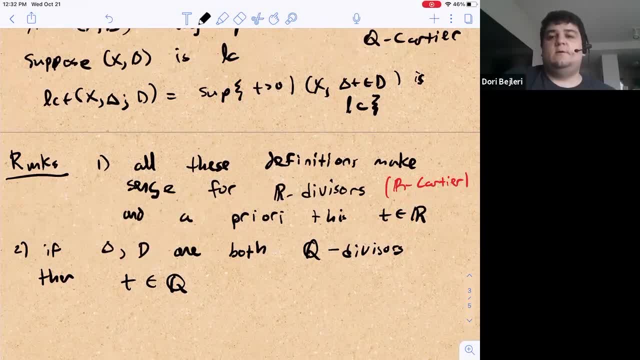 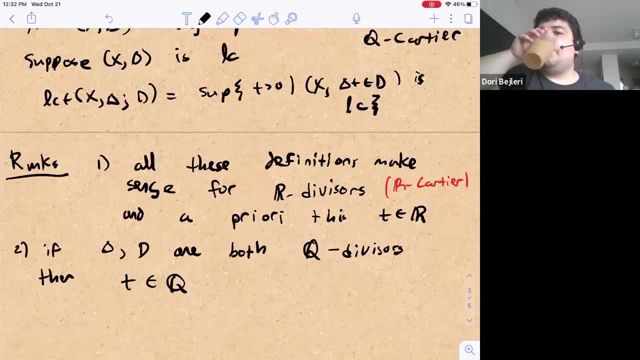 that I know that, uh, If, when you're small, rather than a fair sum of a evenings, uh, I've often been able to see if there is an 根 so that we can calculate um, ohcraft or any other basic language in value, which is also just a way of multiplying what I CATED THE LAW CONONICAL THRESHOLD. 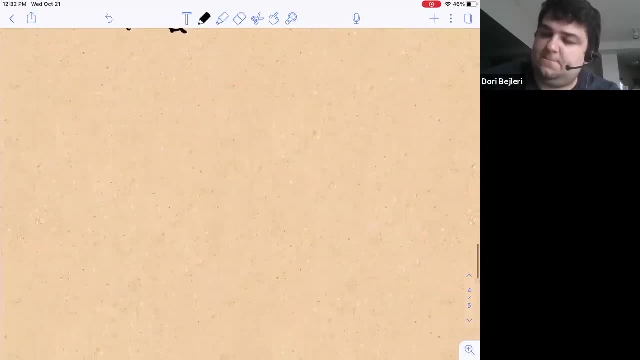 seg, such as if data can put in it's built exec. okay, let's draw some examples. so in all these examples, x will be p2, just because it's the easiest thing to draw. well, in all the examples except the last one. so let's say we have p2 comma, an irreducible. 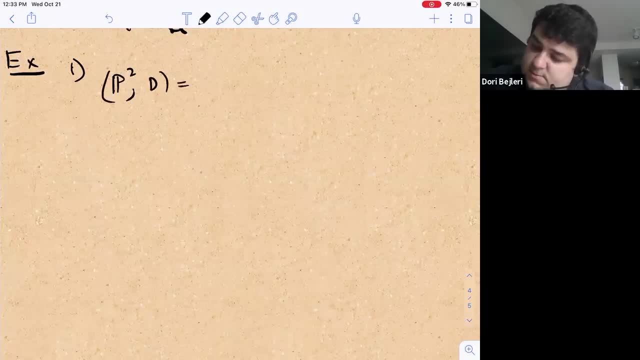 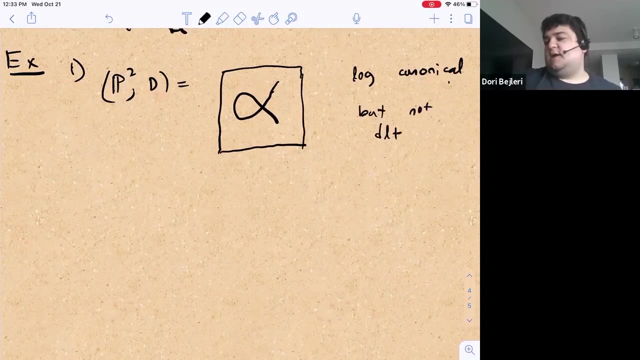 uh, nodal cubic. uh, then, and with coefficient one. so d is really this, this, uh, irreducible nodal cubic, and the coefficients are one. uh, then, this is log canonical, but it's not dlt. uh, so, to see it's log canonical? uh, well, you can take a simple, normal crossings resolution. 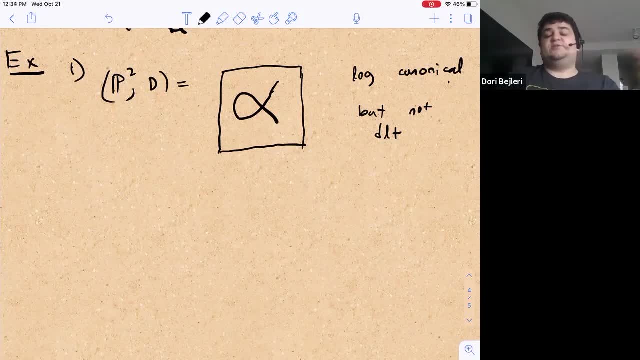 by blowing up that node point, uh, and then the discrepancy of that divisor is minus one, and everywhere else you're just have x with a smooth divisor. so any other discrepancies of any other blow ups are strictly bigger than minus one. um, but it's not dlt because there's 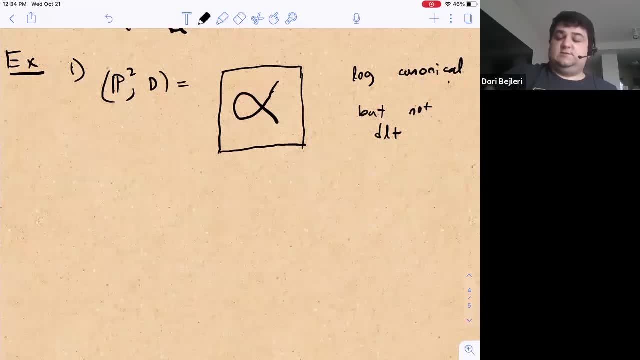 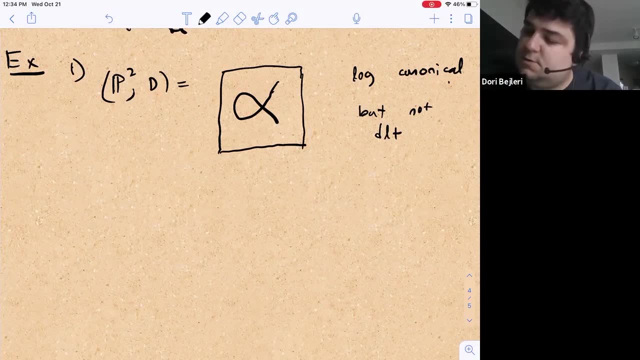 no locus where this divisor is normal crossings, because a simple normal crossing- sorry, it is normal crossings but it's not simple normal crossings because it has a self-intersection. so to see if you can get a simple normal crossing, now we can look at p2 with d1 plus d2, where 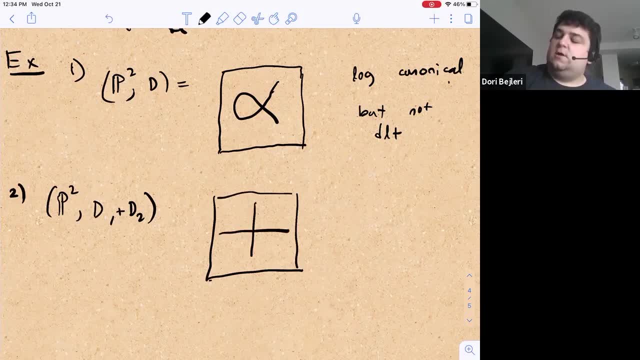 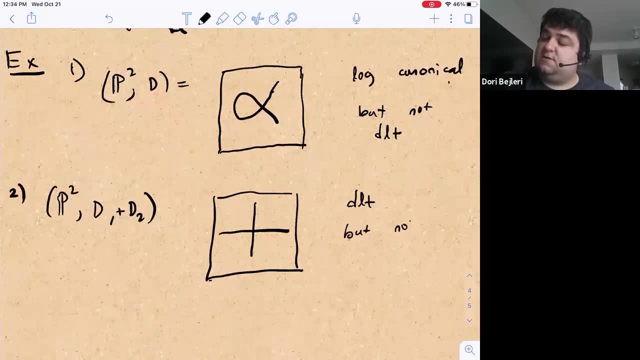 uh, d1 and d2 are the, the nodal union of just the, the axes, uh, then in this case we have something that's dlt, because it's actually simple, normal crossings, uh, but not a plt. uh, if you blow up that, that node point, then you have a discrepancy that's uh, strictly minus one. 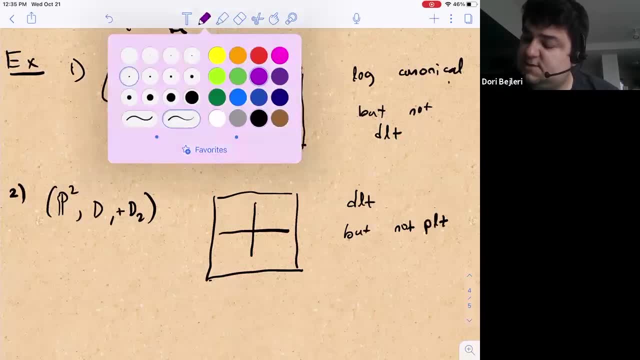 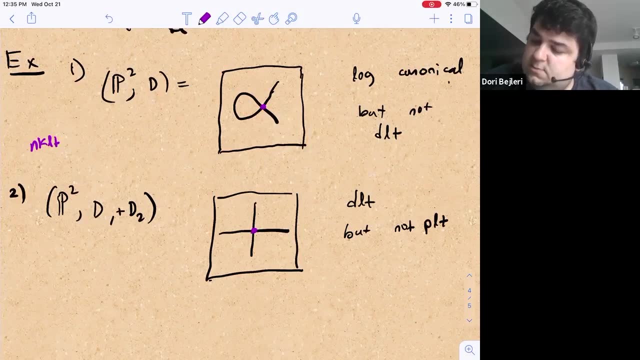 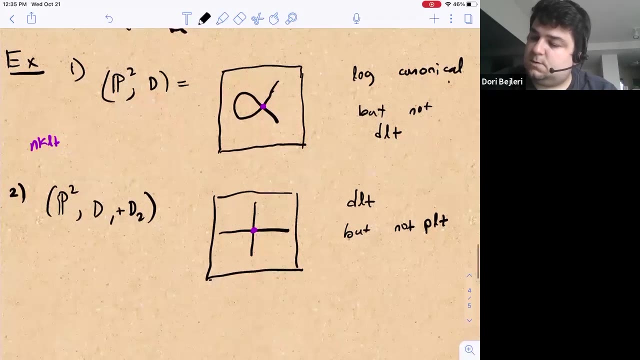 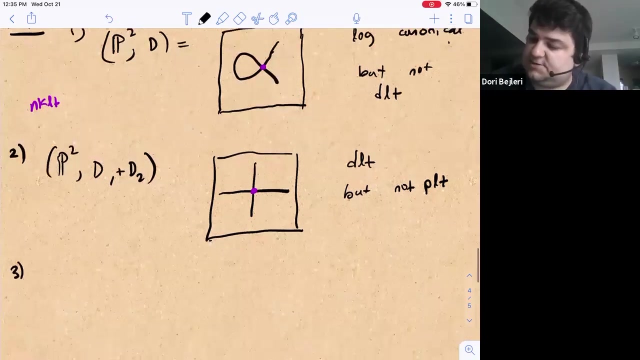 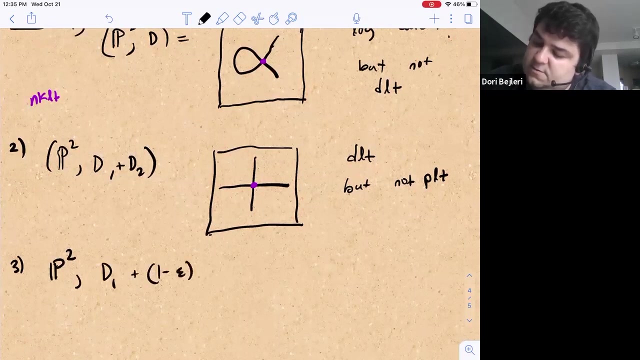 so in both these cases, the the non-klt locus is this node. we can get something that's plt by just decreasing the coefficients on on one of these divisors. so if we look at p2, comma d1 plus one minus epsilon d2, then this is plt. 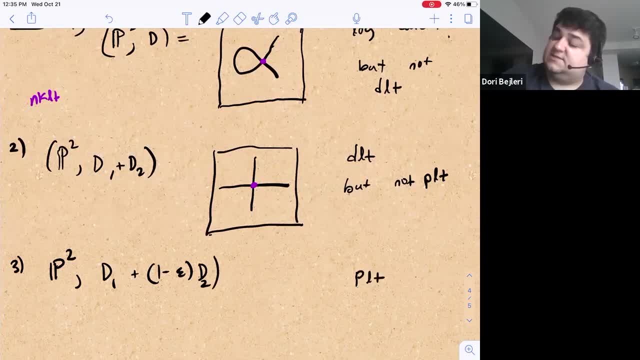 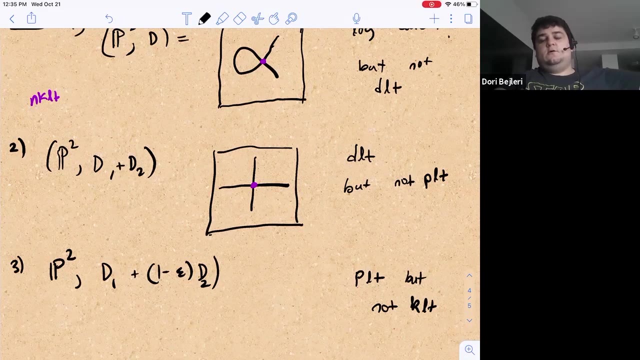 but it's not klt because there's still this divisor d1 with coefficient one, but it's plt because soon as we decrease this coefficient by epsilon, then that exceptional over that exceptional that gave us a discrepancy minus one now has a discrepancy minus one plus epsilon as soon as we decrease this. 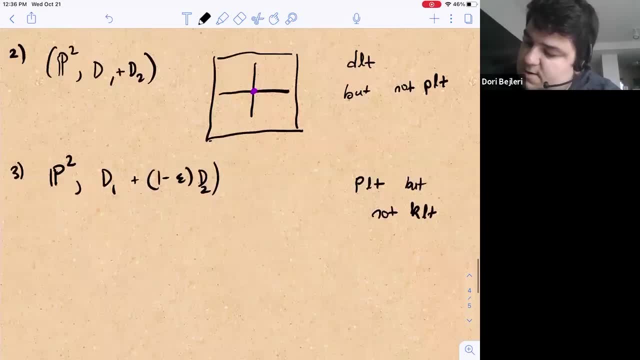 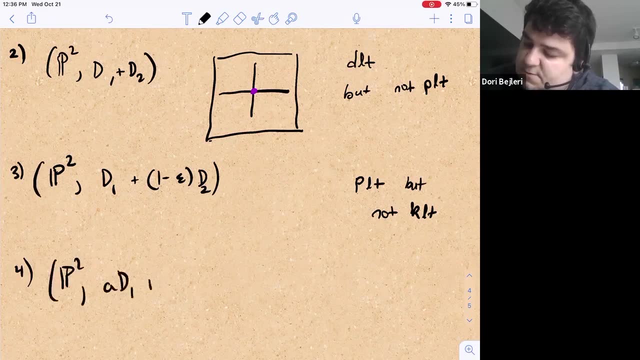 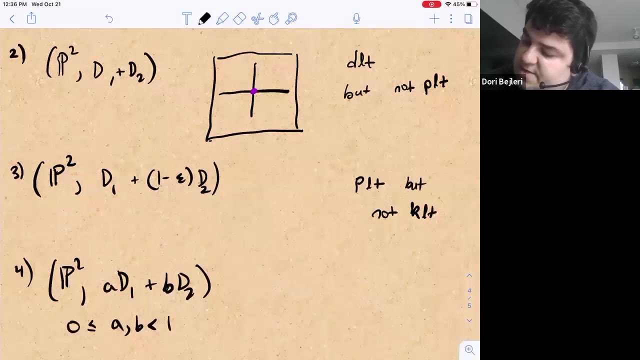 and then finally, uh, in the same same sequence, we can just look at p2, comma a, d1 plus b, d2 for a and b, both strictly smaller than one. then this is something that's klt now we have. all the discrepancies are greater than minus one and all the coefficients are smaller than. 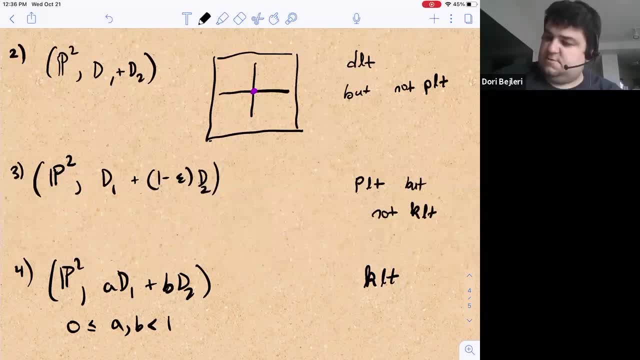 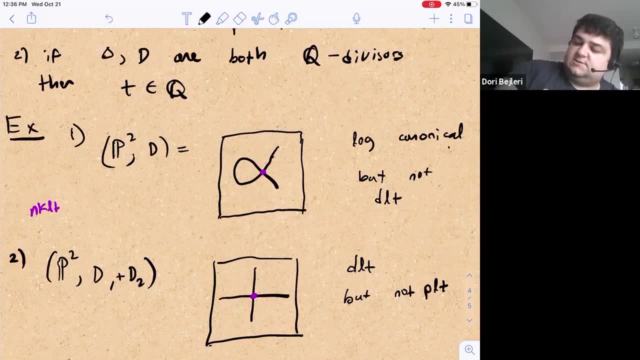 one. um. okay, so those are some kind of basic examples, but but it really the the most important takeaway is that this the dlt condition. the thing that makes it so subtle is that it's a global condition. locally. these two pictures, one and two, look exactly the same. 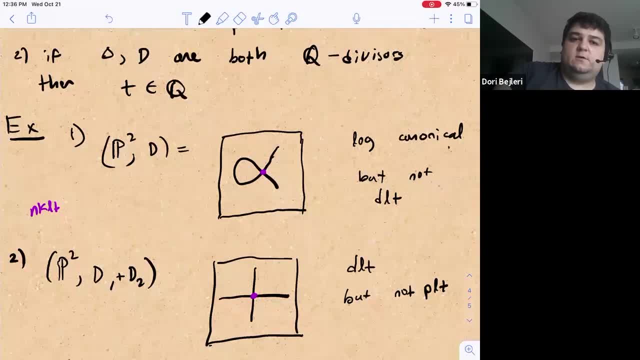 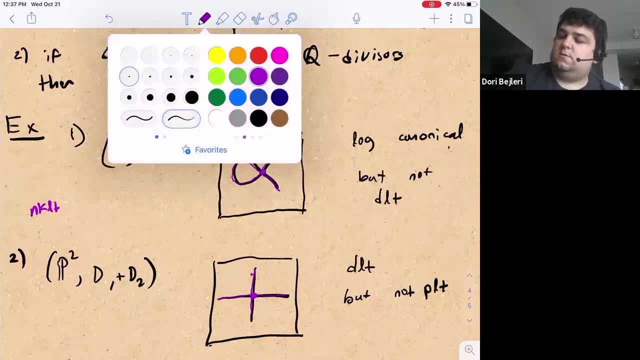 locally around around the, the non-klt center, um, oh, also i should say here the, in these cases, actually, the non-klt center is this whole, i guess the whole thing, because it has coefficient one, um, but anyway, uh, so right, so so this dlt condition. the thing that makes it subtle is that it's a. 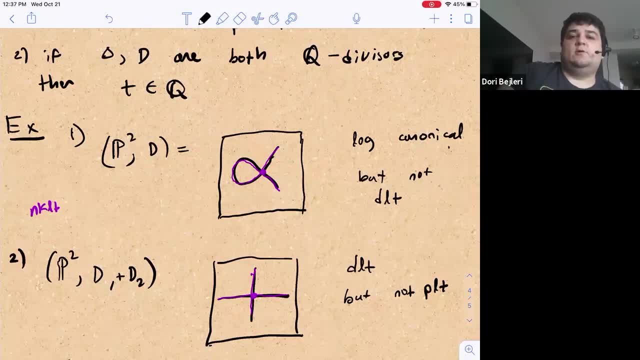 global condition. so it's a global condition, so it's a global condition, so it's a global condition, while all the other discrepancy conditions are really local. they're really local around each of the centers of each divisor. they're a condition that says: at every non-klt thing, um. 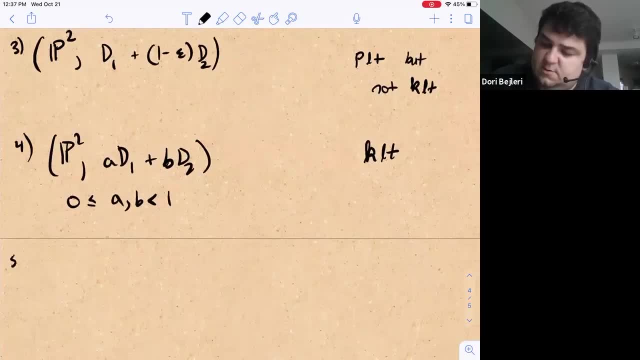 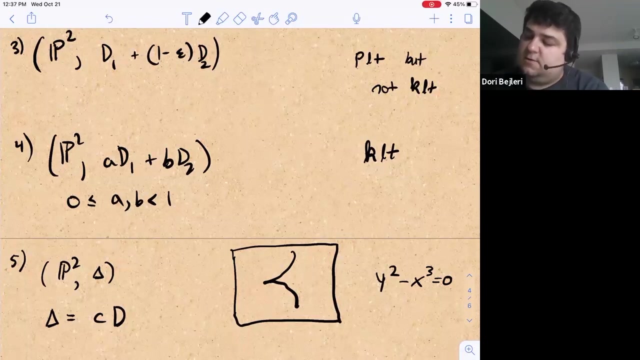 okay, um, okay, more interesting example: uh, let's look at p2 comma, delta, where delta is some constant times the cuspidal cubic um, and now we can try to compute: when is this klt, when is it log canonical um? and so to do that, we write down a resolution, so i claim that there's a resolution. 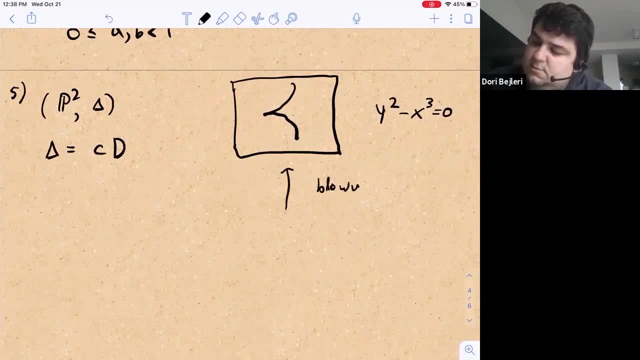 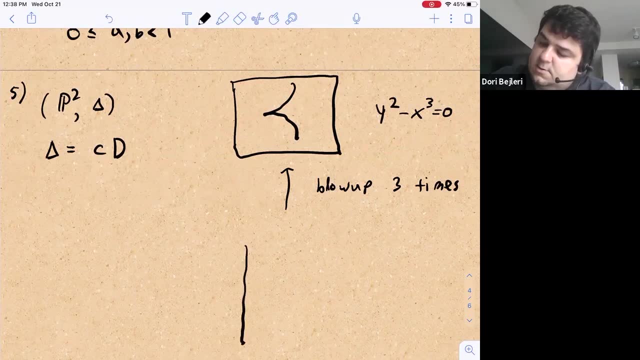 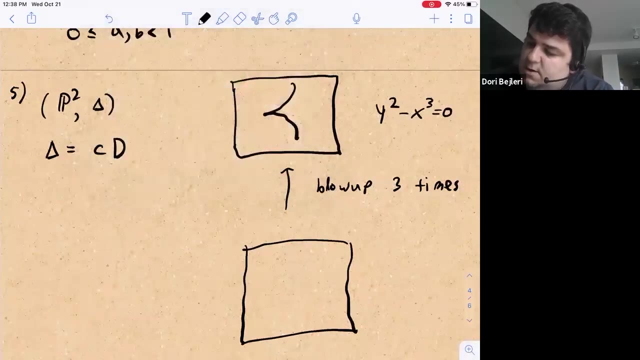 if you blow up three times uh, then we get a log resolution where, uh, the picture looks as follows: so we have a component corresponding to our d, and then we have a bunch of exceptional components, one we'll call e1, and then some other exceptional components like this: 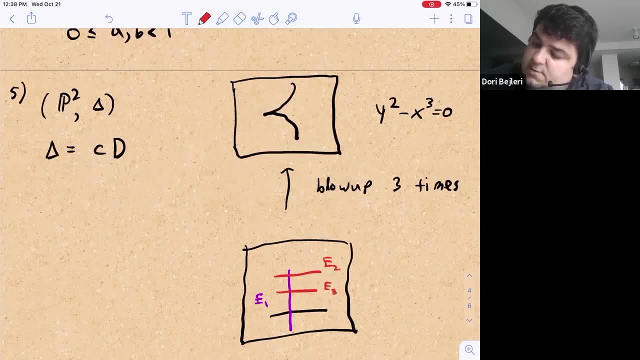 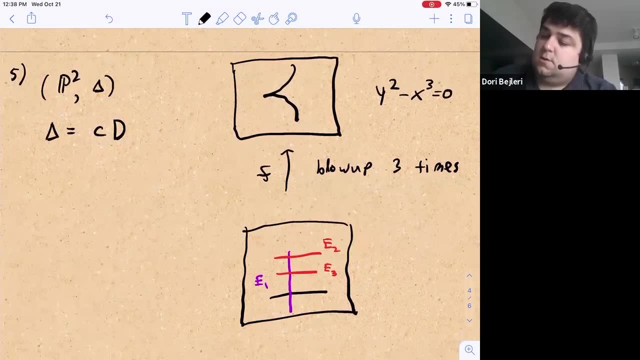 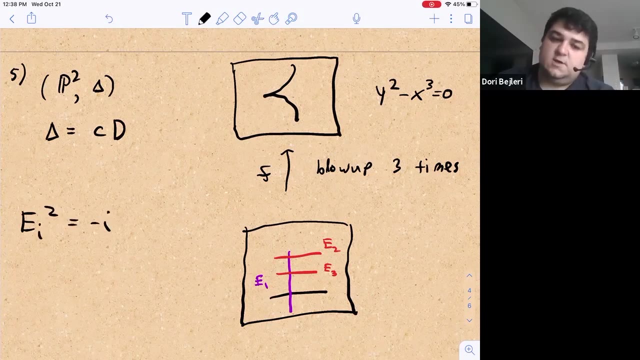 e1, e2 and e3, and now ei squared is minus i. we compute that from these three, three blowups, and then we compute that f, upper star of d is the strict transform plus two e3, and then we compute that f, upper star of d. 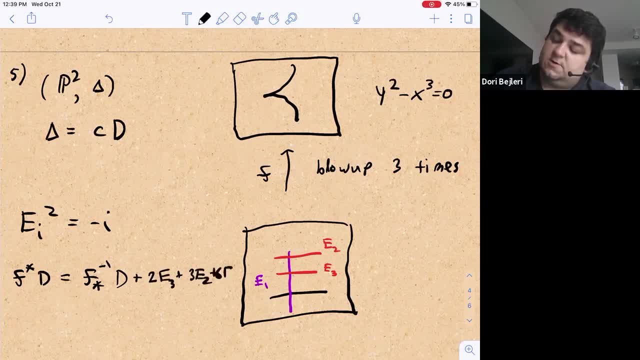 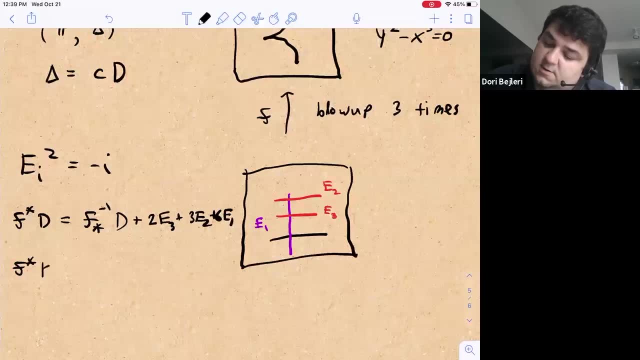 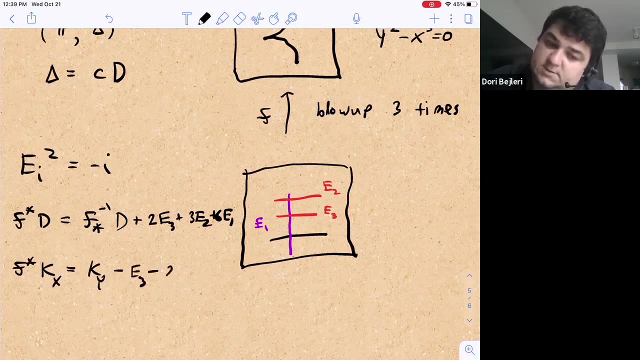 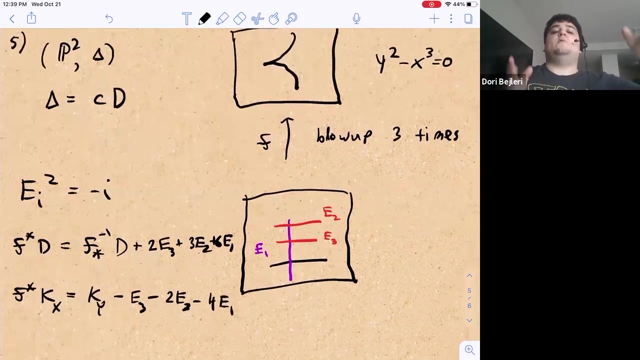 plus plus 3 e2 plus 6 e1. so those, those are the multiplicities. and then f, upper star, k is ky minus e3, minus 2 e2 and minus 4 e1. and again, this is from using the, the formula that when you blow up once, you have to subtract one copy of the exceptional. but then when you pull, 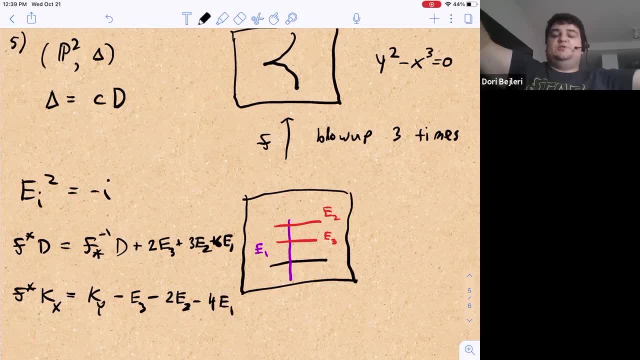 back again. you have to subtract another copy of the exceptional plus some contribution coming from the first copy that you subtracted, because these blow-ups are all kind of on exceptional, on exceptionals, and so putting this all together, we get that. i'm going to write it in the log form. 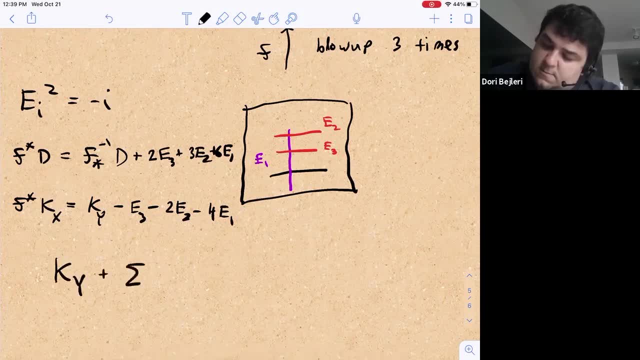 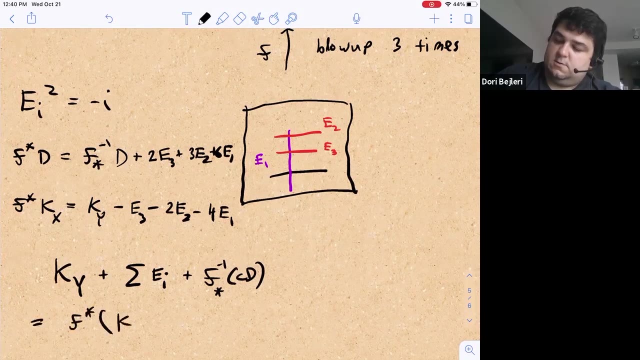 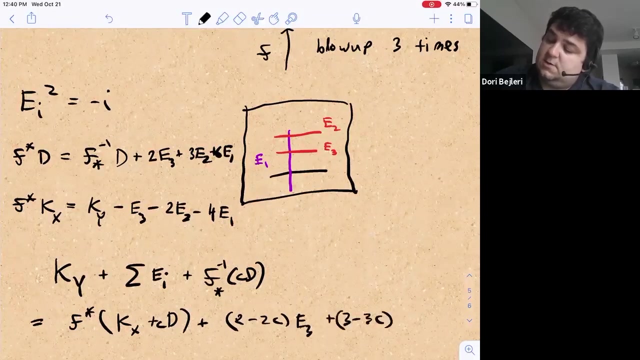 rather than the regular discrepancy form, that this uh log canonical divisor is equal to the pullback plus the following coefficients: we have 2 minus 2c times e3 plus 3 minus 3c times e2 plus 5 minus 6c times e1. 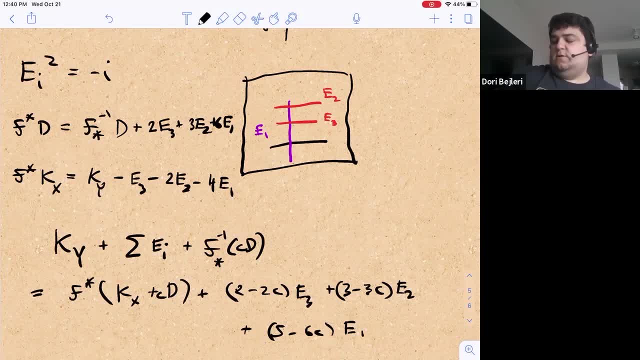 um, and the reason i wrote it this way in the log form, with log discrepancies, is just because, uh, i find it easier to compute this way, because you write it this way, and then you can solve for the, the coefficient on the other side by using a junction, by kind of smashing each side with ei and using the fact that. 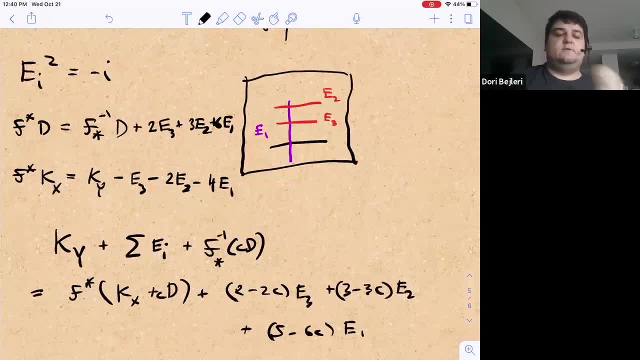 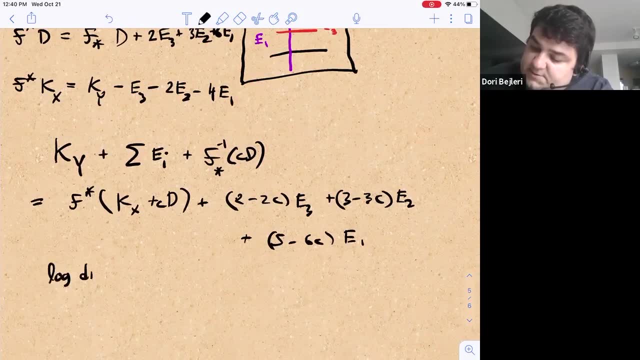 ky plus eiei is the canonical of the uh um, and so what this tells us is that uh. so, with log discrepancies, we need the log discrepancy to be greater than zero or ourage, or greater than or equal to 0 for KLT and log-canonical. 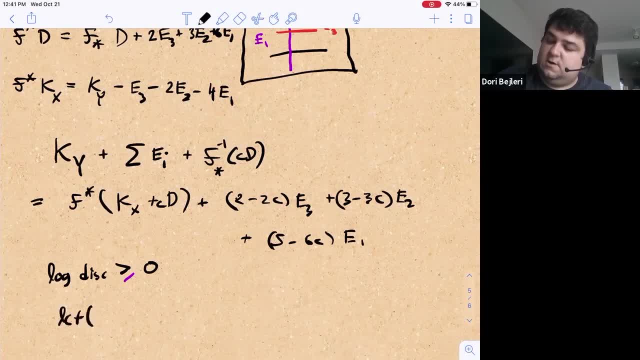 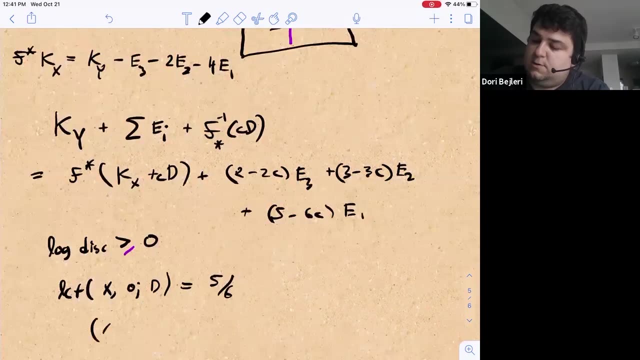 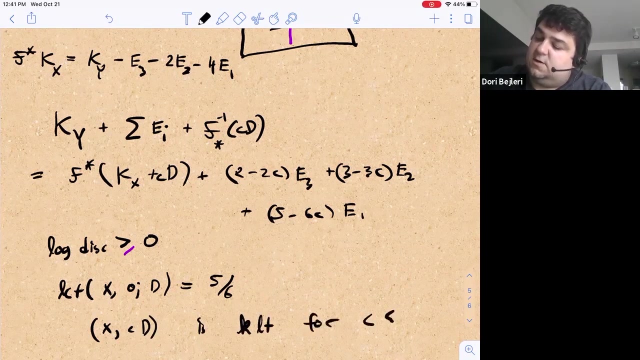 And so this tells us that the log-canonical threshold of P2, with no boundary relative to this cusp, is 5, 6, because that's when the log discrepancy becomes 0, or the usual discrepancy becomes a minus 1, and that the pair x comma CD is KLT for any C strictly smaller. 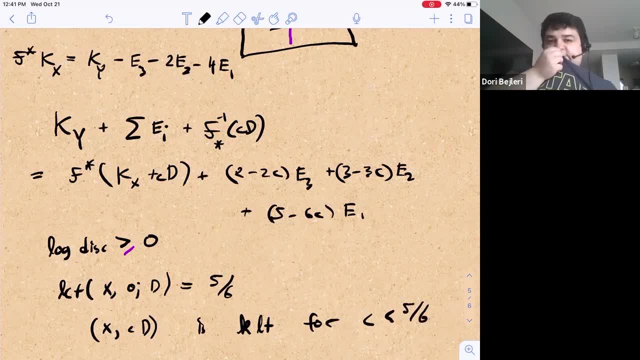 than 5, 6.. And so we see here, the cusp is a more complicated singularity than a node, and so it has a smaller log-canonical threshold and a smaller range where it's KLT, The more singular the divisor gets. 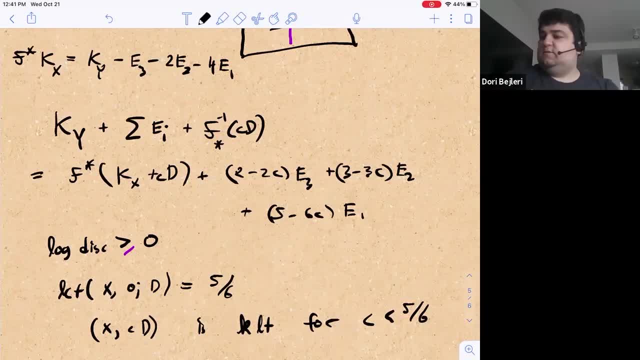 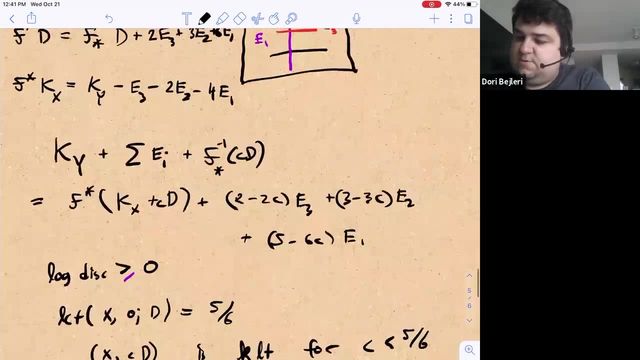 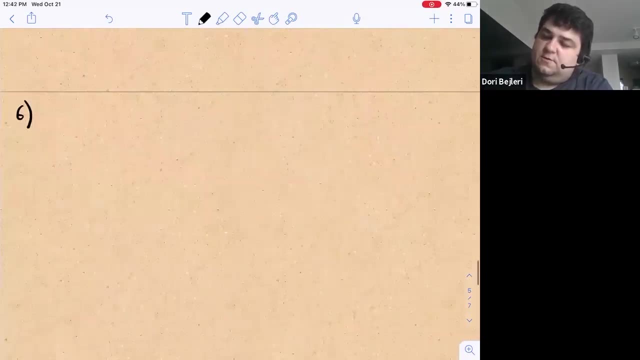 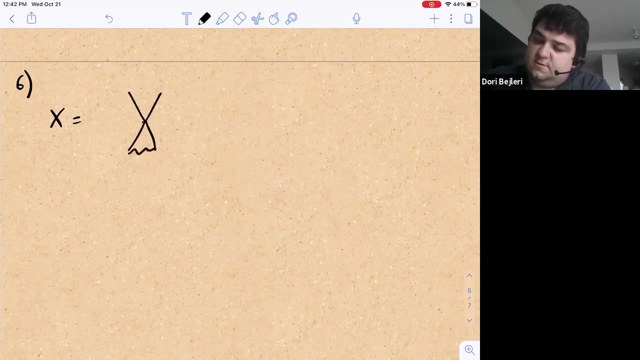 the smaller coefficient, you need to make it KLT. And then one more example: This was 5.. One more example where we're not on P2.. Let's say that x is this cone over a rational normal curve which we discussed a few classes ago. 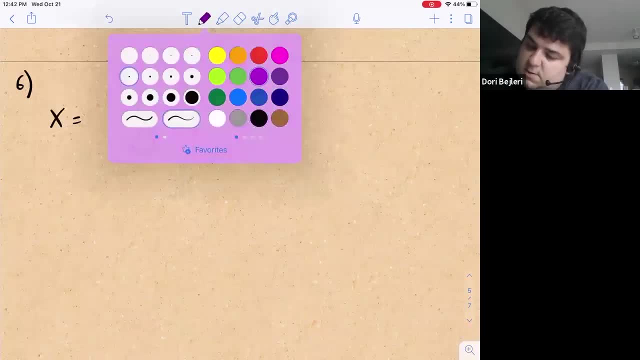 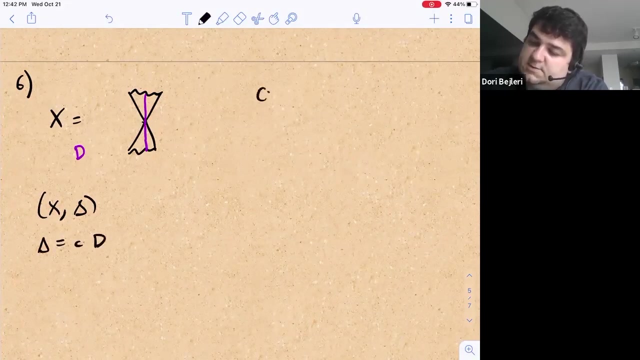 and let's say that d is one of the lines through the cone point, And so we're looking at the pair x comma, delta and 1.. Where delta equals CD, this is the cone over degree n, rational normal curve. It has a resolution that's like this: total space of the line bundle O minus N. 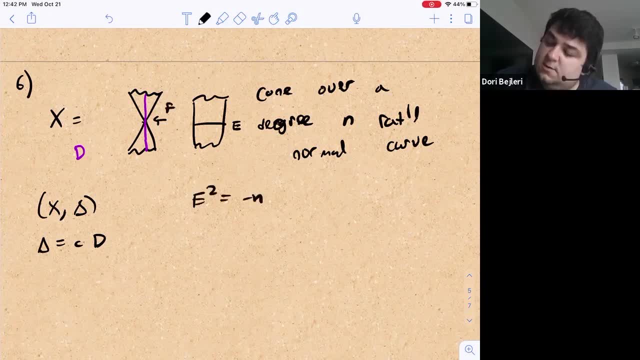 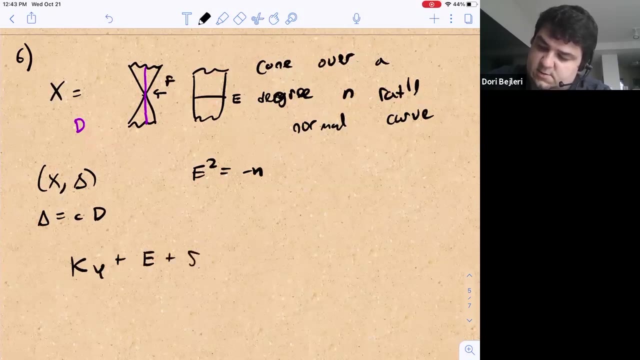 And so E squared is minus N and then using that in a junction you can just compute. I won't write down all the all the various steps, I'll just write down the final computation. So we get the ky plus E plus strict transform of delta is f upper star. 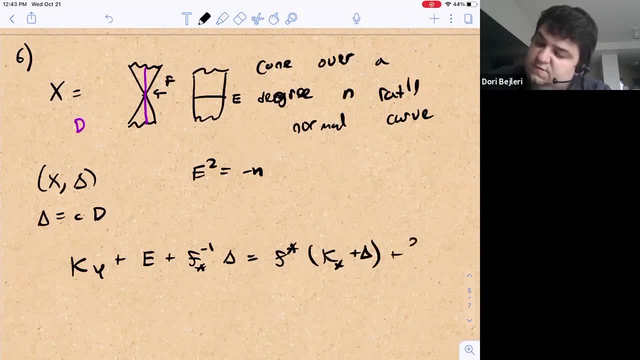 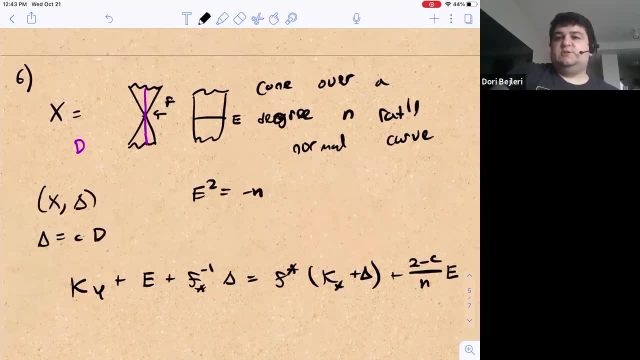 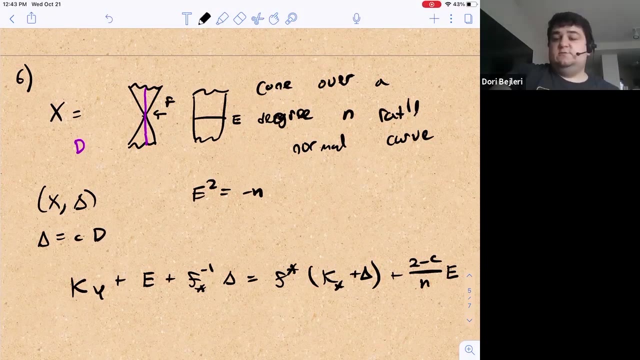 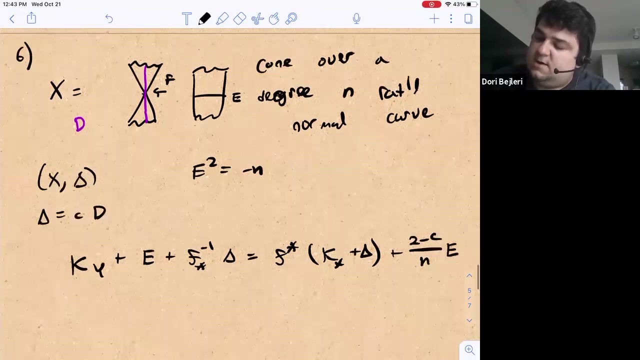 kx plus delta plus two minus C over N, E And this two. it comes from a junction. The way we're going to compute this coefficient is by using that E as a rational curve. So ky plus E, dot E is two, is minus two. So that's where this two comes from. The N comes from the E squared minus N. The C comes from the coefficient on D and 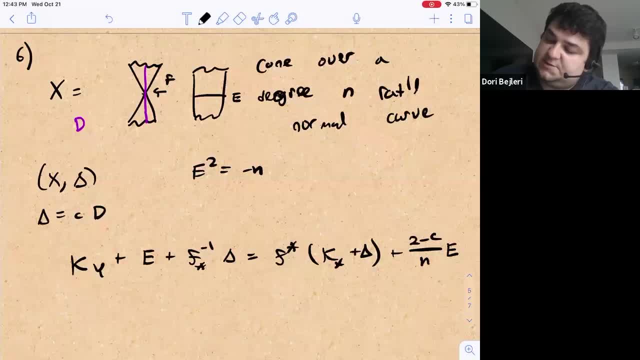 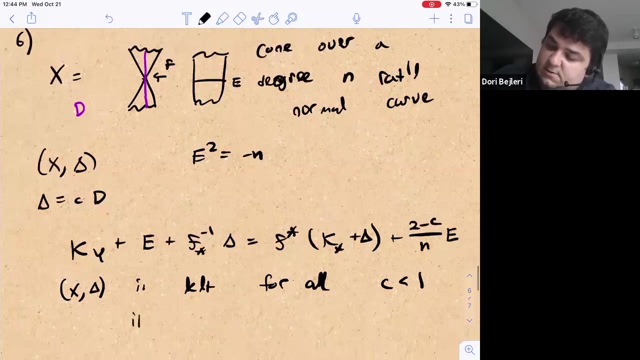 Yeah, so it's the upshot here. The upshot is that actually, X comma delta Is KLT For all C less than one. So of course C needs to be less than one for the round down condition. and this, this discrepancy, this two minus C over N is always going to be strictly smaller than one as long as C is is less than or equal to one, In fact. and so it's, it's KLT for all C less than one. and then it's 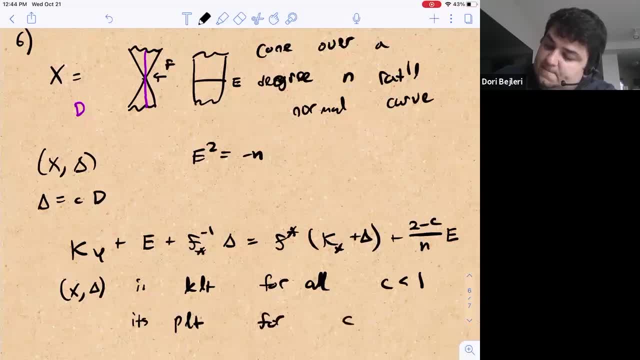 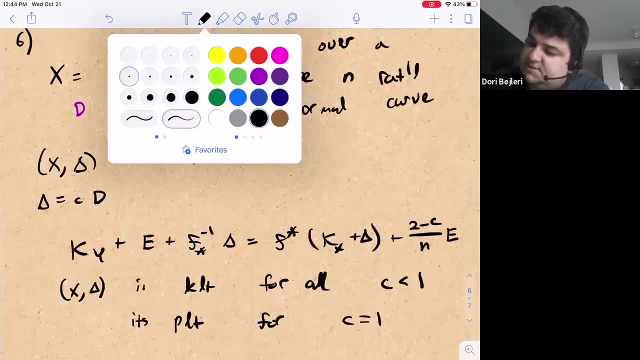 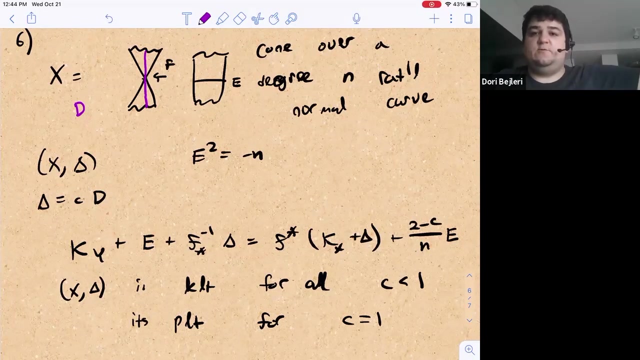 PLT For C equals to one, Because that C equals to one, the discrepancy is still. It's still Bigger. the log discrepancy is still bigger than zero, or the discrepancy is bigger than minus one. And so this gives us an example of something that's that's PLT at the log canonical threshold. So as soon as you go above one, you're not even log canonical anymore, because you have this divisor with large coefficient, but at the log canonical threshold it's actually still just PLT. 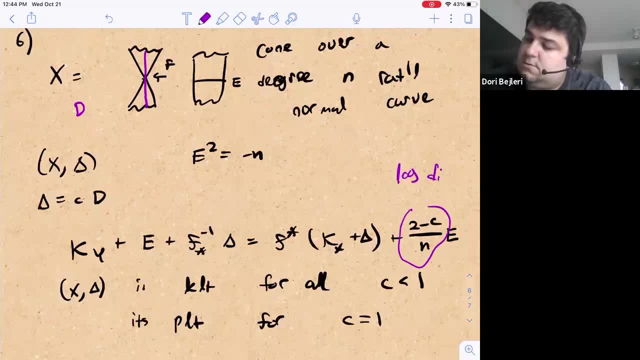 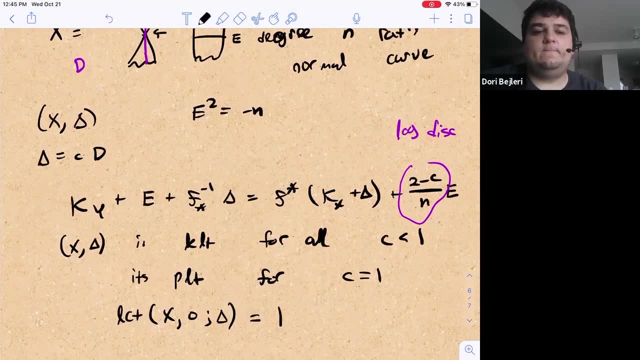 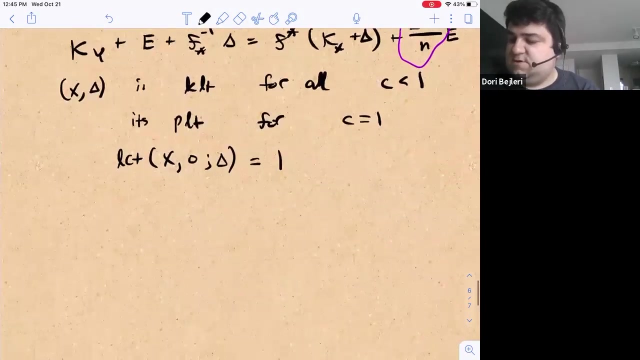 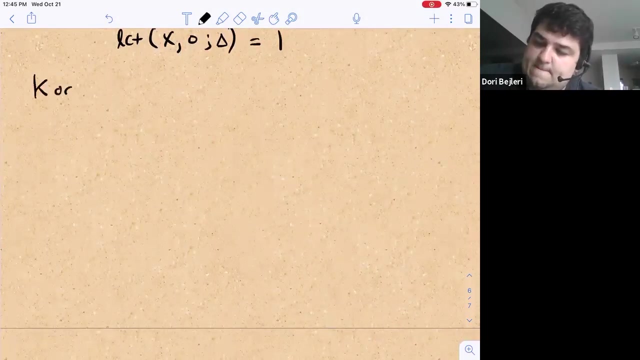 Let's say this: Okay, Next we're going to move on to vanishing theorems. So, So our next goal is to prove a sequence of stronger and stronger vanishing theorems, starting with the Kodair vanishing theorem. 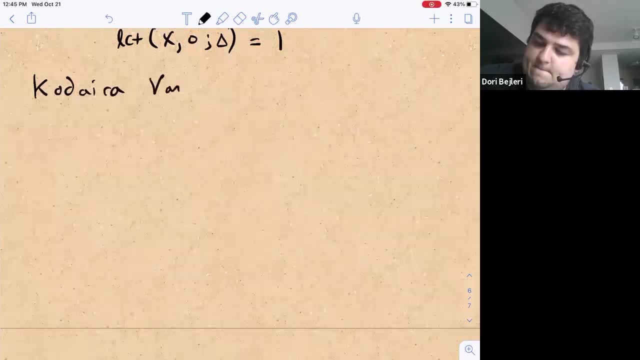 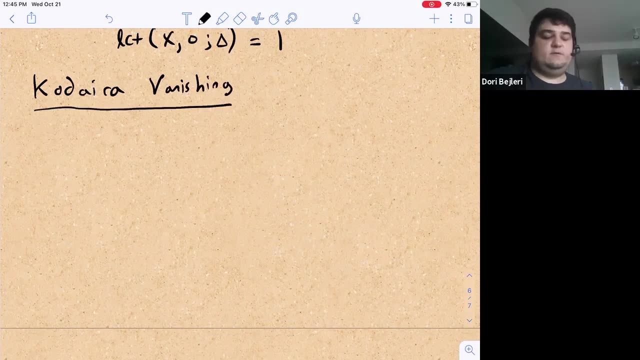 So, So And all So, in the end we want to prove at least a vanishing theorem for KLT pairs. But all of these different vanishing theorems reduced to, to the smooth case and reduce the Kodair vanishing theorem. 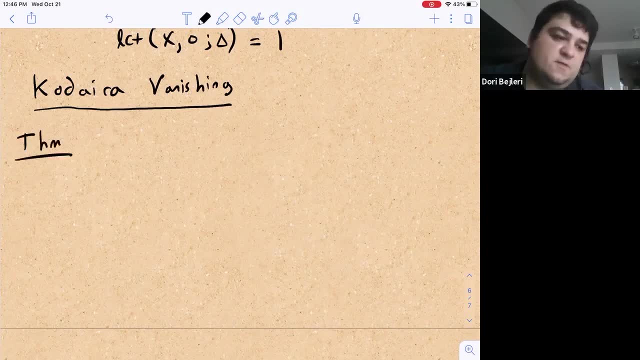 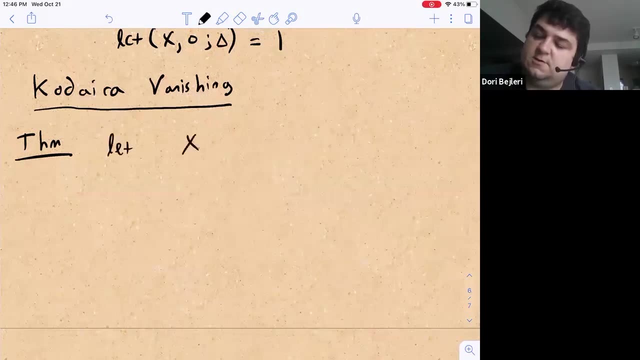 So we'll start there. So the theorem says that, and I think this came up in the surfaces portion, where we just use it without proof. But I'll recap the theorem. So let X be smooth projective. And here I'm really going to. even though I said the whole class is over the complex numbers, I really want to emphasize that this is over the complex numbers. 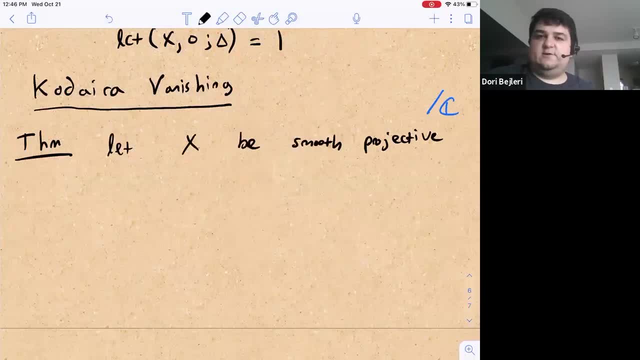 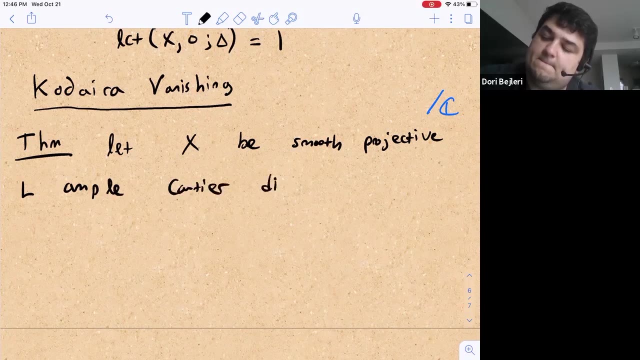 Though other characteristic zero fields are okay by standard reductions to the complex numbers. but the proof is really a complex thing. Um, And let's say L is an ample Cartier divisor, Then The cohomology of X with coefficients in KX plus L is zero for all I greater than zero. 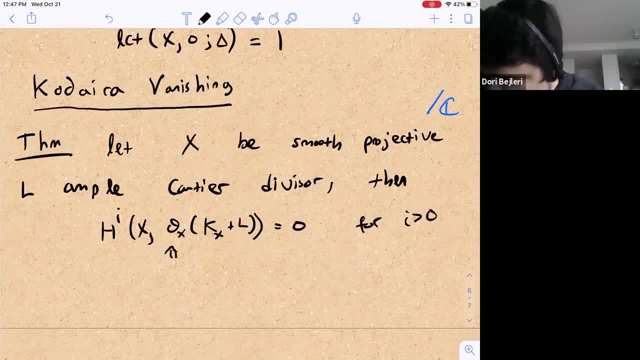 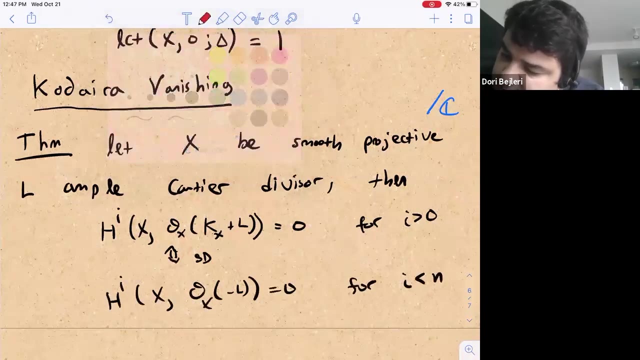 Um, or If we can, just, If we can just say that. So then, If we can just stare dually, We could say that the cohomology Of X with coefficients in ox of minus L, Zero, For I, strictly less than N. 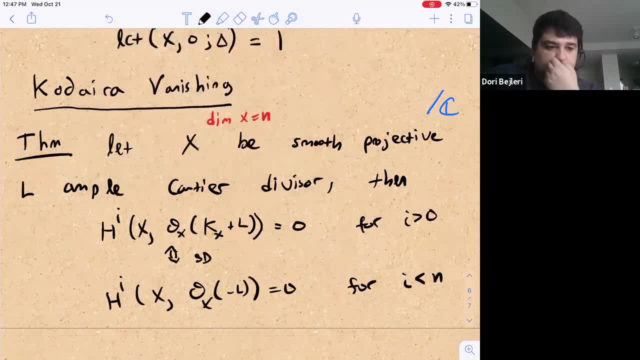 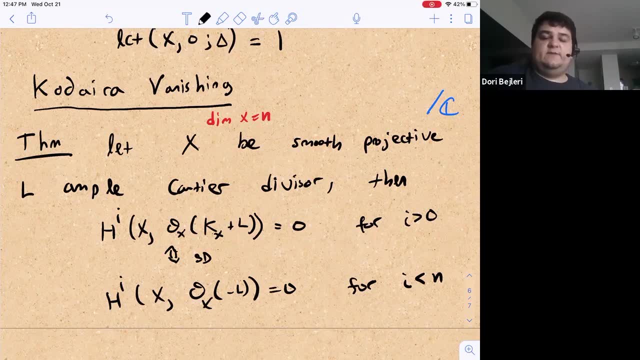 Where N is the dimension. So throughout all these proofs, we'll use N for the dimension of X. Um, So when L is actually our delta, our boundary for some log-canonical pair, then we call it the log-canonical divisor. 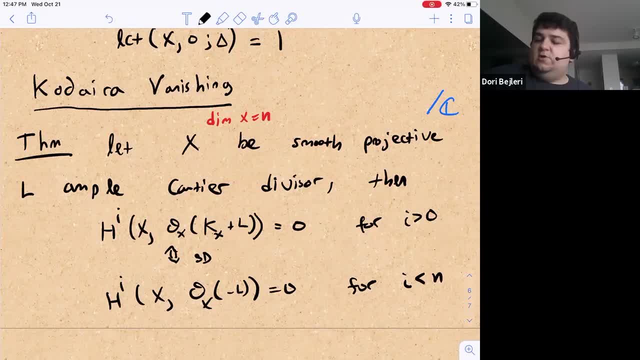 But more generally, when you just have this L and you're looking at cohomology of kx plus L, these are often called adjoint divisors And because they appear so frequently in these vanishing theorems, they have a name. 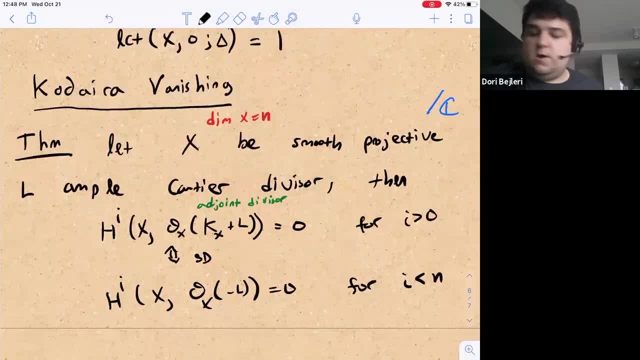 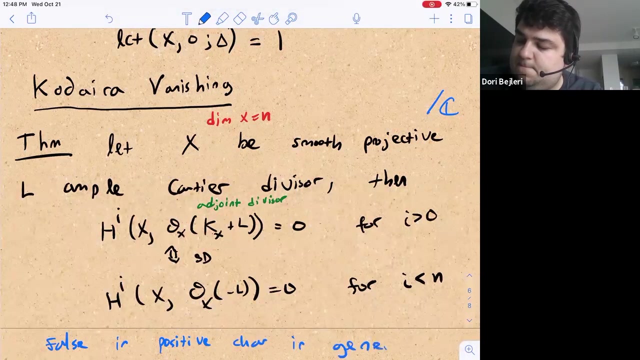 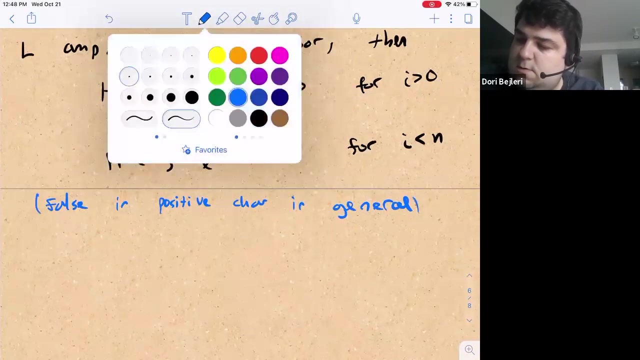 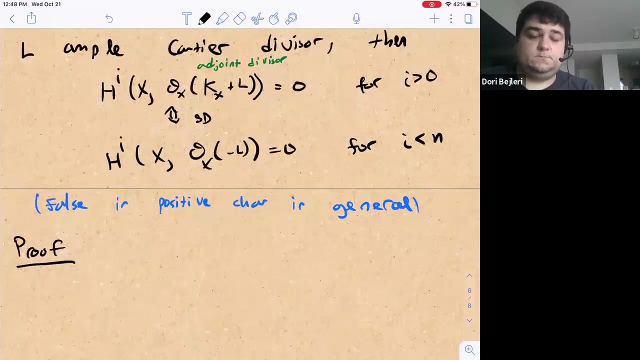 Or adjoint linear series. OK, so let's just start with the proof, but with the remark that this is actually: not only do we really need to use C in the proof, but this theorem is actually false in positive characteristic. OK, so the first step is: well, we'll. 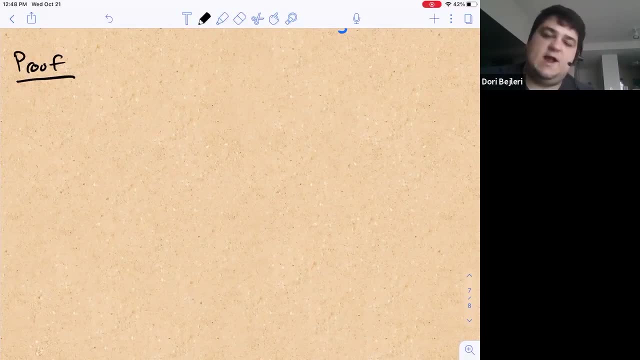 do it for the slightly easier case where L itself is actually an effective ample divisor. So L is just some ample divisor, but not necessarily effective. Let's assume that L is some smooth, effective divisor. Then we go back to the proof for this. 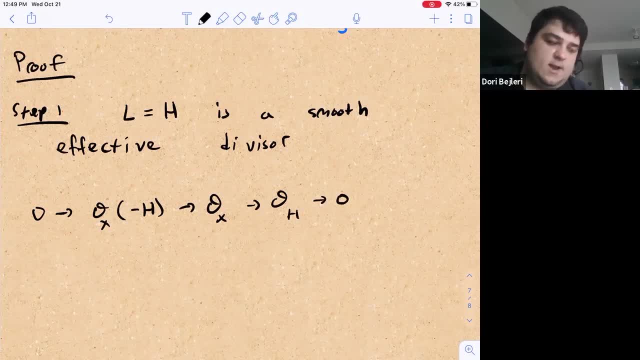 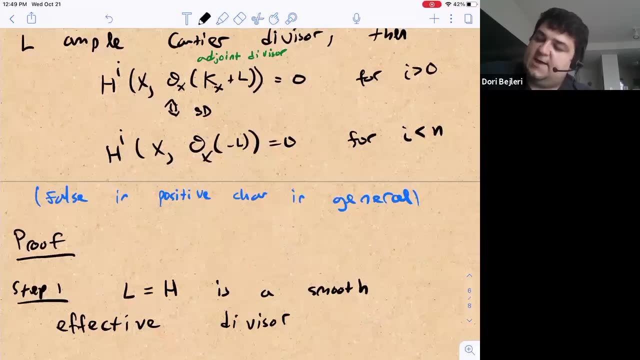 So in this case we have this standard ideal sequence, And so we're going to prove the Sear-Duell version, where we want to show that h, i is zero for all i less than the dimension. So we'll take cohomology. What do we get? 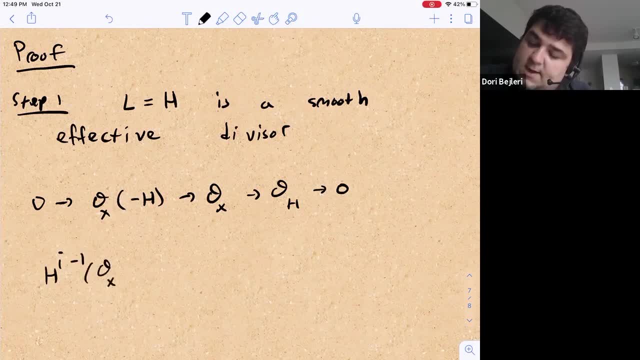 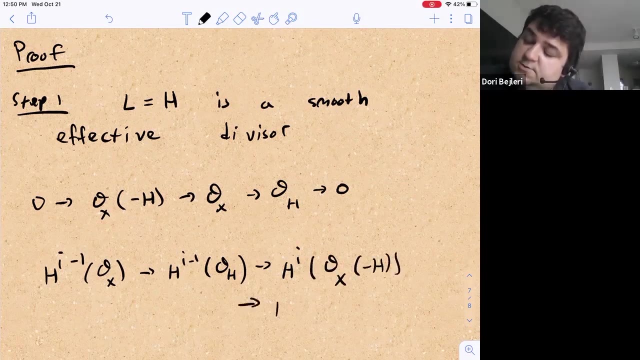 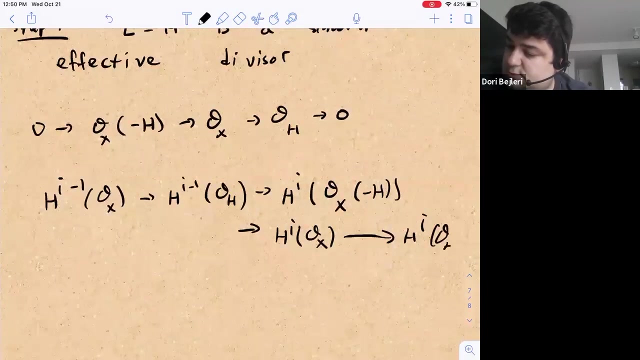 We get h? i minus one o x maps to h? i minus one o h, maps to h? i of. the thing we want to show is zero In that range goes to h? i o x and goes to h? i of o h. And these maps, what are they? They're restriction maps. 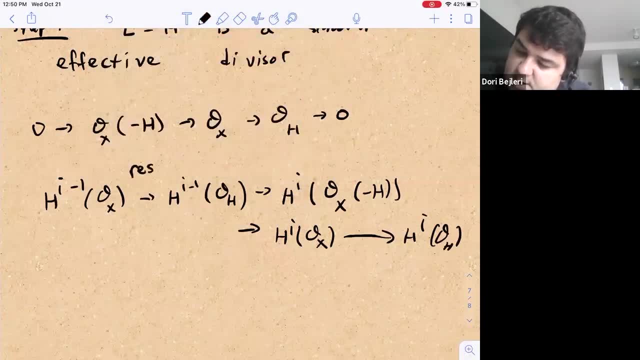 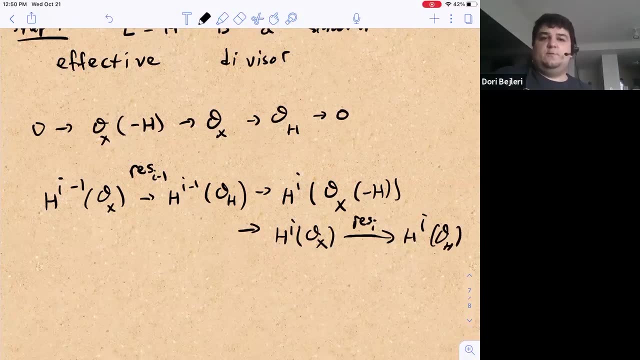 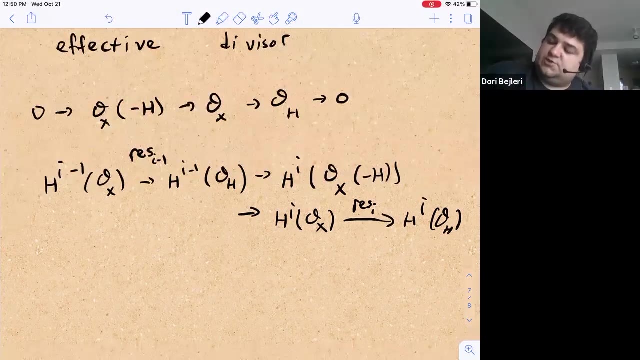 So let me just call them restriction i minus one and restriction i. They're the maps on cohomology coming from restricting the structure sheaf from x to h. So what do we want to show? We want to show that all these maps, all these restriction maps, are isomorphisms, except possibly at dimension n minus one, where it's okay to be injective because we're only proving the vanishing. for i, strictly less than n. 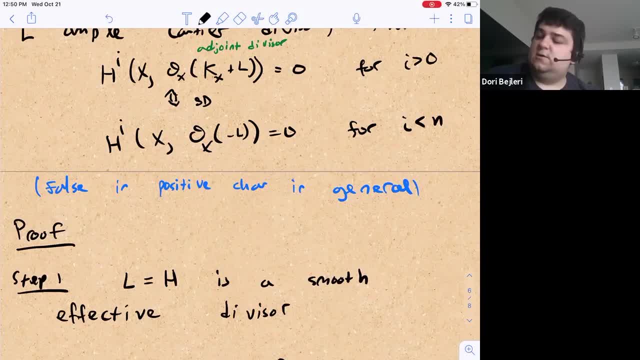 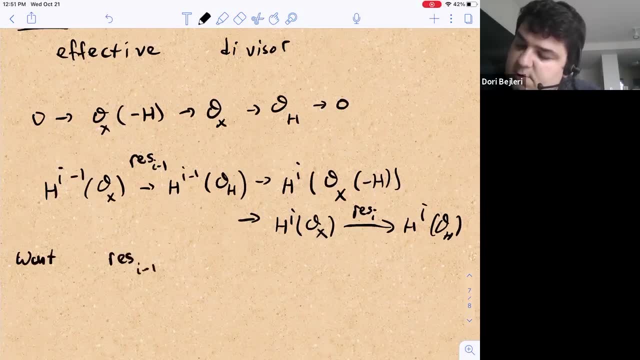 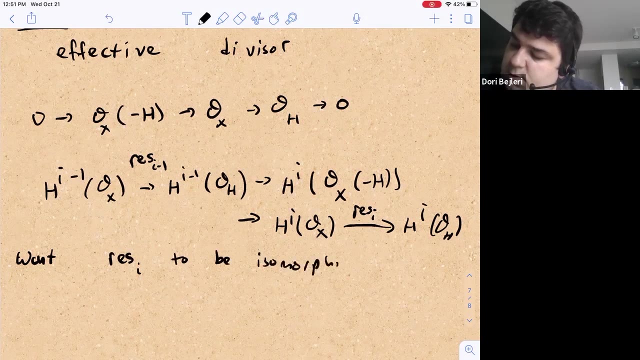 We don't care about the vanishing. I mean, the vanishing just isn't true when i is equal to n. So we want the restrictions to be isomorphisms. So we want the restrictions to be isomorphisms for i strictly less than n minus one, and injective for i equal minus one. 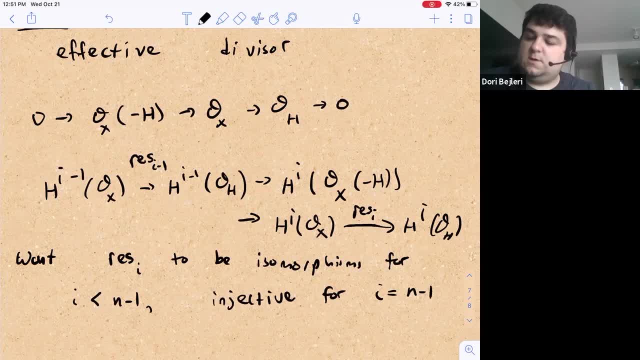 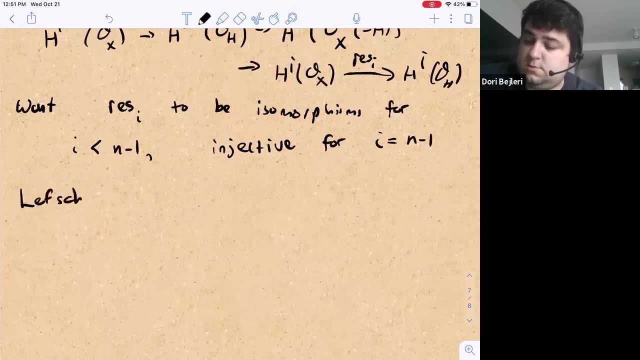 That's equivalent to the statement that we're trying to prove in this case, And this is essentially the statement of the Lefschetz hyperplane theorem, And so this is where we're really using that. we're over the complex numbers And so we have topology. 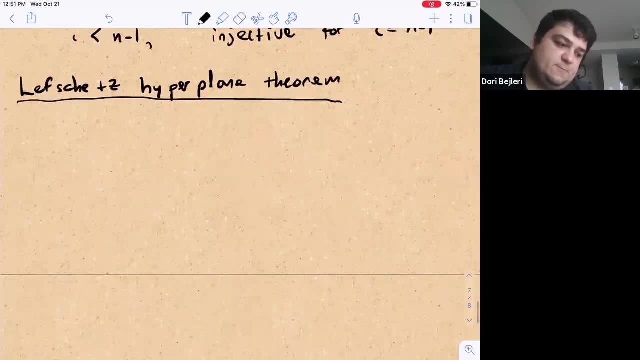 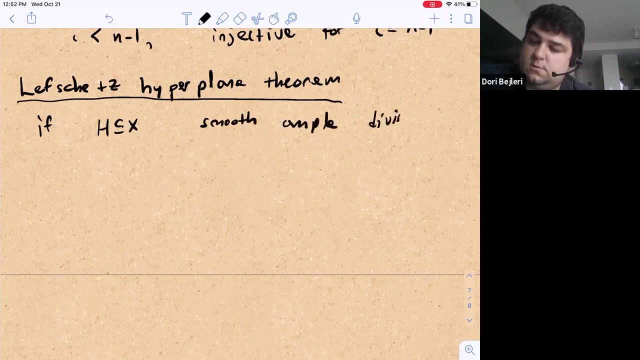 So the usual form of Lefschetz hyperplane tells you that in this setting, where h is a smooth, ample divisor And x is projective, Then The restriction maps on Singular cohomology Are isomorphisms In the range. 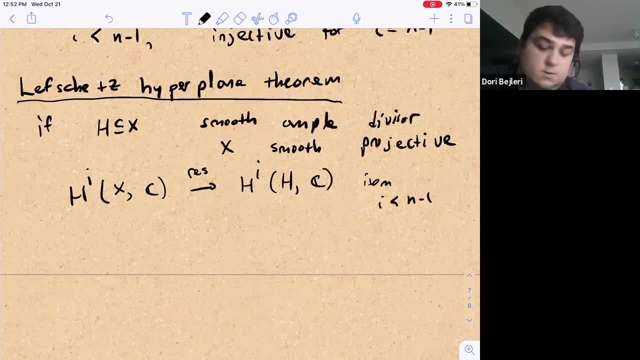 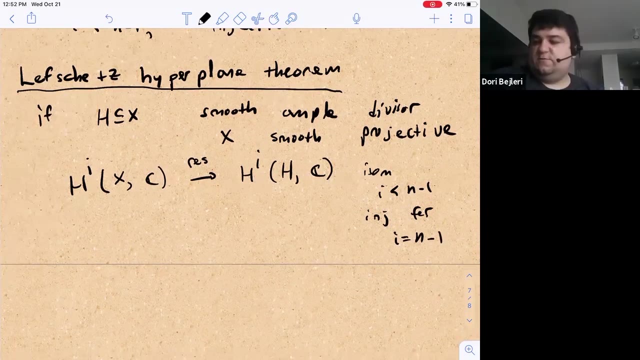 I less than n minus one, and their injective For i equals n minus one. So So it's a very Important, famous classical result. I won't give the proof, but I'll just say a few words. What comes up is the fact that, since H is ample than the complement of H, is an affine variety. 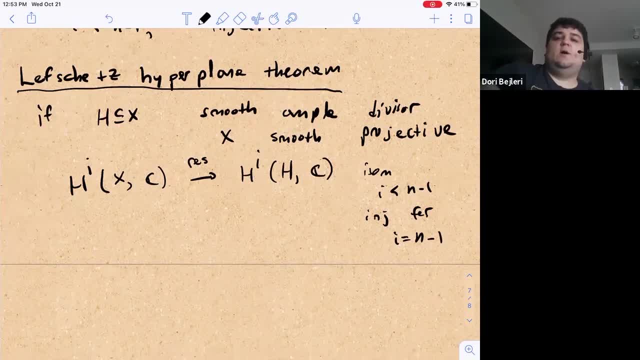 So we have complex combology of complex affine varieties that is worth half the dimension that you'd expect. And then there's a long exact sequence that relates the cohomology of the affine compliment to this restriction map on the cohomology of X and H. 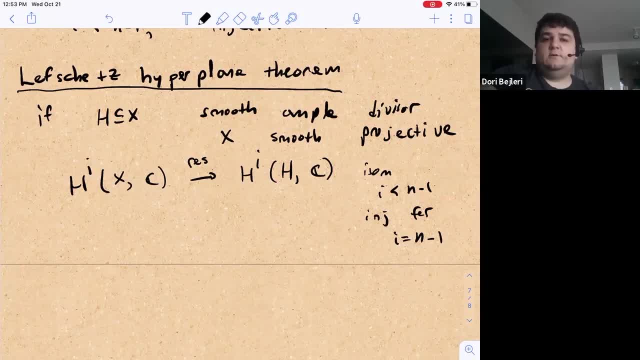 And then, and then you can use a famous result that says that the cohomology of complex affine varieties are half the dimension that you'd expect, That complex affine varieties have the homotopy type of a CW complex of half the real dimension, And so that that that kills off the core kernels and kernels of these restriction maps in the right. 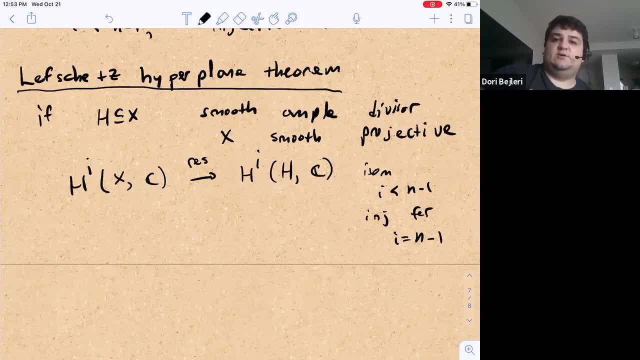 The definition of a CW complex and therefore we have a combination in the right way, Okay, in the right degrees, and that's how you get it exactly for half of the degrees, minus one where you have singular cohomology, because the singular cohomology goes up to the real dimension. 2n. 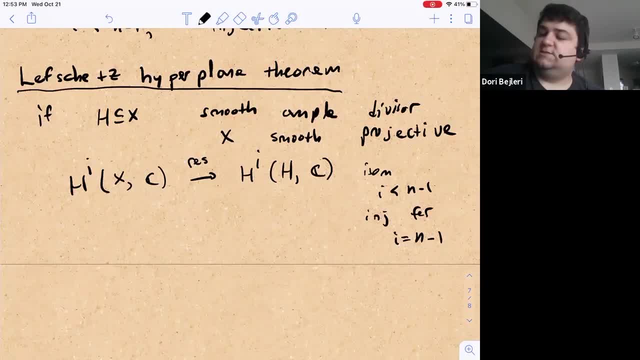 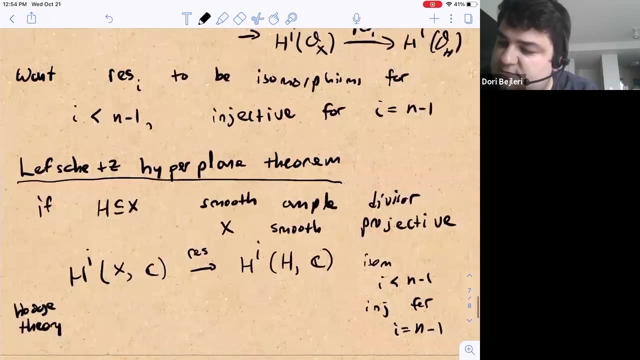 and so we get it for these, uh, in these, in these degrees, because the complement has half the cohomology that you'd expect. um, okay, but then then we use some hodge theory, because we don't care about singular cohomology, we care about the cohomology of o. 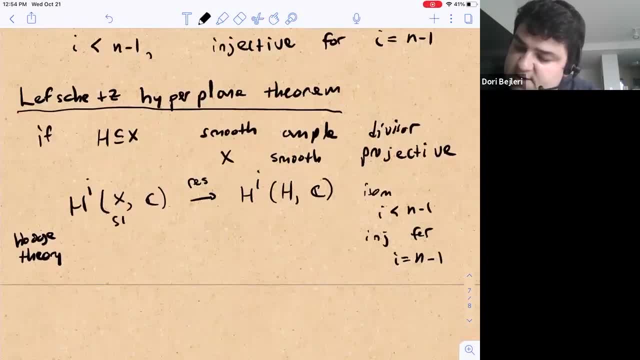 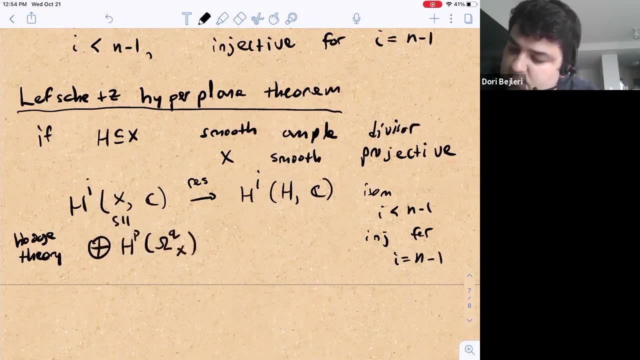 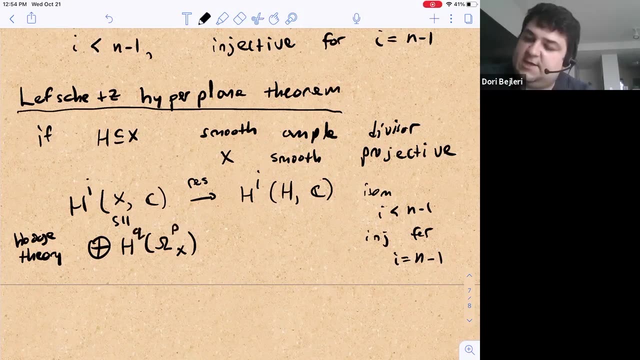 but hodge theory tells us that this is the direct sum of hp, omega, q, x or maybe i. i really should get in the habit of writing it the other way, because that's the convention with hpq, where p plus q is equal to i, and this is the same thing for h. 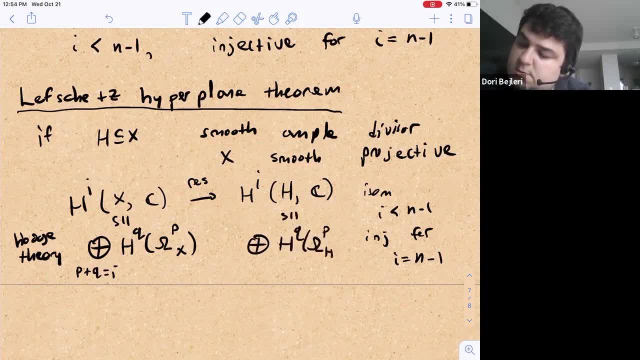 and then the. the only input left is that the restriction map for singular cohomology is really functorial with the restriction maps for these coherent cohomologies. that this diagram, where here i put the direct sum of restrictions for hpq, really commutes with this restriction. 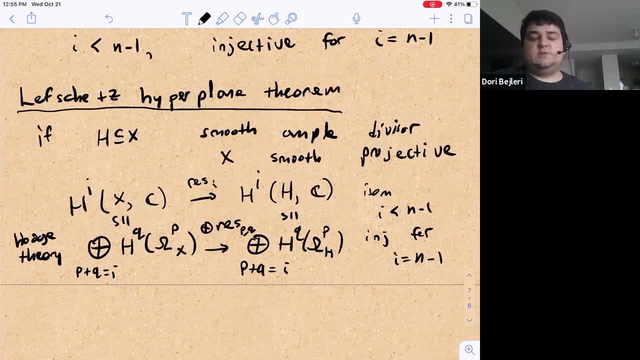 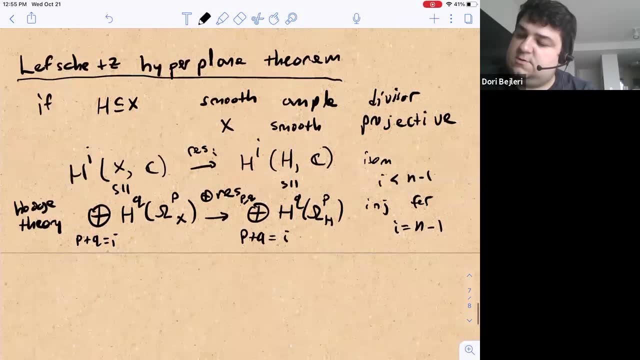 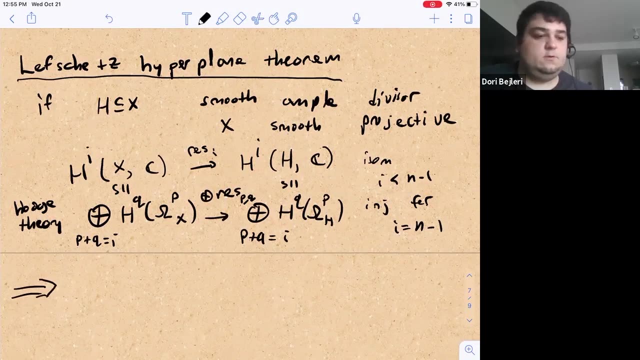 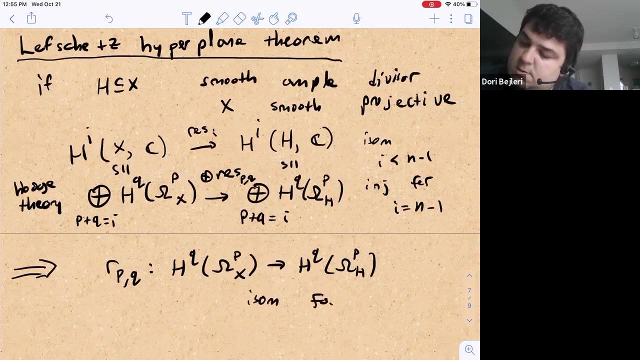 uh, for for singular cohomology, so that that's the kind of naturality of the hodge decomposition. and so this tells us that. well, it tells us that these restrictions on hodge groups, huh, there are isomorphisms, for i less than sorry for p plus q. 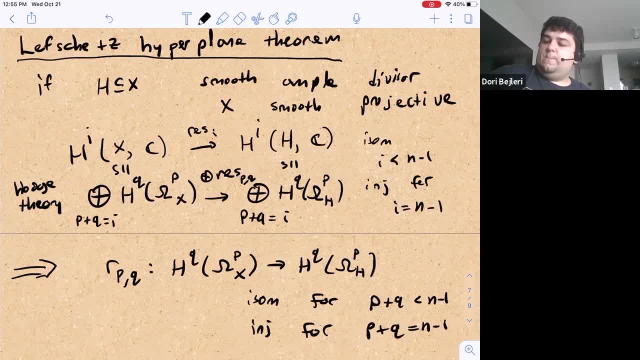 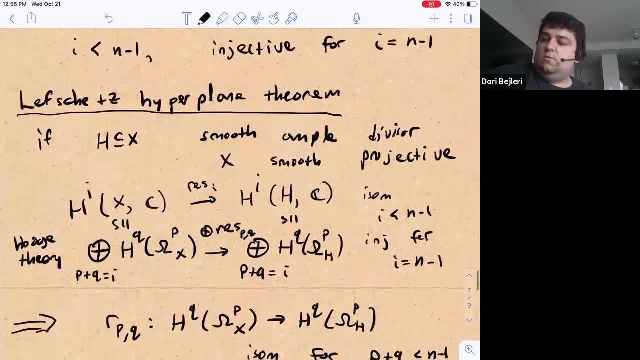 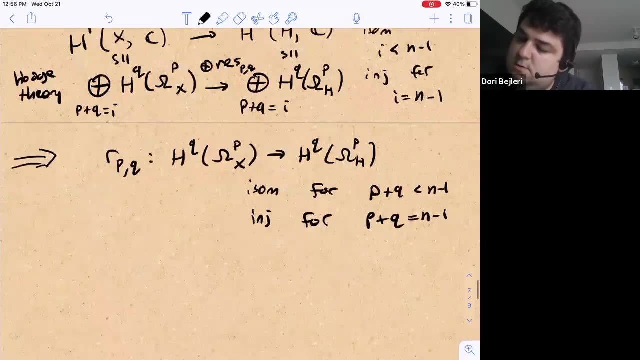 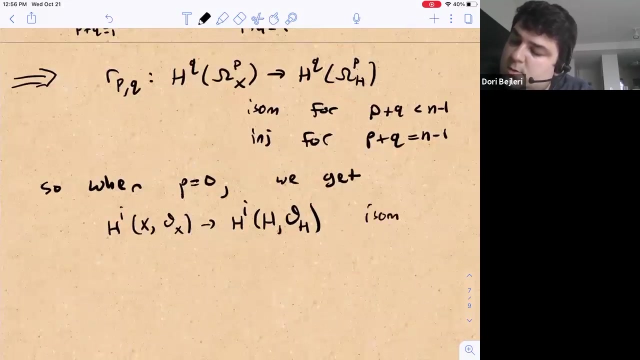 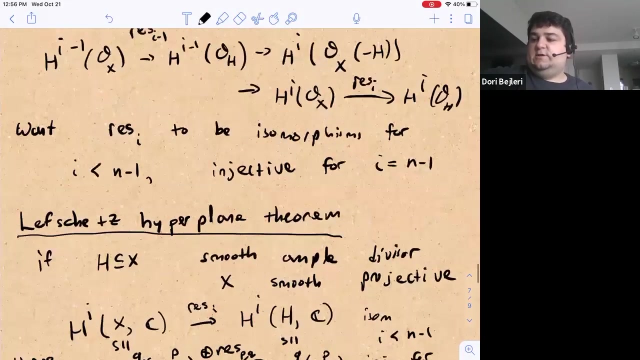 less than n minus 1 and injective for p plus q equaling to n minus 1. but these restriction wraps, as a special case, are these restrictions? because these are the cases where p is zero, And so we get our quadrira vanishing, in this case by this long, exact sequence, as we observed above. 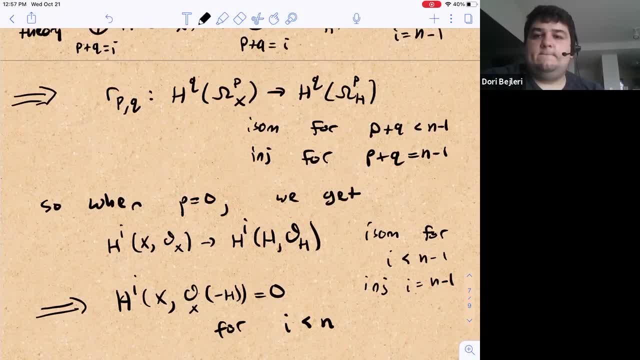 Now step two: we want to reduce to this case, so we want to have some L. that's not necessarily a smooth, effective divisor, but it's just some divisor that happens to be ample, and we want to reduce to this smooth case using cyclic covers. So this is a trick that already came up. 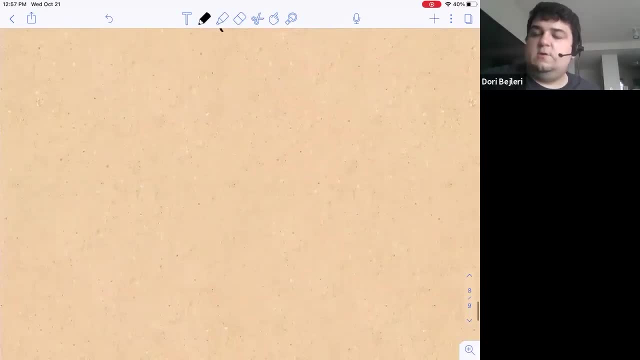 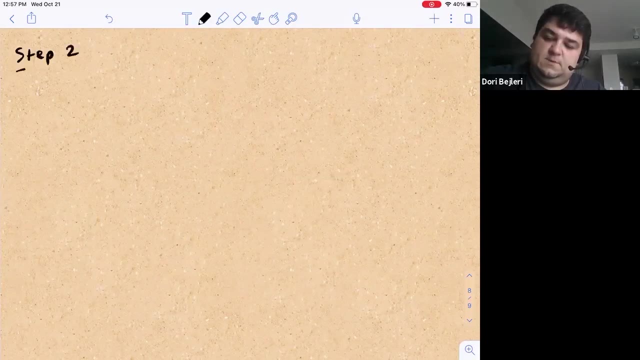 when we were classifying surfaces And it's just sort of a trick that we're going to use to reduce to this case. So we want to reduce to this case using cyclic covers. So we want to reduce to this case using cyclic covers. 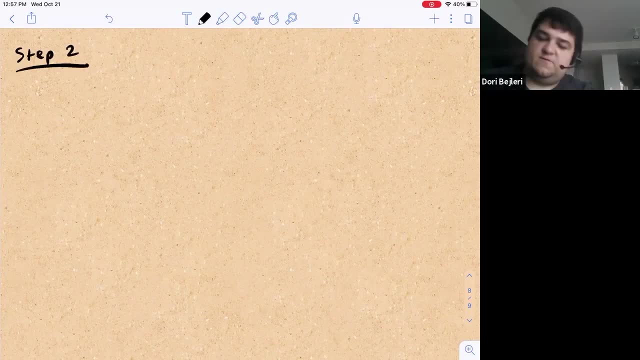 And we want to reduce to this case using cyclic covers, And this is a really key and useful technique improving these vanishing theorems. So it'll come up over and over again, But we need something slightly more general. When we were classifying surfaces, we we wrote down the cyclic cover construction for where you get unramified cyclic covers associated to torsion bundles. 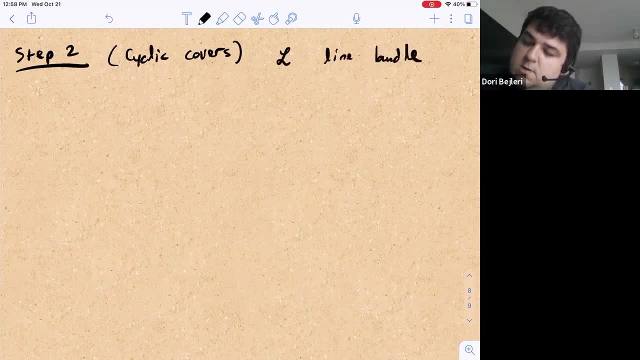 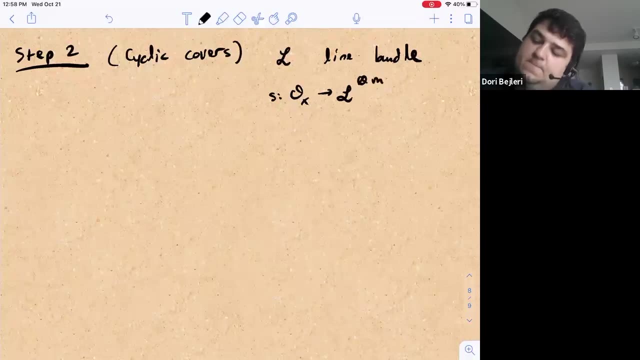 And now more generally, if you just have any line, bundle l and let's say we have a section of l to the tensor m. so in our previous setting we had actually a non-vanishing section, so s was actually an isomorphism. now we have something more general, just any section, maybe non-zero. 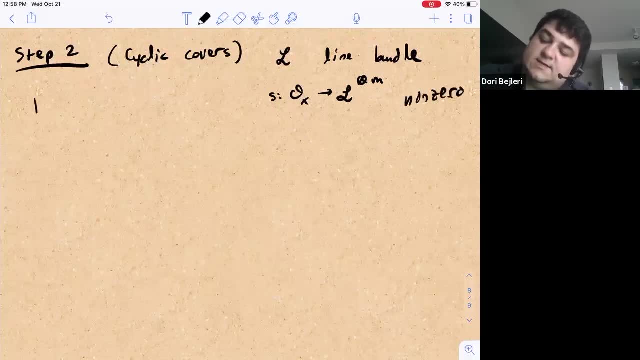 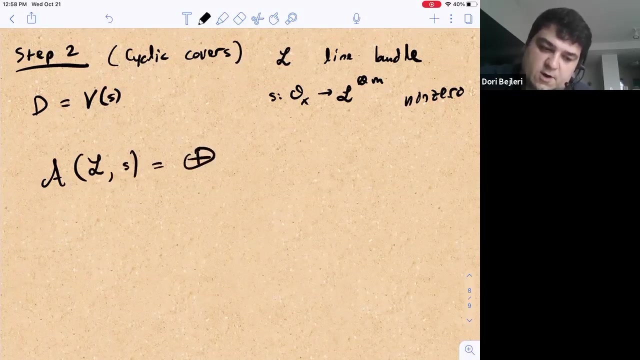 and let's say d is the divisor associated to the section, then we can construct a cyclic cover that's branched along d and that's an m-fold cyclic cover as follows: so we want to define an algebra to take spec of and it looks exactly the same as before. our algebra is: the sum from i equals zero to m minus. 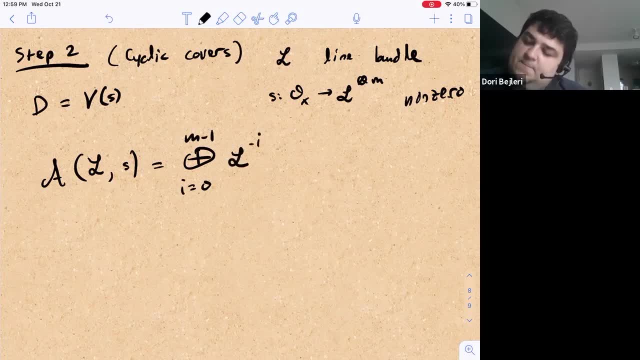 one of the line bundles l to the minus i, and we want to define a multiplication that's compatible with the grading. and we want to define a multiplication that's compatible with the grading. and we want to define a multiplication that's compatible with the grading, and so for that we look at the usual multiplication map. 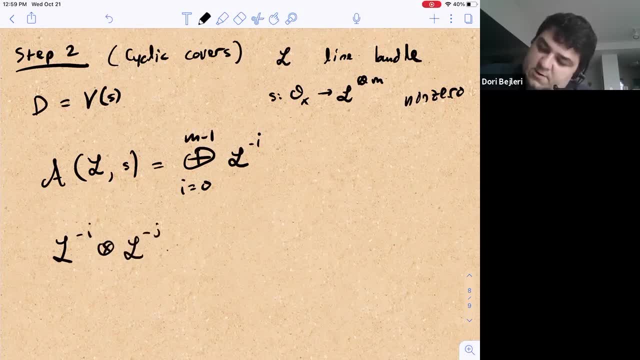 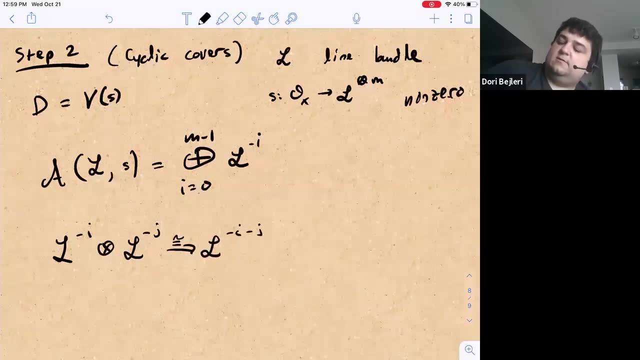 on this line bundle. but now l to the minus i minus j is not actually one of the terms in our algebra, so we need to shift by the section s to get back to, to something in degree between zero and m minus one. so we apply s, tensor, the identity, to get something. 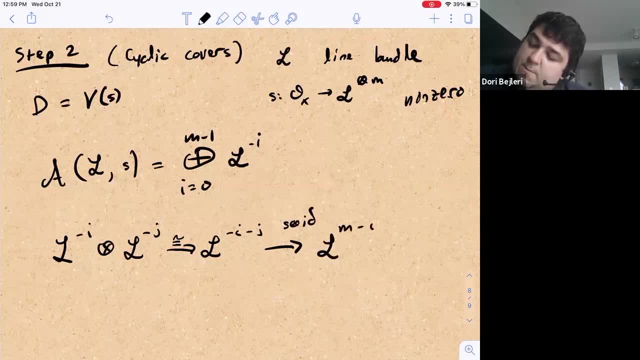 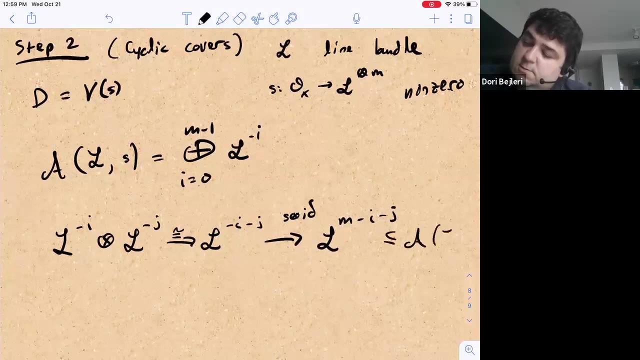 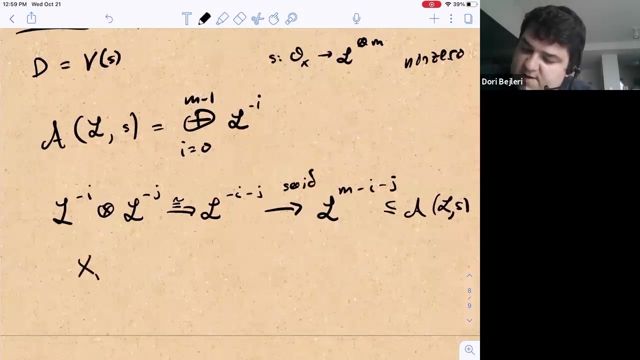 in l to the m minus i minus j, and now if i and j are between zero and m minus one, then m minus i minus j will be in that range, and so this gives us a multiplication on on this algebra a, and so now we'll just define x and d to be spec over x. this 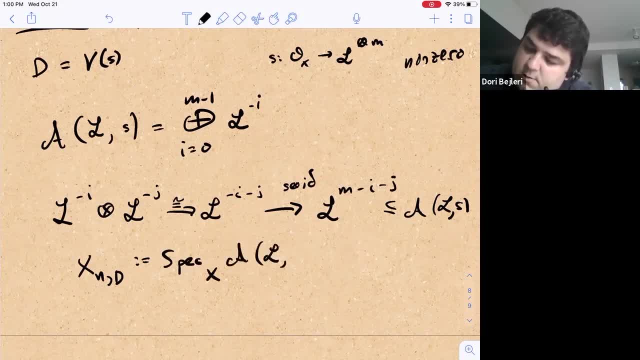 relative spec, and then we'll just define x and d to be spec over x- this relative spec. and then we'll just define x and d to be specこの a and d to be spec over x- this relative version. this is actually static here. that's special. so now let's try after refining ourselves. 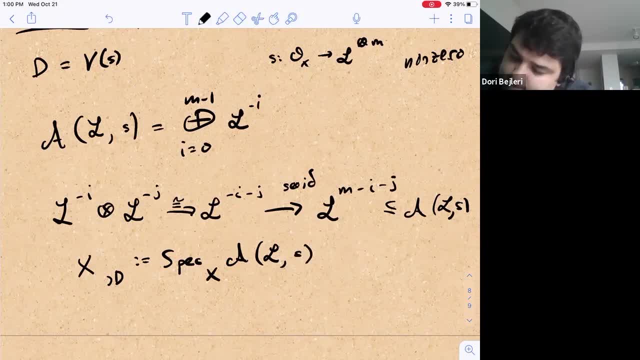 and let's try it this way now, let's face it. so x is here, we have this Yeager setup, nice of an, okay, so that's that's just the abstract definition. we constructed an algebra, took its spec- uh, that's some scheme that's affine- over x. 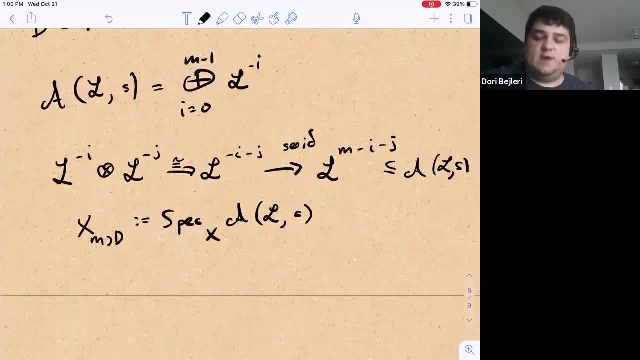 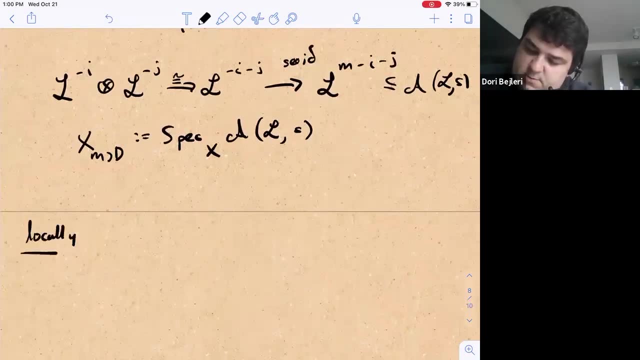 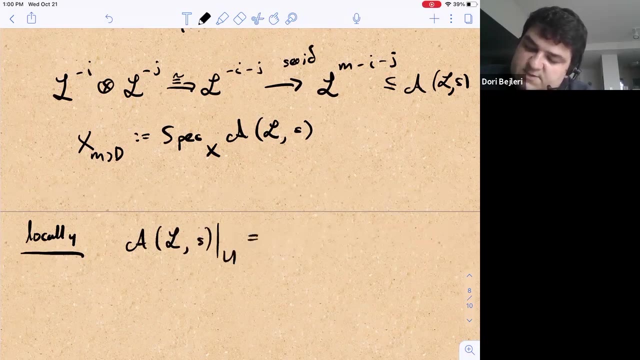 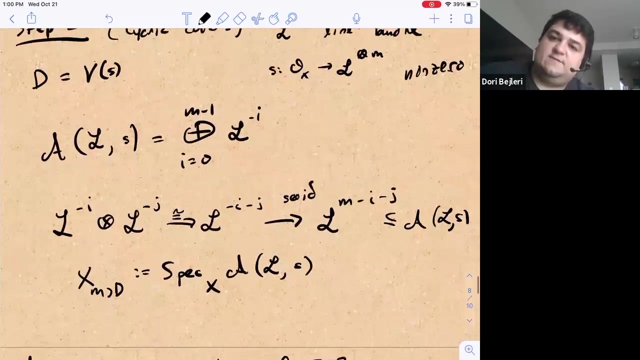 um and the algebra's finite coherence was actually finite over x, but we really want to understand it a little better. so the the key point is that, locally, What is this algebra? If we trivialize everything, then this just looks like OU adjoin a single generator, Z, so where the degree I term is generated by Z to the I. 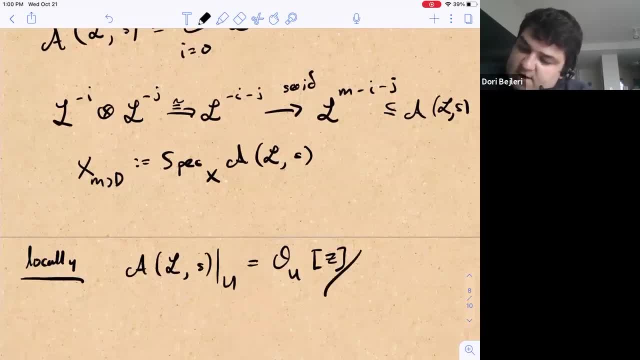 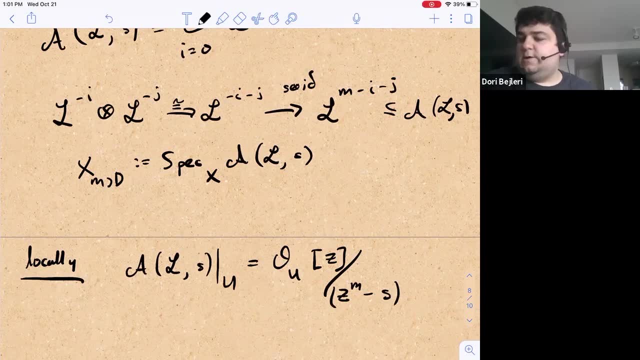 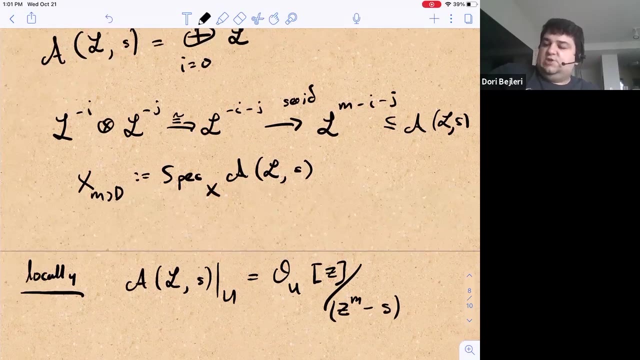 But now we're quotienting out by this multiplication is exactly saying that Z to the M is equal to our section S, And so locally, this algebra is just this algebra: OU adjoin Z mod Z to the M minus S, And so what is this thing? 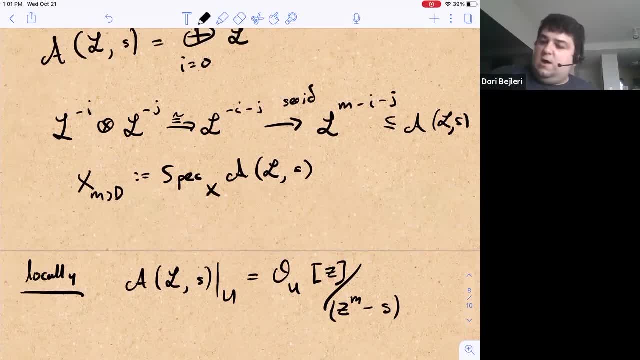 It's a cyclic cover of degree M, So by that I mean it has an action by the Mth roots of unity. It's a Galois extension of algebras with Galois group mu, M, And it's ramified exactly where S vanishes. 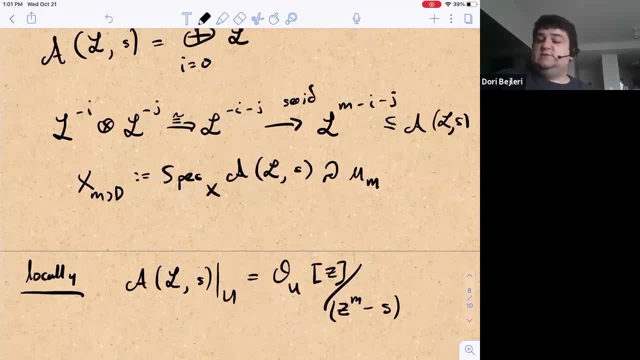 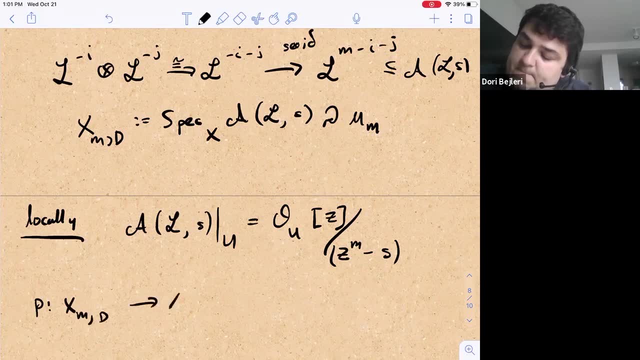 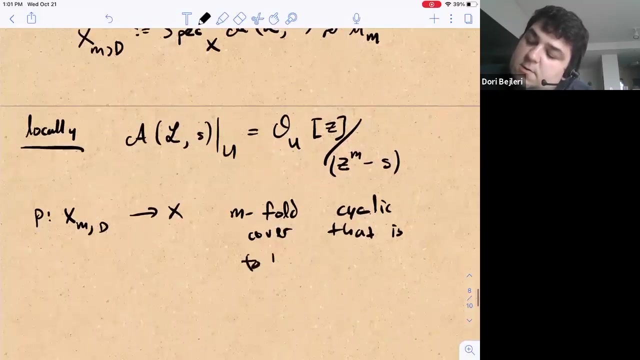 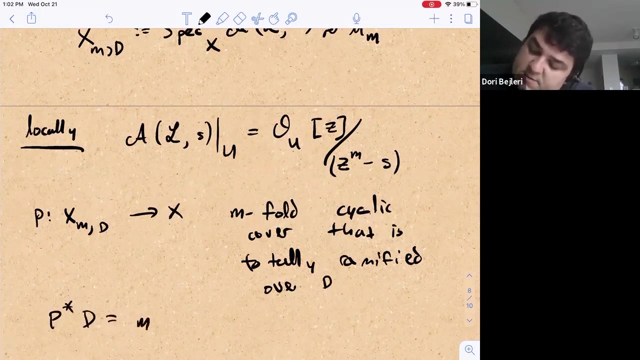 And it's totally ramified Because it's Z to the M equals S. So the upshot is that this map is an M-fold cyclic cover that is totally ramified over D. And so if we look at P- upper star D, then that's going to be equal to M times some reduced divisor, DM, where the reduced divisor is the vanishing of Z. 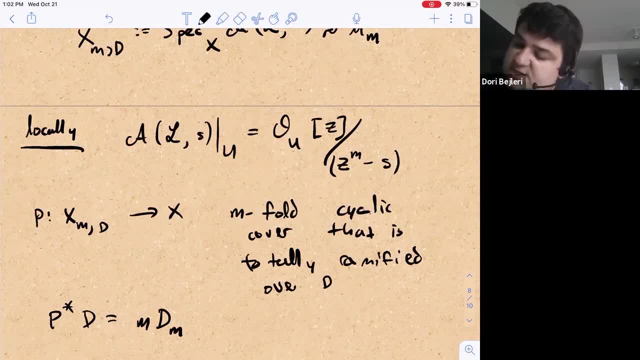 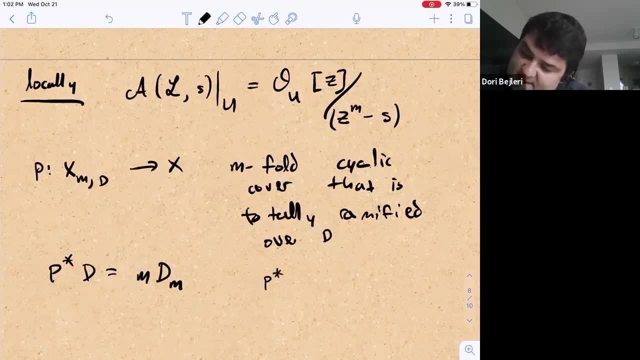 So the vanishing of S is M times the vanishing of Z And in terms of line bundles, P upper star of L is now isomorphic to OX of DM. So the point is L itself. It's not necessarily effective, but L to the tensor, M was. 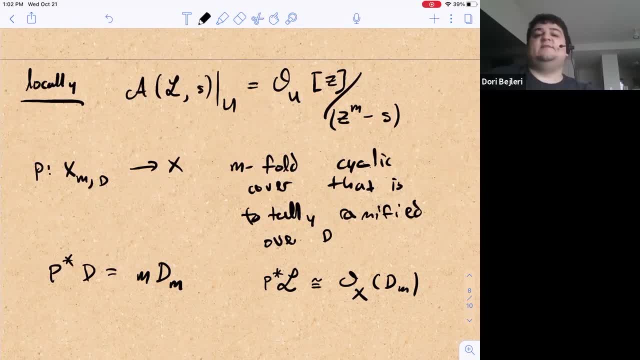 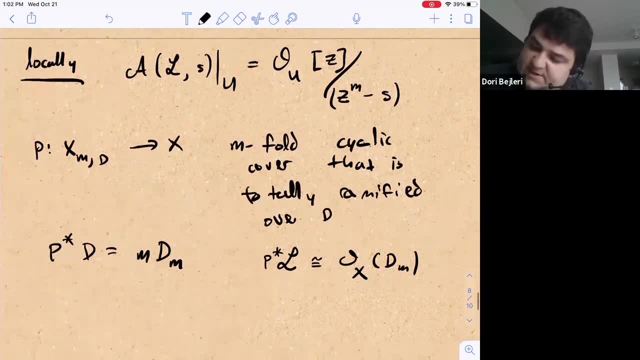 And so now we've extracted an Mth root of L. We've extracted an effective divisor for L after taking an Mth root. The other observations are that the projection map from DM to D is actually an isomorphism. Again, that comes from looking at this algebra description in terms of affine coordinates. 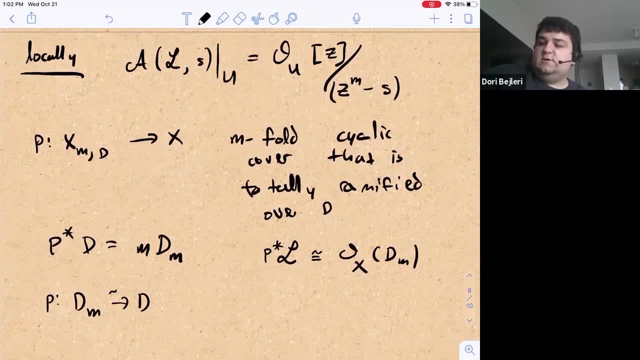 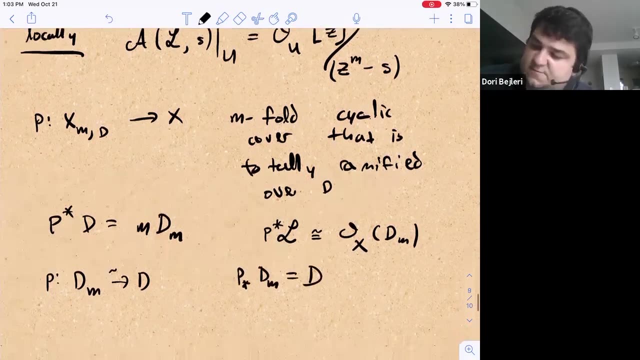 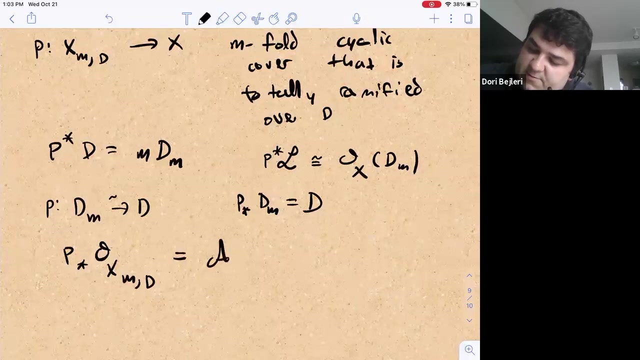 Because if you look at the reduced vanishing of S, well, that's just the same as OU mod S, just from this algebra, So this is an isomorphism. And so P lower star DM is D. And then, finally, just from the definition of relative spec, P lower star of OX MD, is this algebra that we took spec of. 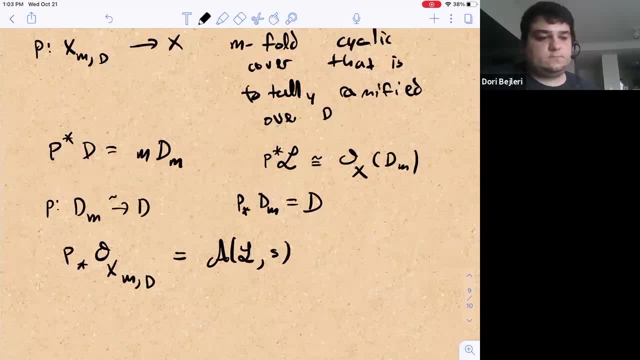 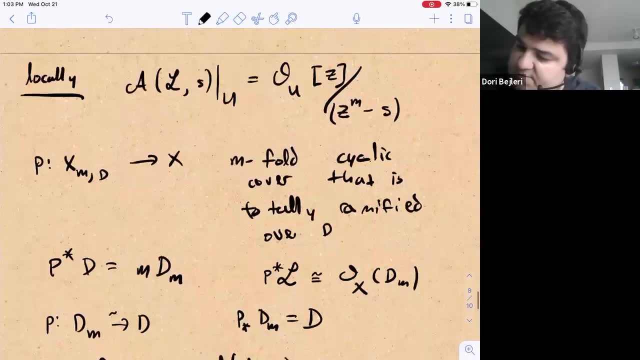 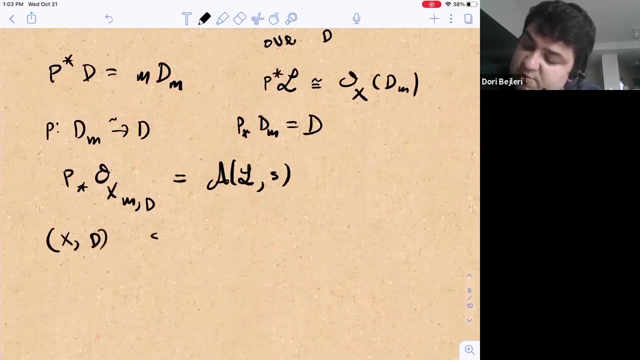 Some formal property of relative spec. Okay, I said finally, but there's actually one more, one more fact again coming from just looking at this local description: If X comma D is a smooth pair, So if X is smooth and D is also smooth, then that implies that XMD comma DM is also a smooth pair. 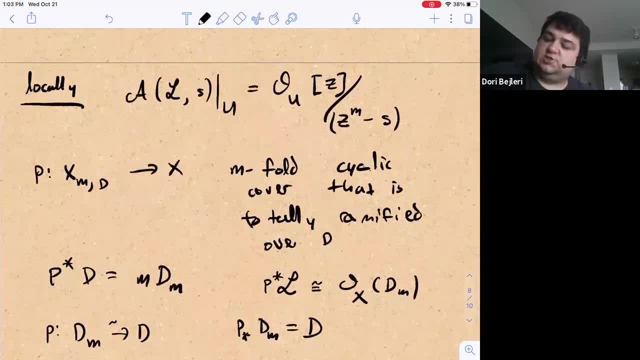 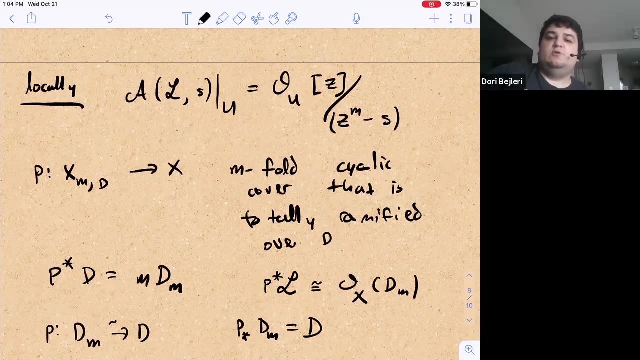 And again, that just comes from this local description. So if X is smooth, then After completing we could, we can write down this OU as some some polynomial ring, And then we're joining one more variable and modding out by Z, Z to the M minus S, where S is a smooth, cuts out some smooth locus in the polynomials X one through X N. 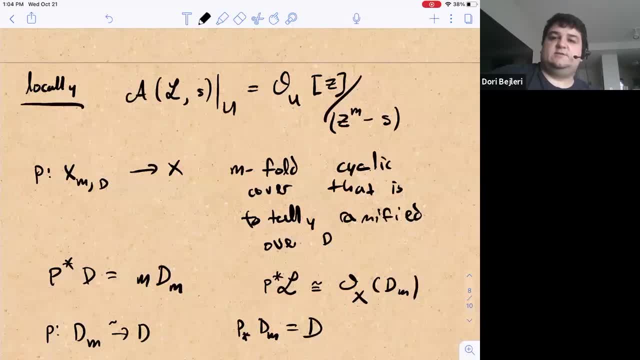 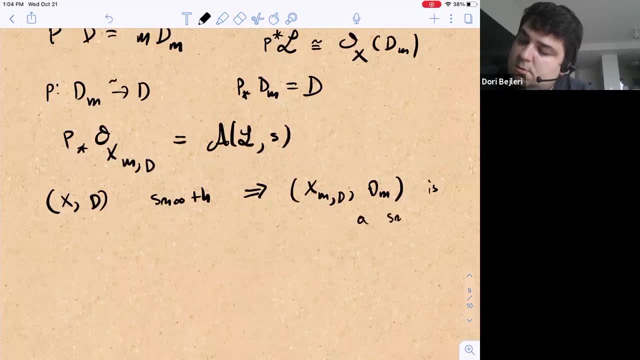 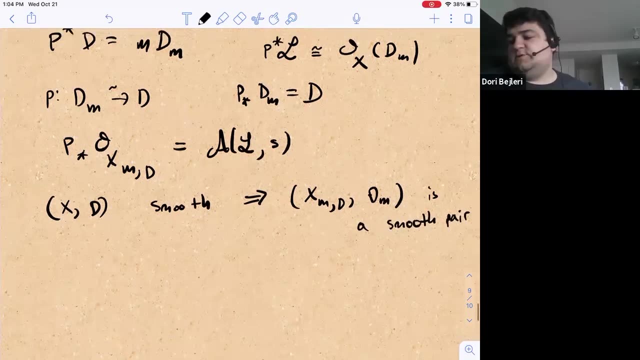 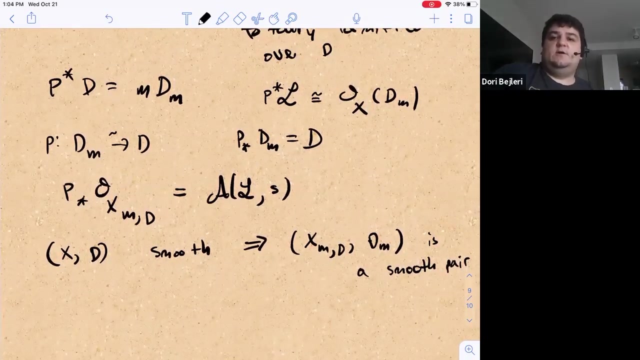 And so then, by taking derivatives of the Z to the M minus S, you see that that this guy is also smooth. okay, so now our strategy is to uh say, we have this ample divisor. that's not necessarily an effective smooth divisor, but because it's ample, we know that some large enough power is very ample. 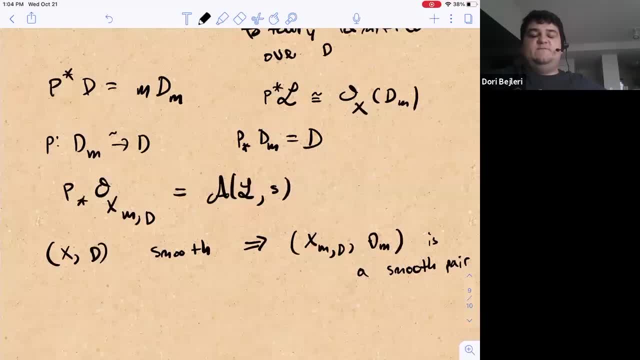 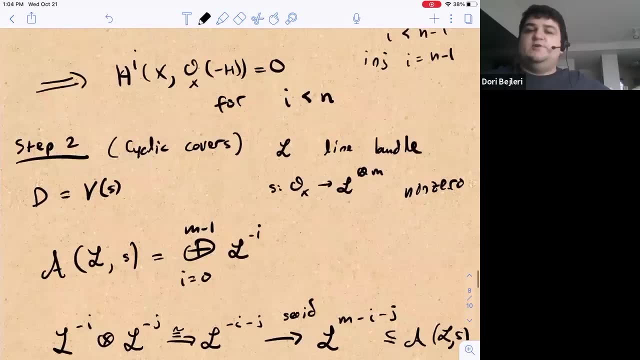 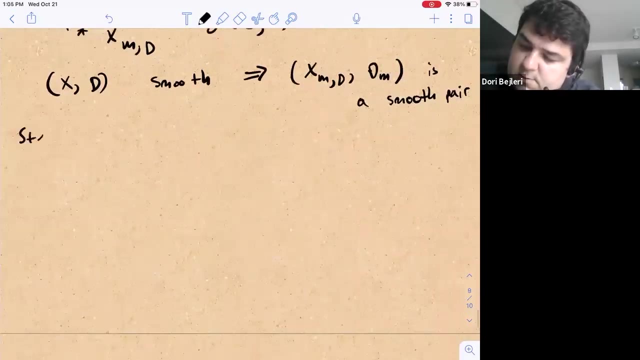 and so we can take a generic hyperplane section of that large enough power and that's a smooth divisor. and so then we're going to apply this root construction to our l to reduce to the case of step one. so so now we're back to our setting, uh, and then the step three: we're going to show the vanishing. 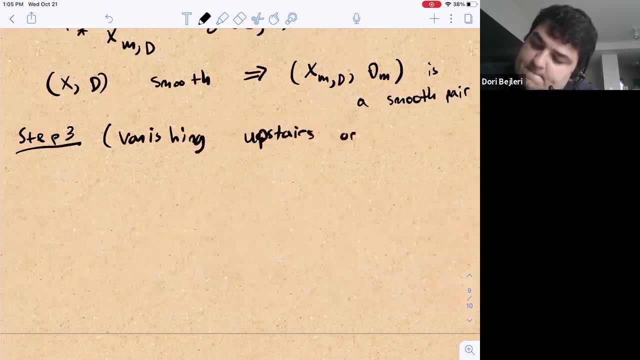 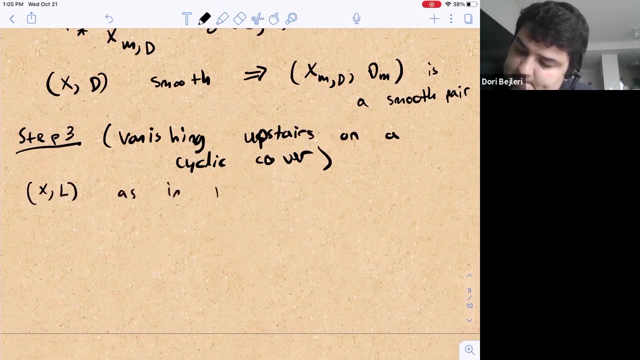 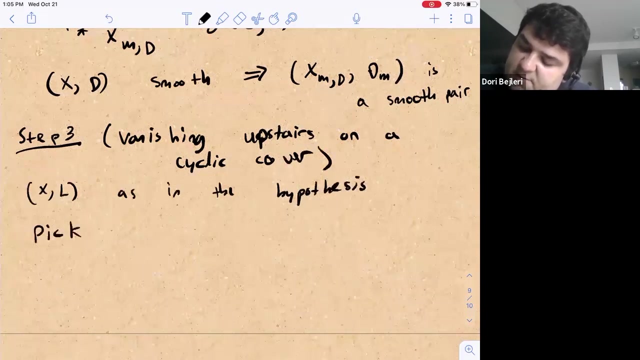 upstairs on a root. so so now we're in our setting of x comma l, and so we're going to show the vanishing upstairs on the root. so now we're in our setting of x comma l, the hypotheses, and we pick some very ample, smooth, hyperplane section of a large multiple. 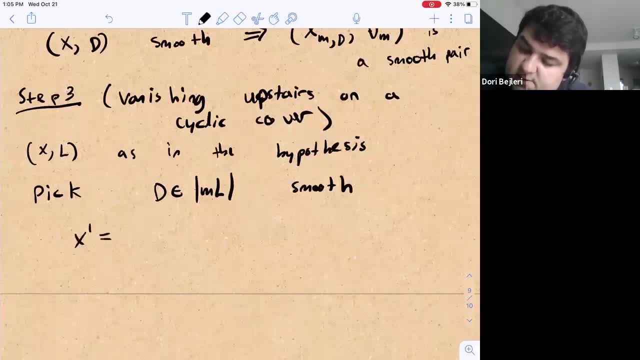 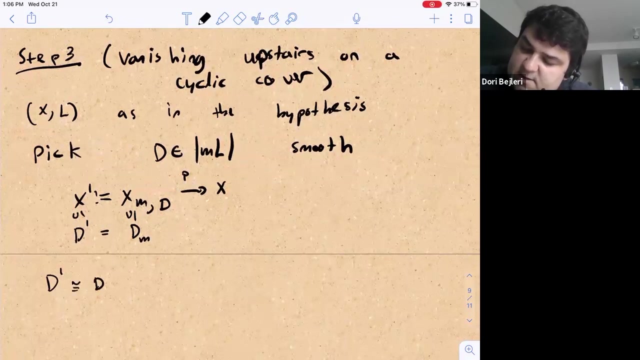 and now we construct the cyclic cover. so let's just denote x, prime, uh, as the cyclic cover, uh, the unfold cyclic cover, branched along d and um. right, and that's just a note- by d prime, the divisor, dm, the root of d? um. so now d prime is isomorphic to d abstractly, so in particular it's a smooth. 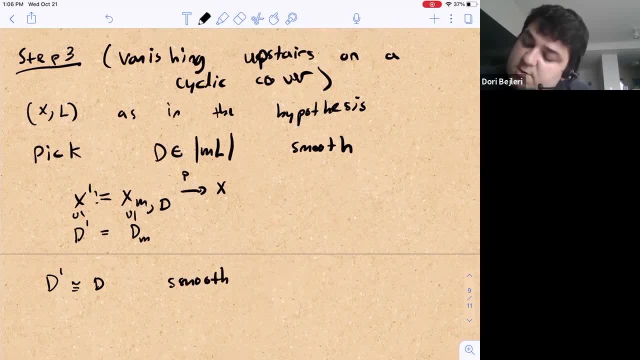 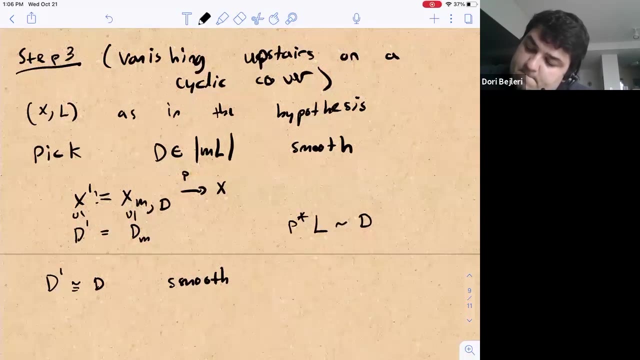 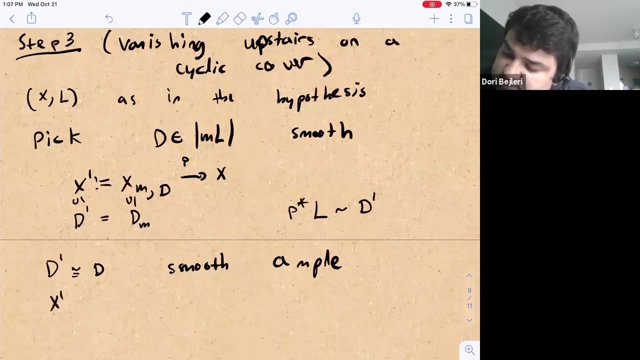 smooth divisor. but also p upper star of l is linearly equivalent to this d prime, and so that's actually what we're trying to do with the sample, because, uh, it's the pullback of some ample divisor by some finite map, um, so we have the smooth, ample divisor. we also know that x prime is smooth. 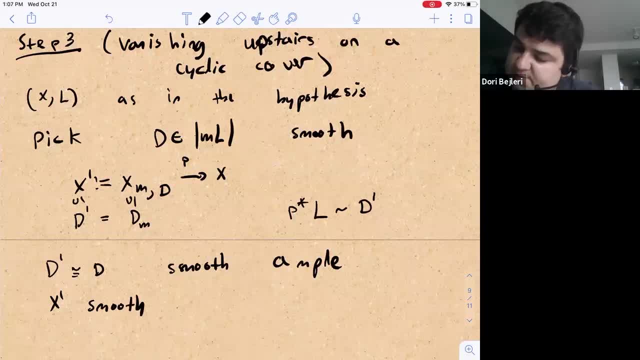 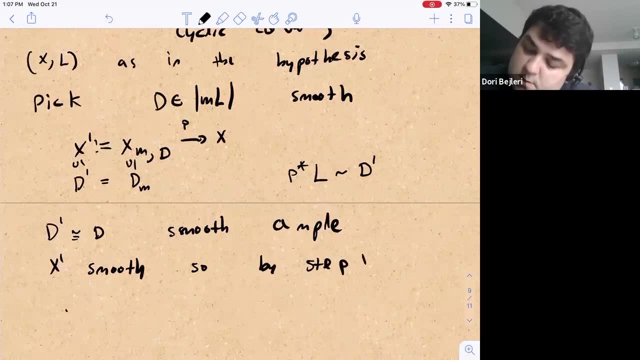 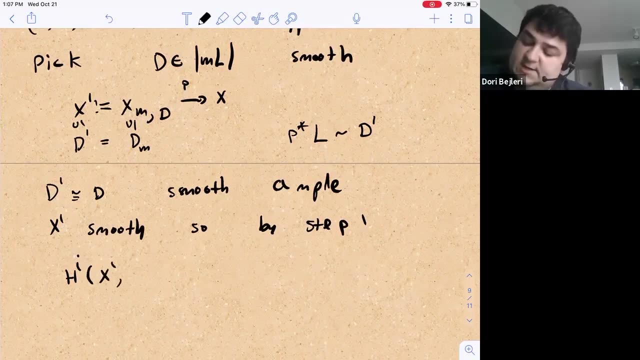 and so on, x prime with respect to d prime. we have the, the vanishing by step one. uh, then this tells us: so h, i, x prime, o, x prime minus d prime is zero, for i less than n, and the dimension of x prime and x are the same, because this p is finite. 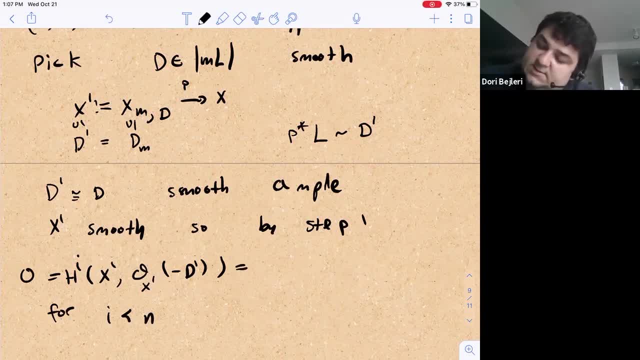 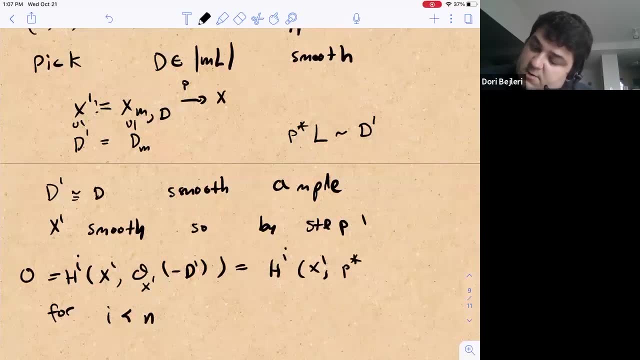 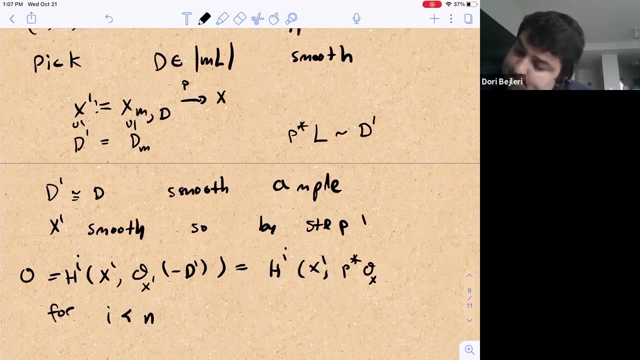 but this: we just said that p upper star l is d prime. so this is the same as saying that h i of x prime with coefficients in p upper star of the divisor. we care about a zero, okay. so what we've shown is that there's some m-fold cyclic cover. 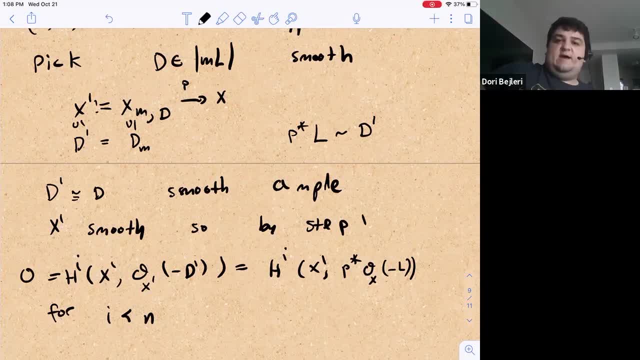 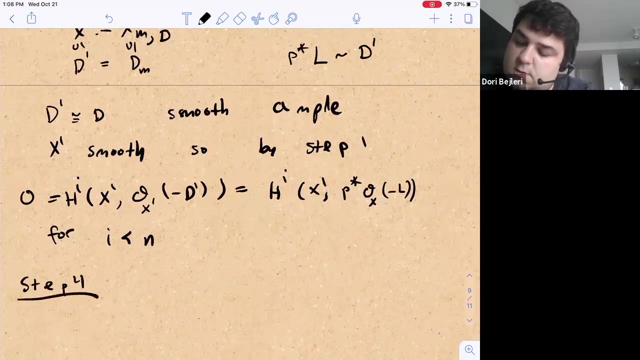 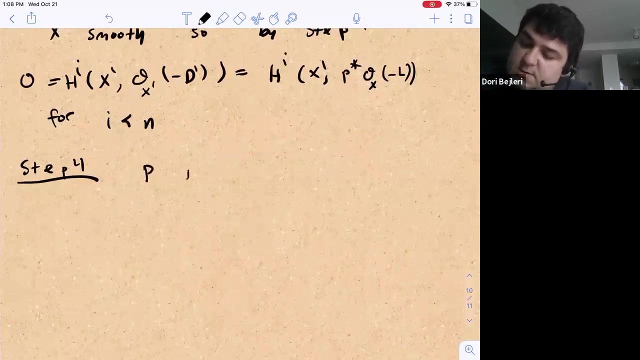 where when we pull back our our divisor, then we have vanishing for that divisor on the cyclic cover. and now the last step is to show that implies vanishing on our original x, and then from the flow all the way up to theirsiniz thequeltsivel of the ever pity. in a편아요. so, uh, if you're going to show that the accessoriesj can beaya, okay. so now, since p is finite, then we know that the higher push forwards are just zero. yeah, and so we can compute columnology upstairs or downstairs. so then, for any locally freesheaf, we have that h i, we have that theyhi. 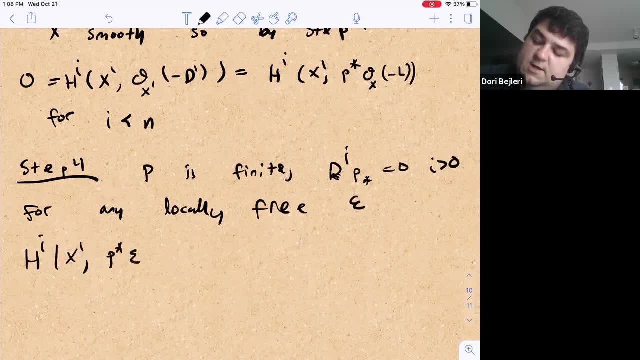 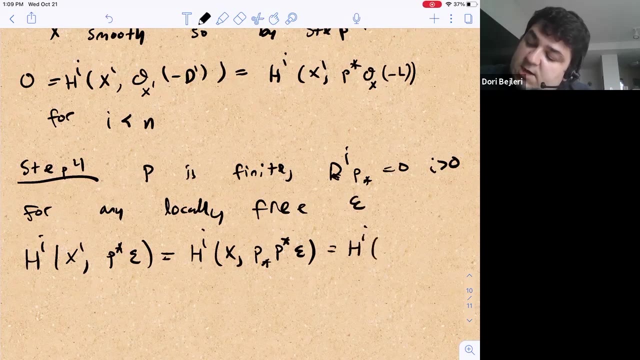 of x prime with coefficients in p upper star e is the same as h i on x with coefficients in p lower star, p upper star e. but now by projection formula, this is the same as h i, x, uh with coefficients in e tensor, p lower star ox prime, um. but then we know what p lower star ox prime is. 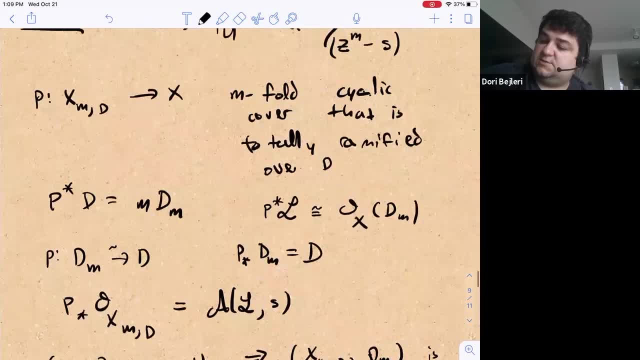 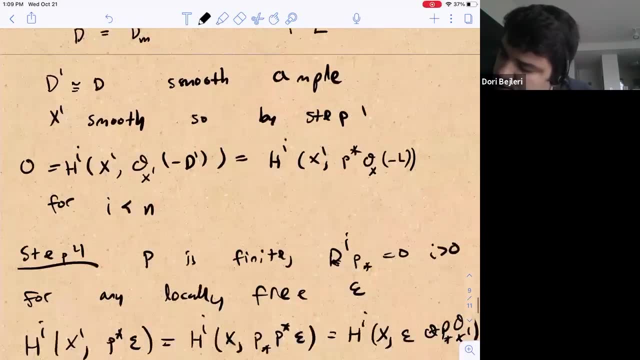 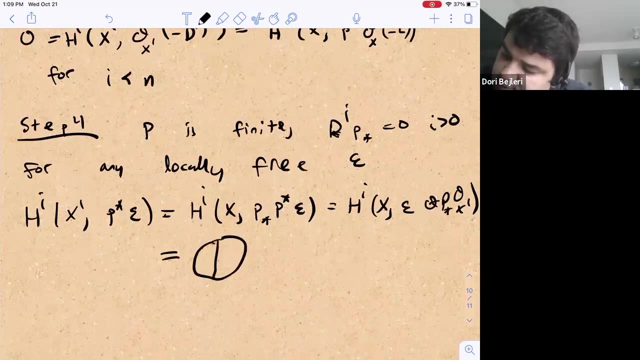 it's this direct sum, uh that we took spec of. is this, uh, direct sum of l to the minus i's? and because cohomology of a direct sum is direct sum of the cohomologies, we can just write that this whole thing is equal to direct sum from i equals zero to m minus one. 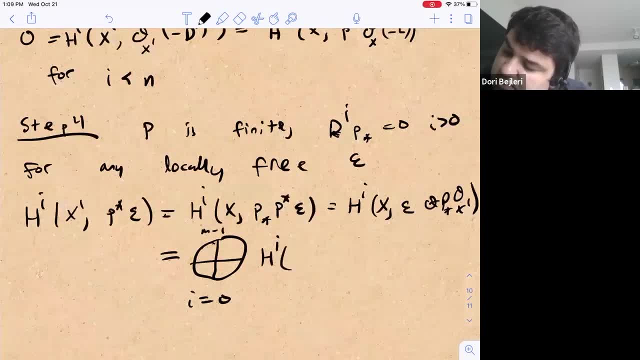 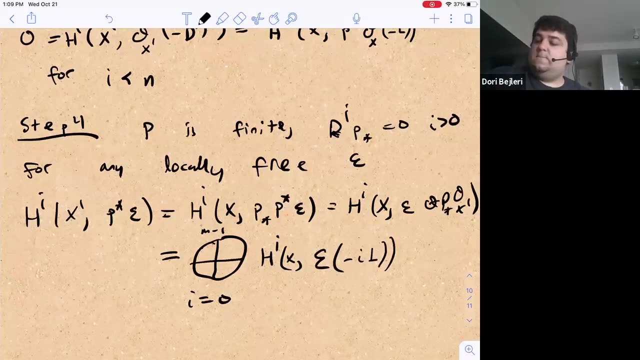 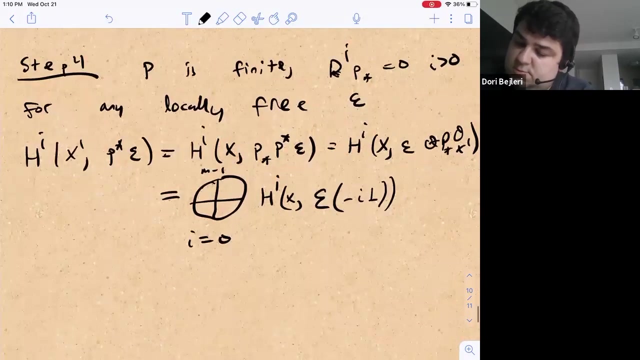 of h i, with coefficients in e twisted, twisted down by our l? um right, and so, in particular, now, uh, we apply this to e equals ox minus l, and so, by by step three, the left hand side is zero, uh, and so that implies that each of these summands is zero. so, in particular, 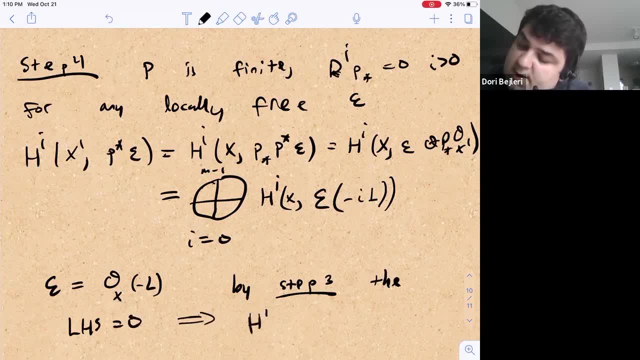 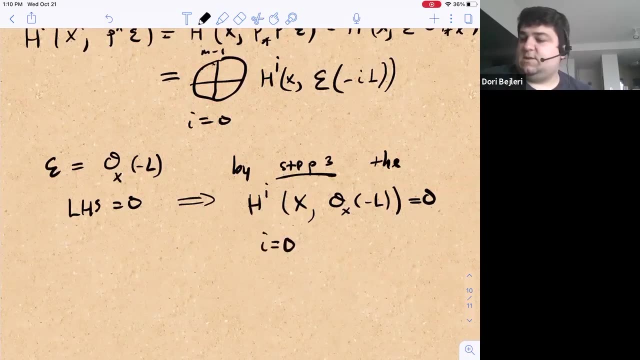 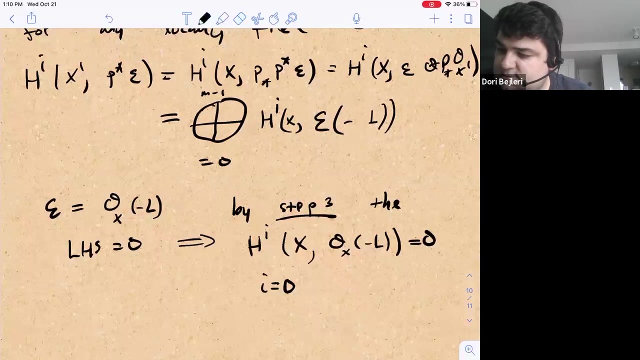 that implies that uh, h, i, x, comma, e itself, or in this case, ox minus l, is zero. uh, because that's the special case where i equals zero. oh no, i used i and i both times. sorry about that. let me uh make this a k here, in case k is zero. 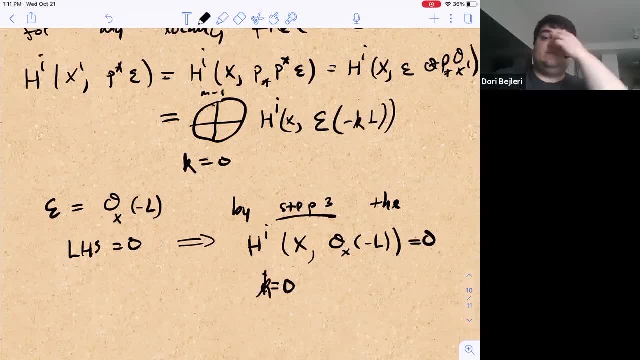 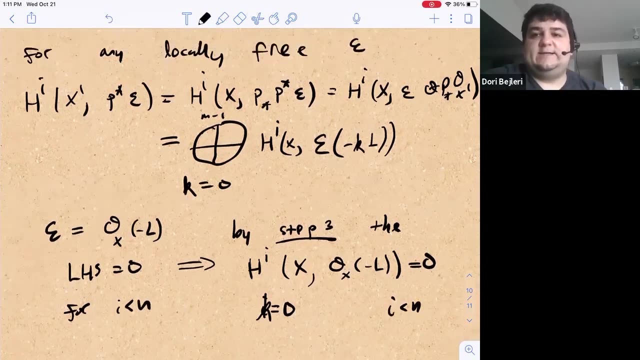 there we go. so a special case where k is zero is when you just have the e itself. um, okay, so that's. uh. that completes the proof of the classical qadari vanishing theorem. um, are there any questions? okay, um, so in the last few minutes, let me give a generalization that uh. 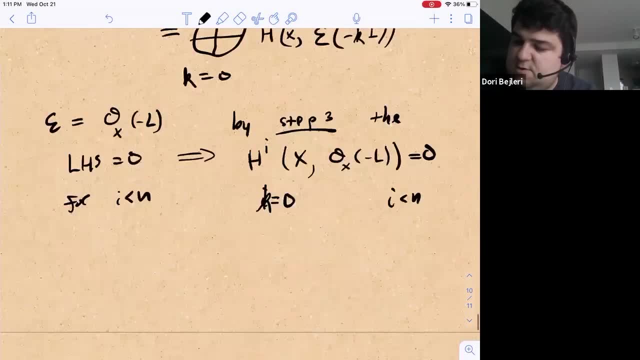 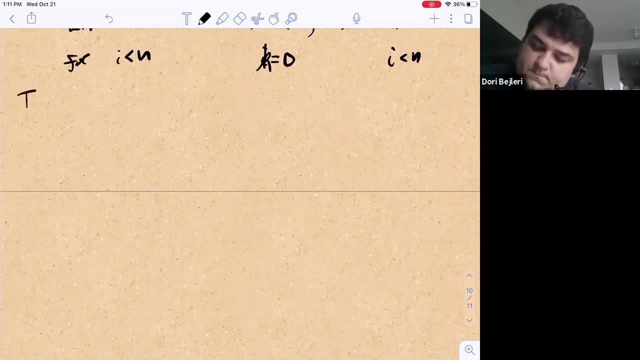 i won't do the full proof of, but it's just useful to know. um, i don't think it's going to come up again in this class, but maybe it will not totally sure. um so, kodaira akizuki, nakano vanishing. um, sometimes just called nakano vanishing. 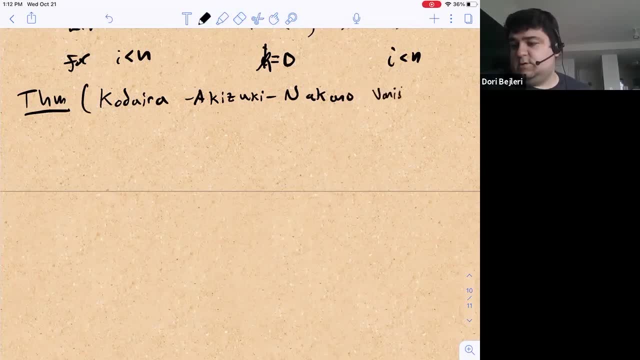 um, but it generalizes kodaira vanishing. and then i think akizuki and nakano had a paper on it together- um, um. so same assumptions. x is smooth projective. i'm going to use line bundle notation. uh, l is an ample line bundle, um. then we have the following: vanishing if we take hq. 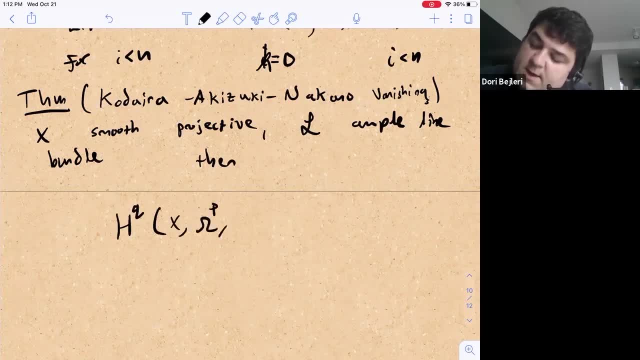 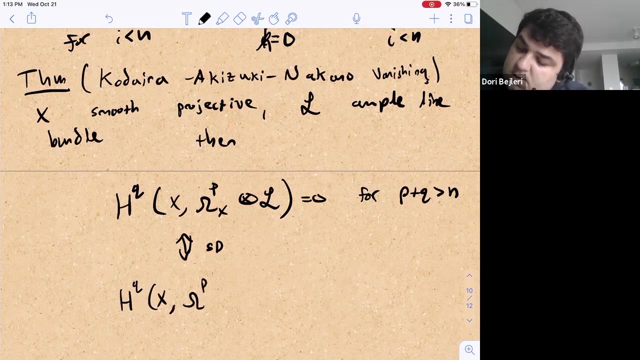 of omega p x times tensor l x x times p, x, p, x, x, p x, p, p, x, x, x strictly smaller, sorry, strictly bigger than n, or by seriduality, this is equivalent to saying that h, q, x, omega p x tensor l inverse is zero for p plus q smaller than n. 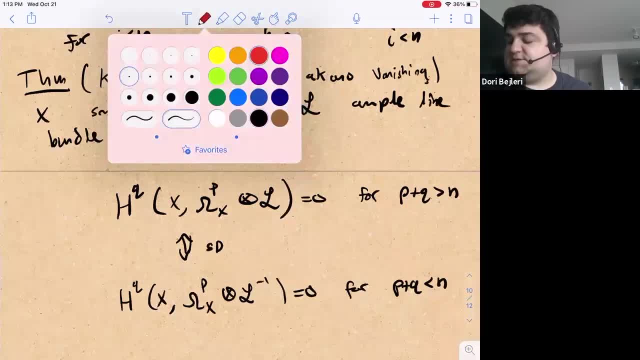 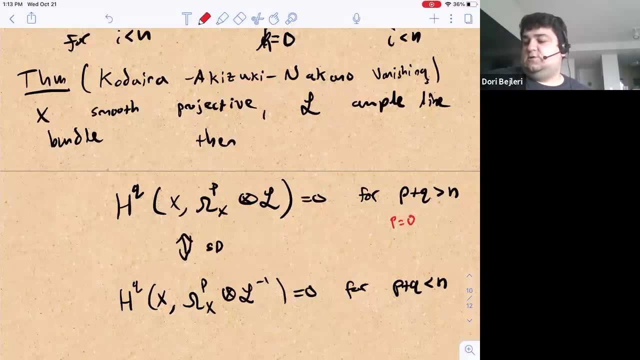 is zero for p plus q smaller than n is zero for p plus q smaller than n. And this is generalization, because if p equals 0 here, then we get sorry. if p equals n here, then we get the usual Kodaira vanishing, because if p is n, then p plus q is greater than n, is just saying that q is greater than 0. 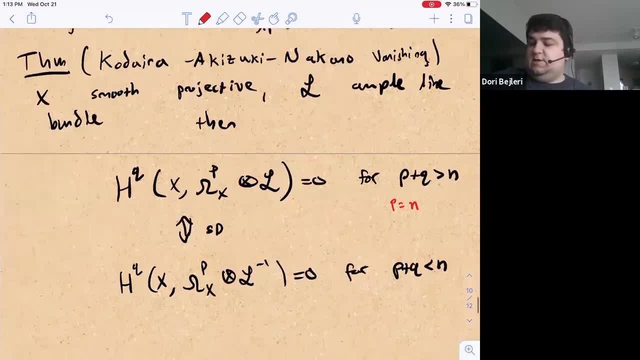 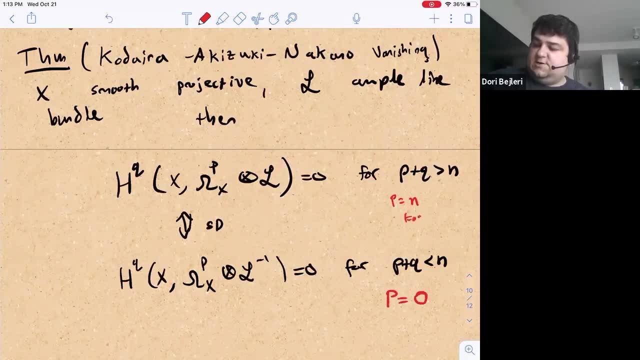 So then we get Kodaira vanishing in its first form And similarly on the seridual side. this is when p equals 0, that's the same as Kodaira vanishing in its seridual form. So this is a generalization to these more general sheaves where you don't just take the canonical but you take any of these intermediate sheaves of differentials. 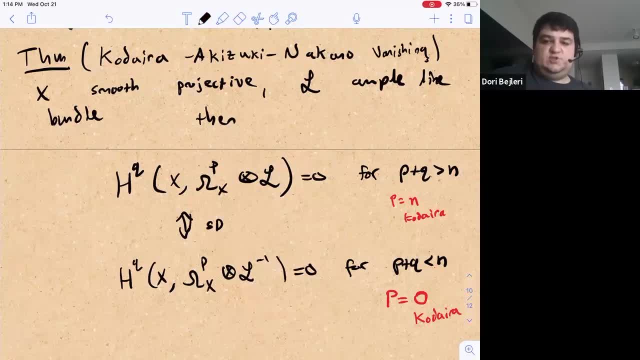 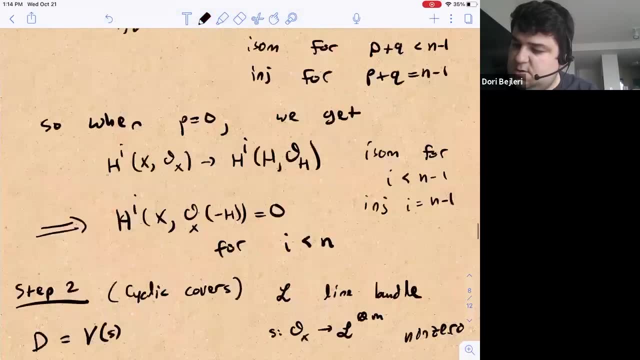 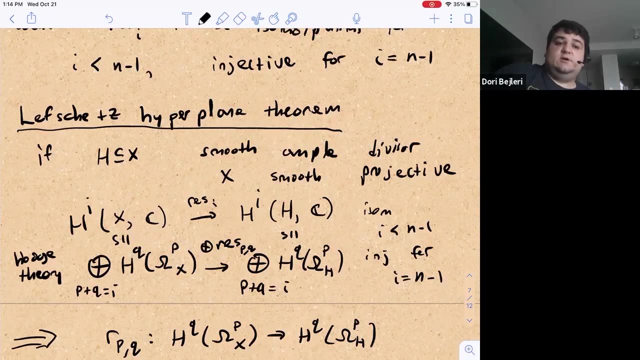 But the proof is kind of the same strategy We saw up here that in the Leschet's theorem we actually do have that these restrictions are surjective for any of these cohomologies of sheaves, of differentials or isomorphisms, and injective in the right ranges. 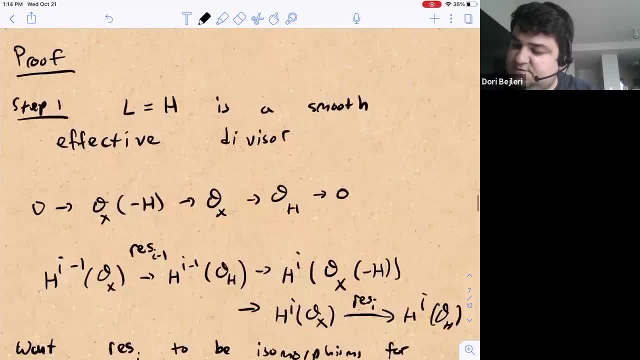 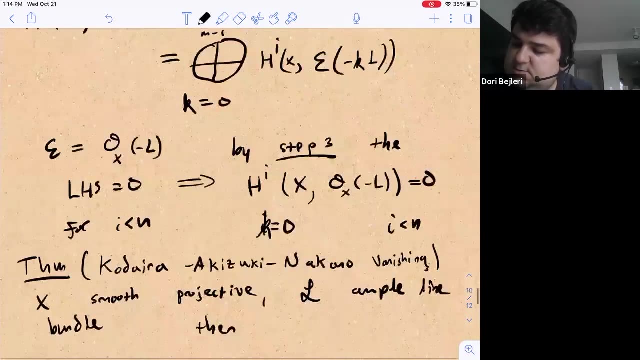 So, basically, the only difference is you need to replace this exact sequence In the case of: So we actually have a smooth divisor. You need to replace this exact sequence with some exact sequence that involves omegas instead of just O. So I'll just write down: 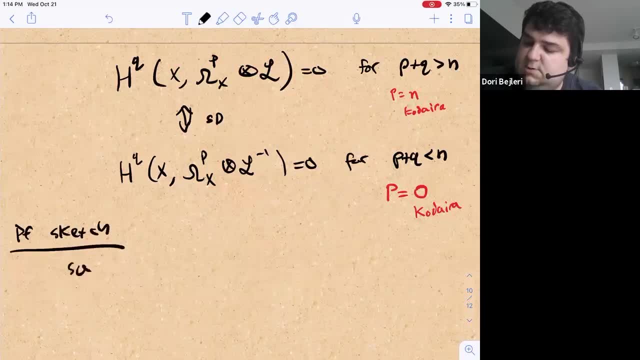 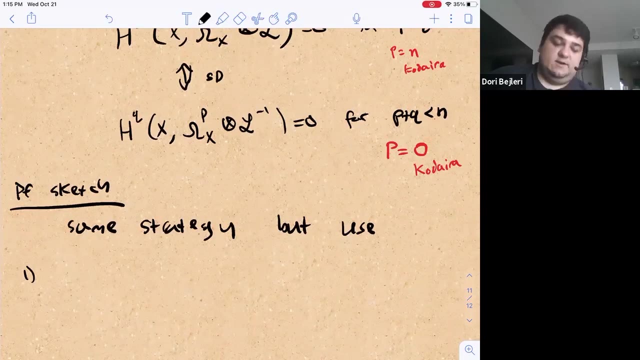 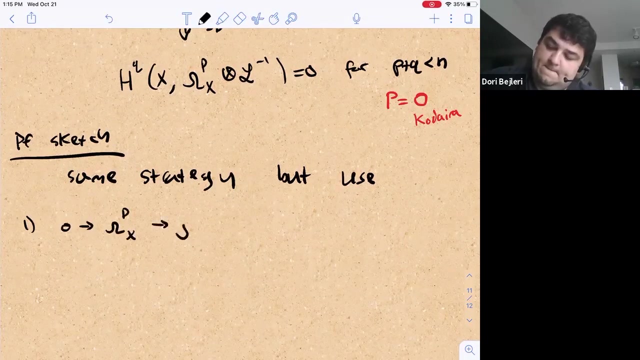 Proof sketch The same strategy But use the following two exact sequences To relate cohomology of these omega sheaves with cohomology homology of on D. So we have a sequence that's like the with these sheaves of logarithmic. 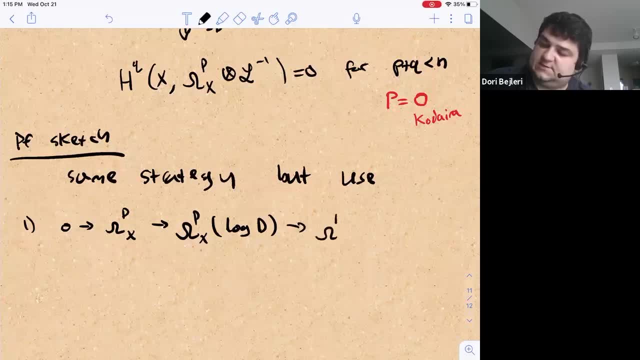 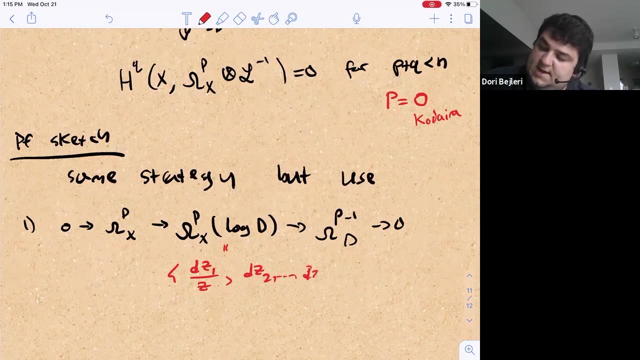 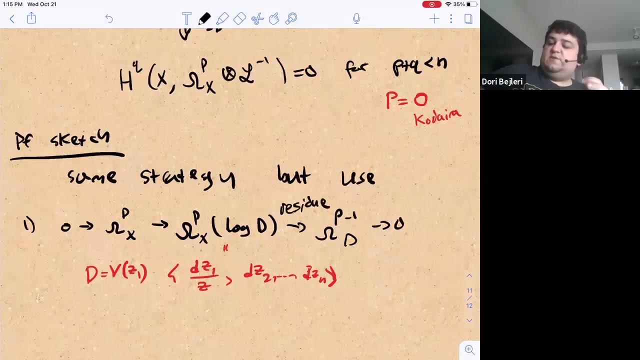 differentials that I briefly mentioned a few classes ago. So these are sheaves that, locally, are generated by things of the form DZ1 over Z and then DZ2 through DZN, where D is the vanishing of Z1.. And what is this map? This map is the residue map that takes some differential form. 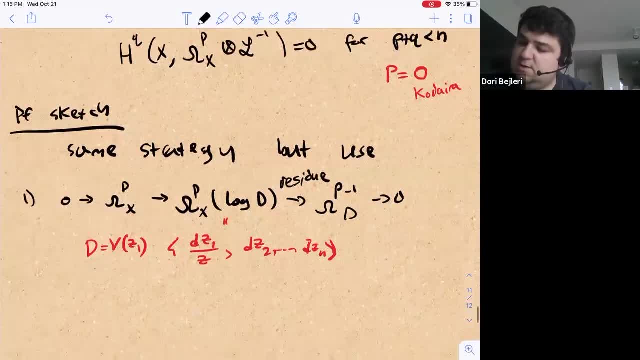 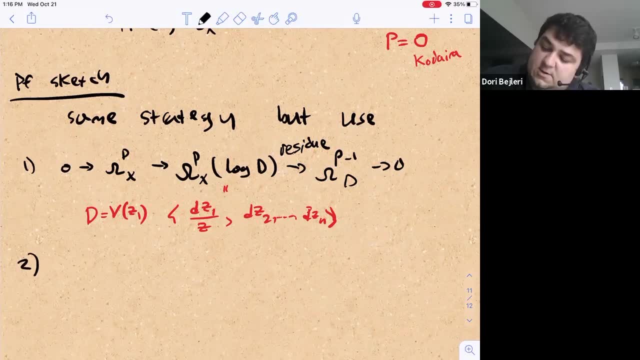 with poles to its residue, which is the usual complex analysis residue, And since it eats up one of the poles, that's why you get something P minus And then the second one. you need to have restrictions somehow So the restriction fits in. 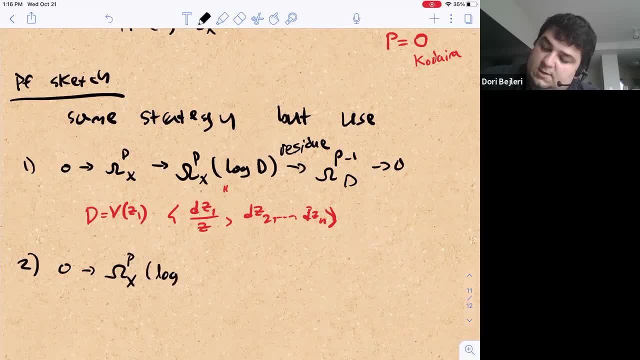 where, if you look at omega PX, log D twisted down by D, this sits inside of omega PX and this is the kernel of restriction to omega P, Like that. So the strategy is the first exact sequence plus induction on the first exact sequence plus induction on the first exact sequence plus induction. 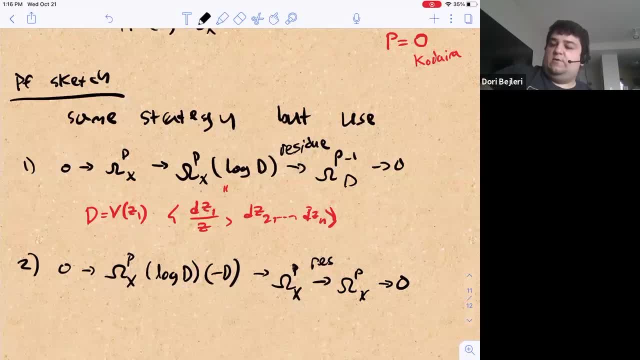 on the dimension reduces the statement to proving something about omega P log. And now this omega P log, when you twist down, becomes the kernel of restriction. So now the second exact sequence relates you back to the case of Lefschetz hyperplane theorem. 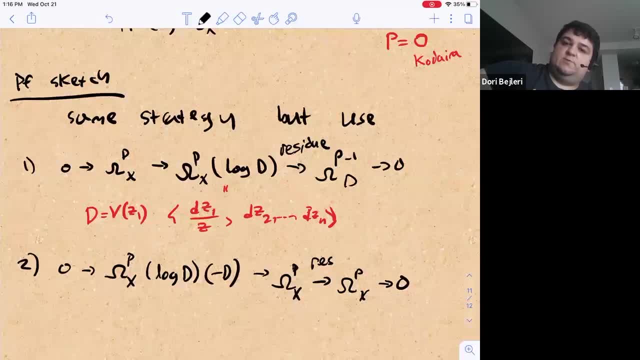 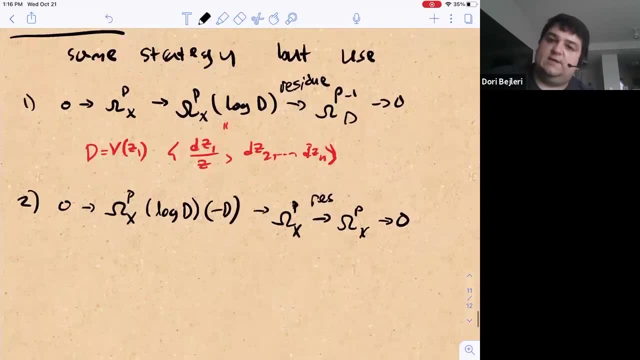 And so these two exact sequences, plus induction prove it in the case where your divisor is actually a smooth ample. And then you do the same exact cyclic cover. but now you need to understand how the logarithmic differentials change on cyclic cover. And so the second exact sequence: 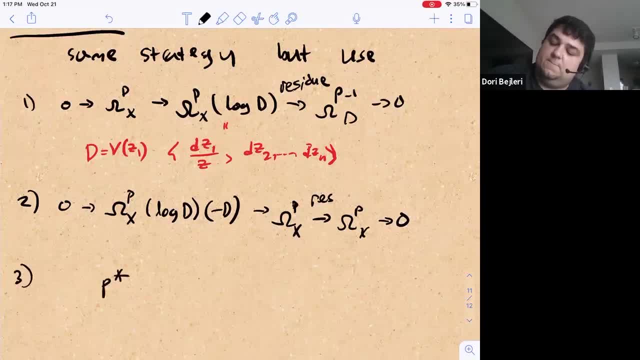 is a smooth, ample And now you do the same exact cyclic cover. but now you need to understand how the logarithmic differentials change on cyclic cover. And so the second exact sequence is that on the cyclic cover, P, upper star of logarithmic differentials, downstairs.